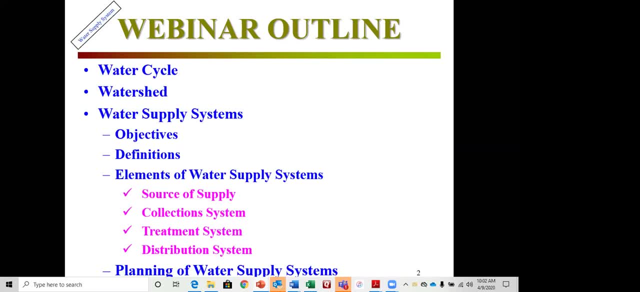 One is the source of supply, collection system, and the treatment system, distribution system. These are the four elements that we need. Then, finally, we'll see planning of water supply systems. So nothing can be done without any kind of plan or anything like that. 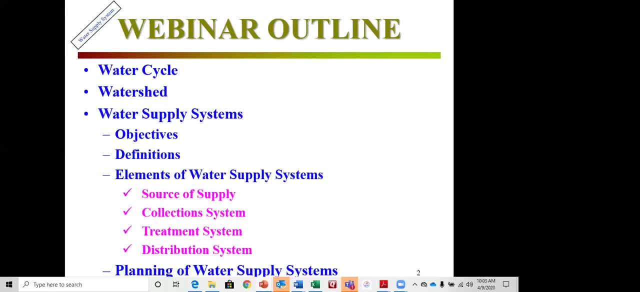 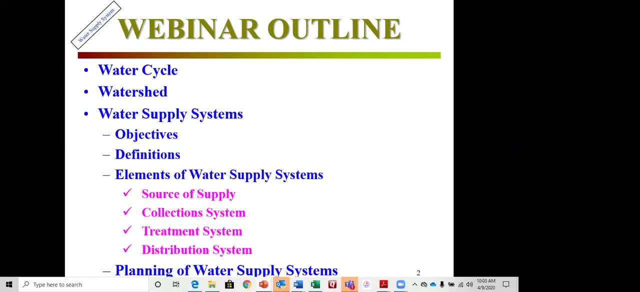 Then we are improved on, like water supply system. So one thing that I see here looks like I can see the participant's name, or sometimes, when I'm displaying my screen, I don't see the like, say, chat box or anything like that. 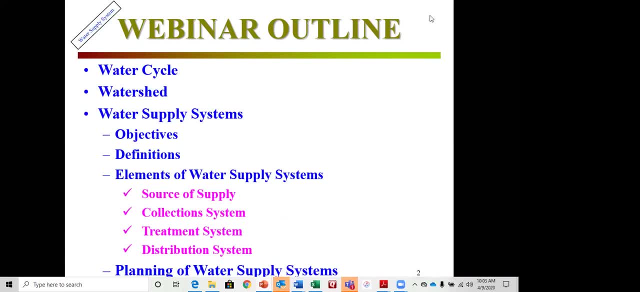 So I don't know whether I will see anybody asking any questions or not. I was wondering whether you guys can probably speak up. So if you can speak up, it would be good. If you can speak up, it would be great. I don't see the list of the people in there. 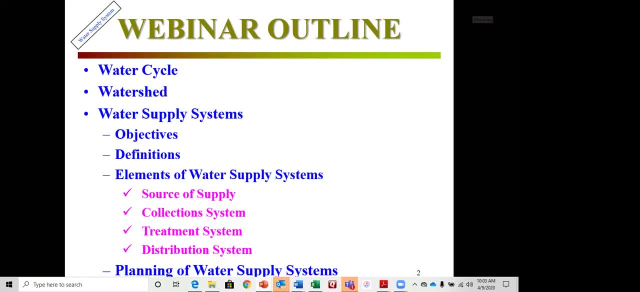 I have to, like say, click another screen. Oh, okay, they cannot talk. Okay, So then time to time I'll open the chat box and see how many questions I have, Because when I'm displaying my screen I cannot keep the chat box open. 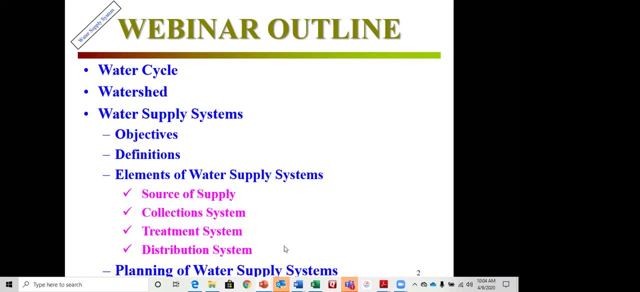 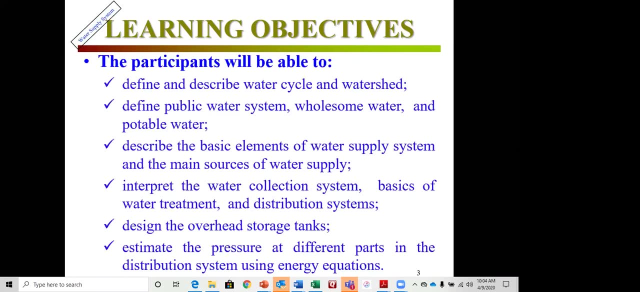 So in this case it goes away. So when I'm changing my slide and other things, Okay, Okay, Very good. The participants will be able to define and describe water cycle and watershed. So these are the two things they will be able to define. 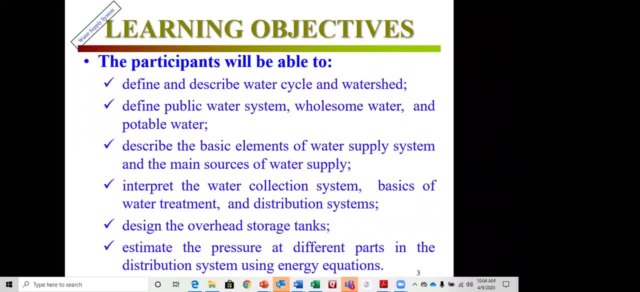 Then define public water system. What are the different types of public water system we use by definition And what are the importance of them? Wholesale water, wholesome water, potable water, palatable water- These are the one kind of different terminology that we use in these scenarios. 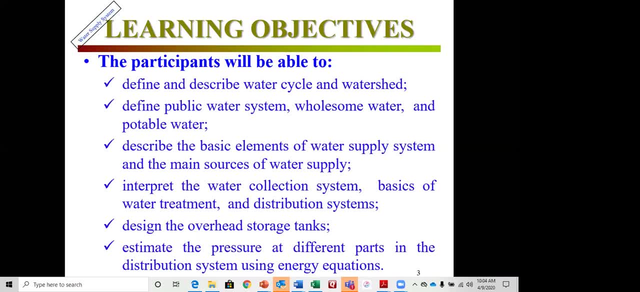 So describe the basic elements of water supply system And main sources of water supply Elements. you guys know the four elements right? So whenever I say describe, that means you have to say the name and just say a few words about those, right. 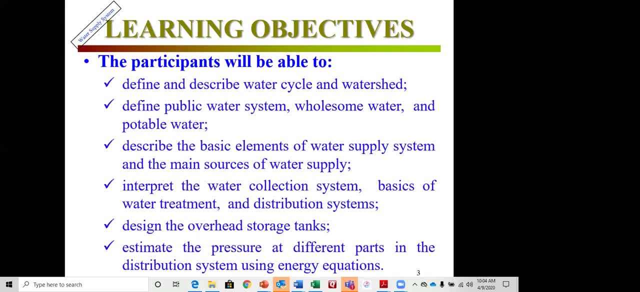 That's the meaning of it- And main sources of supply. we'll discuss at least two sources: surface water and groundwater, and maybe rainwater, a little bit tertiary or third source, but not a viable one. Then interpret the water collection system: basics of water treatment and distribution. 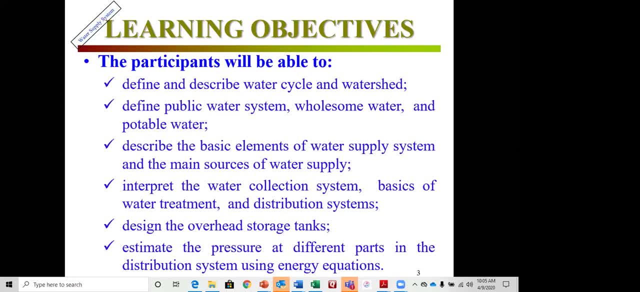 system. I'll go through a little bit of detail, not a whole detail, little bit of detail on those things. Okay, So you guys can take a look on those. Design the overhead storage tank: We'll see a little bit of theory of overhead storage tank, why we have overhead storage. 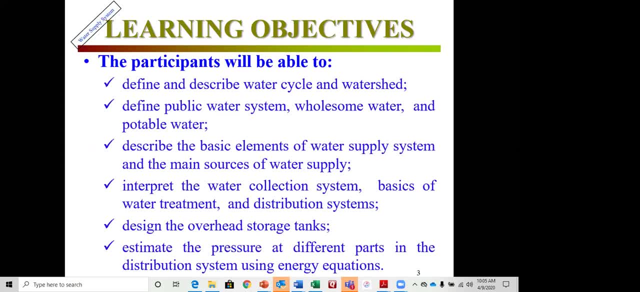 tank And from there we'll try to design a simple one for a certain amount of volume that we'd like to keep in there. Then, finally, we'll do the estimate of pressure at different parts in the distribution system using energy equations. So energy equation is a very important equation. 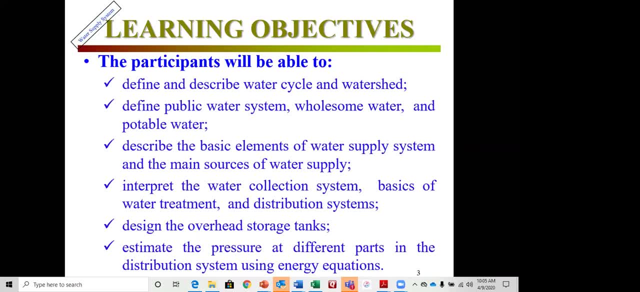 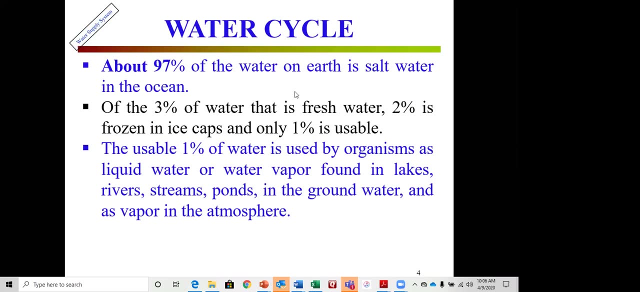 We know that right, So I'll show some example: how to use the energy equation to find the pressure in different places. Oh, I don't know that. I have the clap in here. Okay, So in the water cycle, in order to understand the water cycle, we know that about 97% of 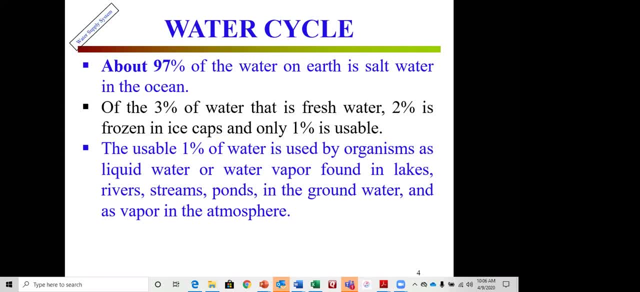 the water on the earth is salt water. Only 3% is fresh water. right Out of the 3% fresh water, 2% is frozen ice caps and only 1% is usable, that we are using recycling back and forth when we are using it. 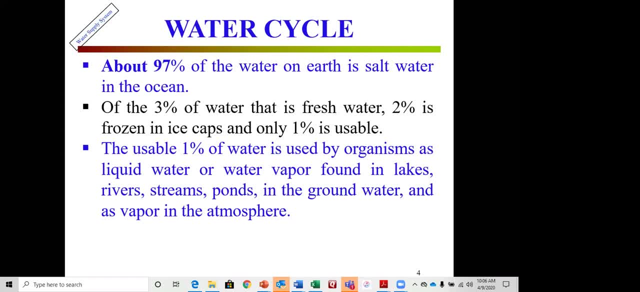 The usable 1% water is used by organisms as liquid water or water vapor found in lakes, river streams, ponds in the groundwater and as vapor in the atmosphere. right So water form and the vapor form, whatever the form we have. 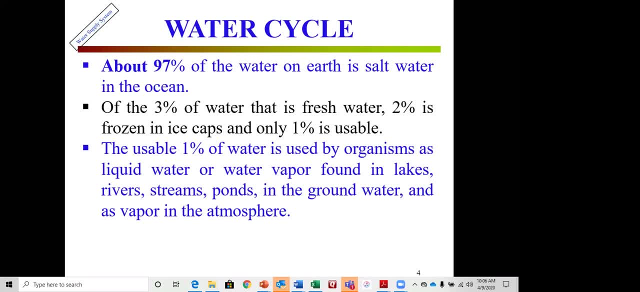 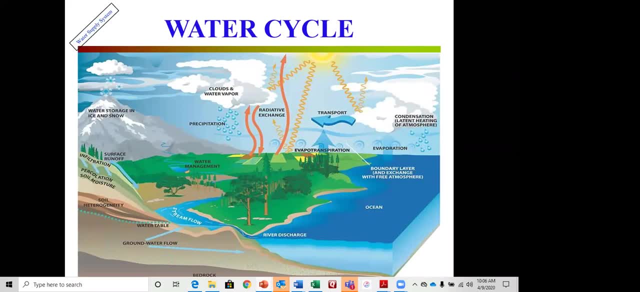 Only 1% of the water in the atmosphere, Only 1% of the water in the whole world. Sorry man, I don't know. I have this somehow set it up over there. So this is the water cycle. basically it shows the different parts of the water cycle. meaning: 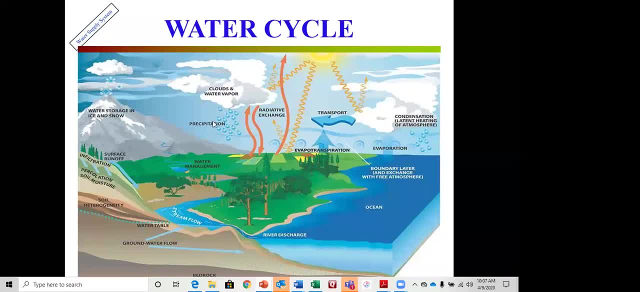 the water coming to the earth as rainwater and precipitation and other things, and it's radiating. It's radiating back to the atmosphere and so on, And when it's coming to the upstream, it's going to the downstream, like so then even. 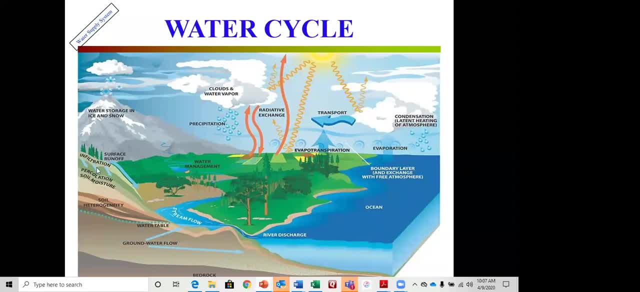 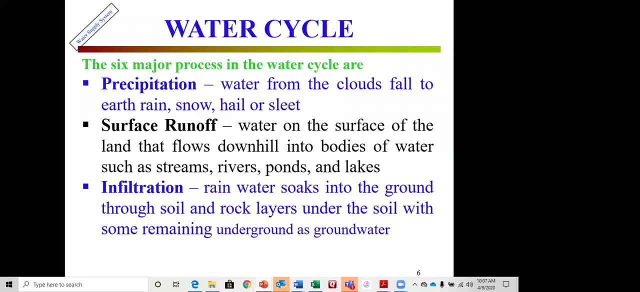 if it's coming out from the groundwater in different ways- evapotranspiration and other things like that. So this is basically a basic view of water cycle. So, sorry guys, let me see whether I can take those things off, Okay. 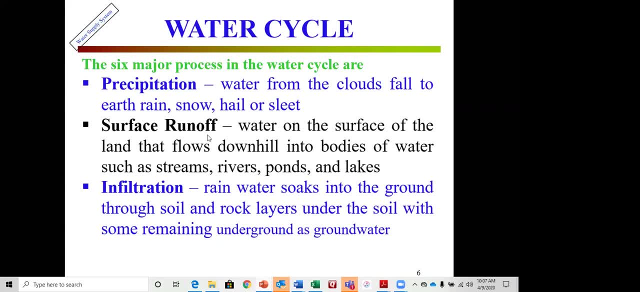 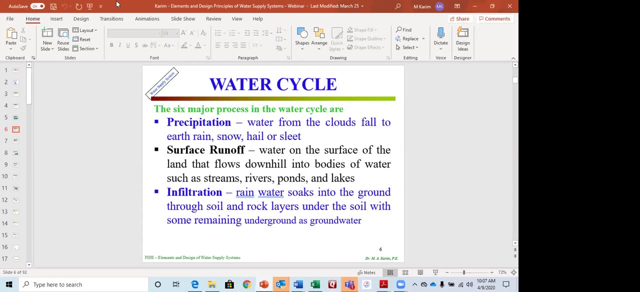 Okay. So this is the water cycle and these are precipitation, surface runoff, filtration, evapotranspiration and condensation. Sorry guys, I need to go and probably just change this. a little bit of animation. Okay, Okay, Okay. 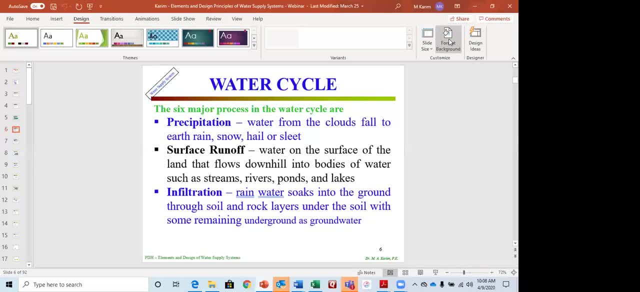 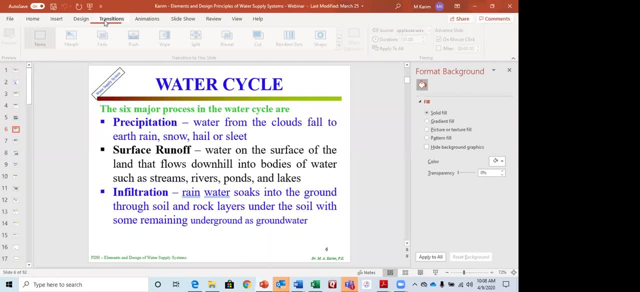 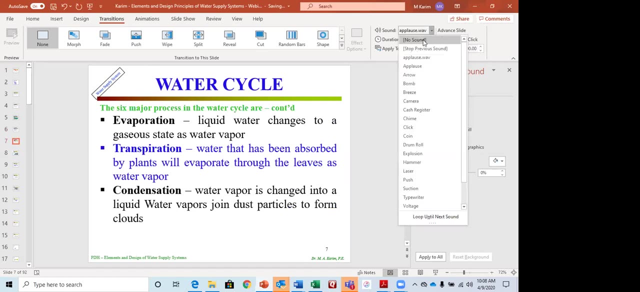 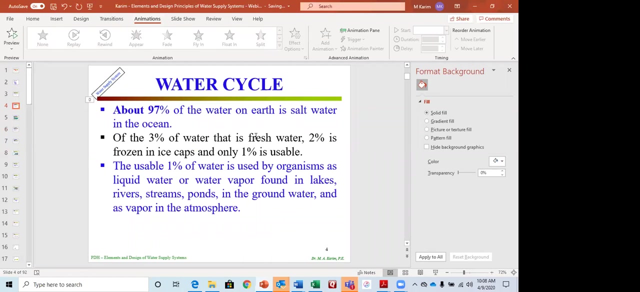 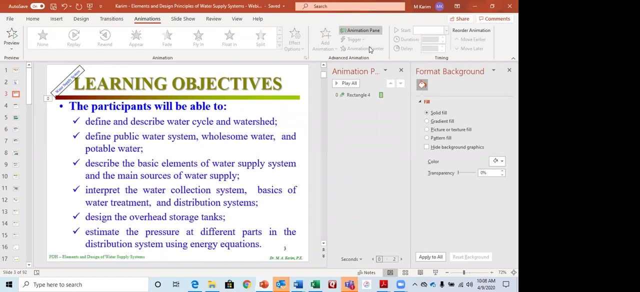 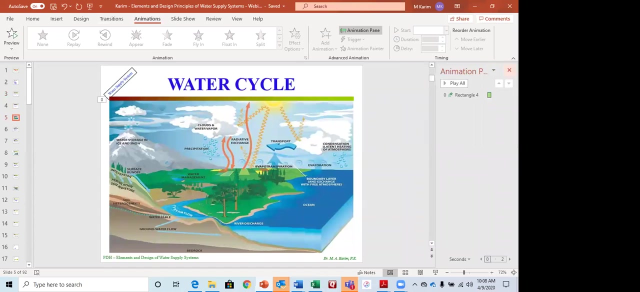 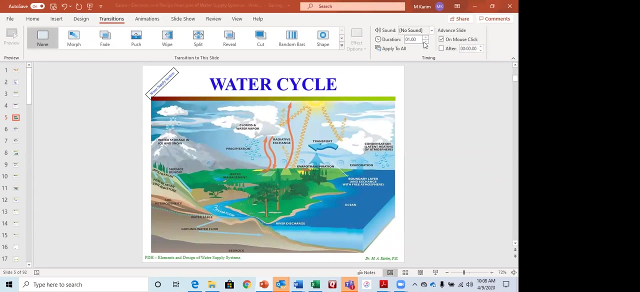 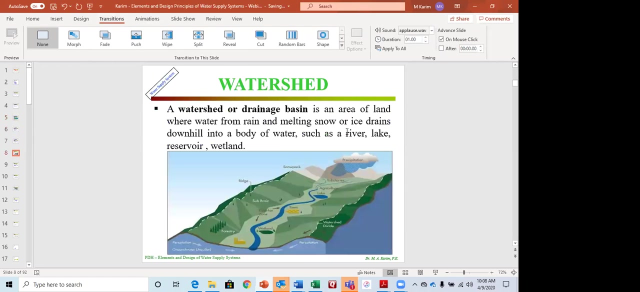 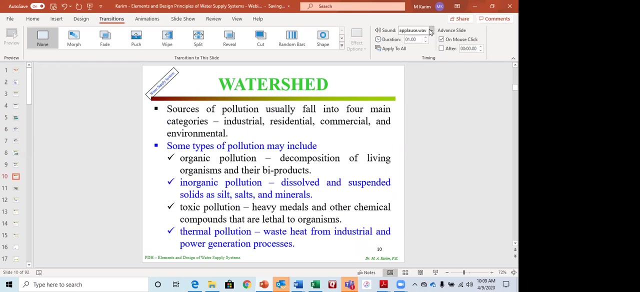 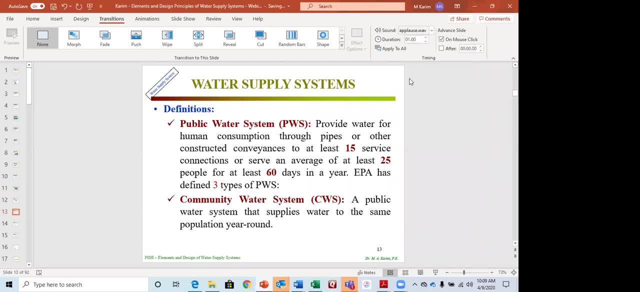 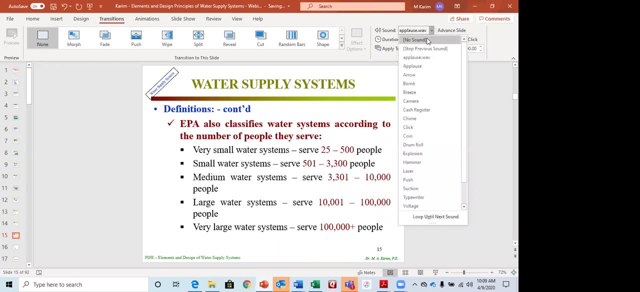 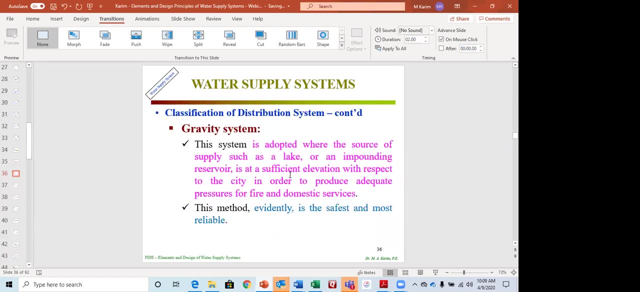 because it will give us kind of hard time. I don't know that I can take everything off from one slide because I copied from slide to slide, So that's why it went in there. Hopefully there'll be no more sound. Okay, okay, very good. 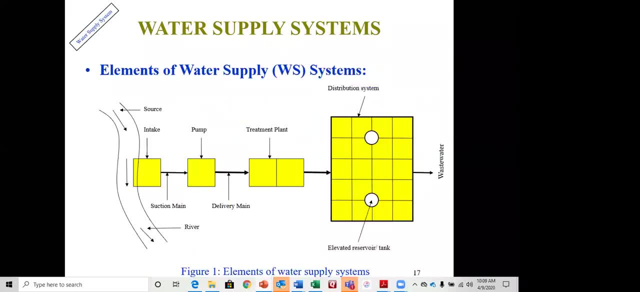 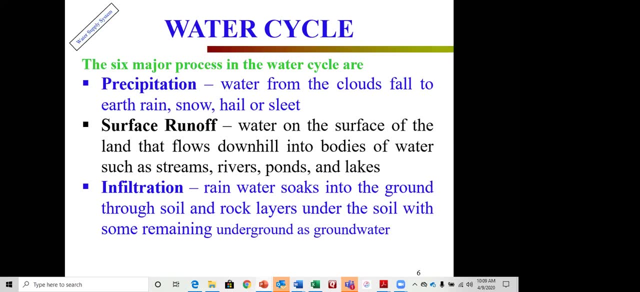 Okay, we were here. Sorry about that. I do apologize again. The six major processes in the water cycle. these are: number one is precipitation. We mentioned that: the water that from the clouds fall to the rain as a snow hill and slay. 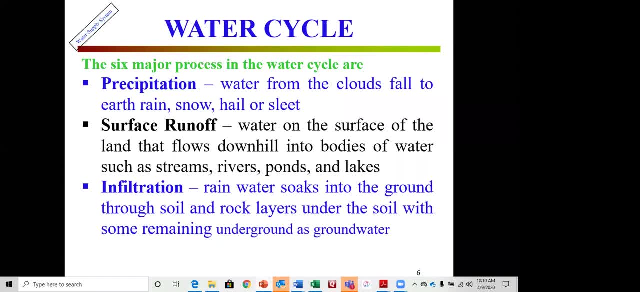 things like the surface runoff the excess water when the rainfall like falls into the ground surface, then part of it infiltrate to the groundwater and remaining flows to the surface. water goes to the river and other things Infiltration. the rainwater soaks into. 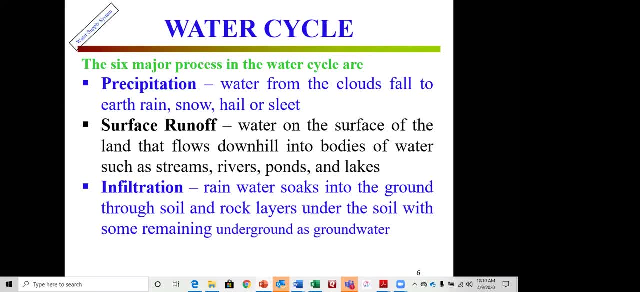 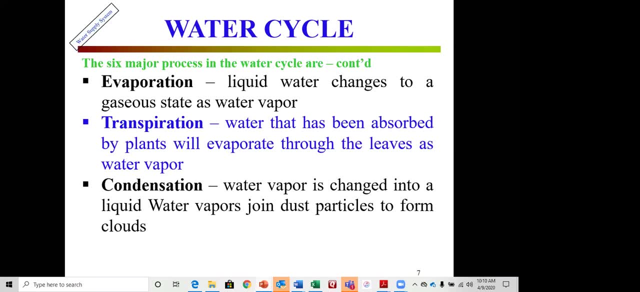 the ground. once they fall into the, the rainfall falls into the ground surface. Okay, then the evaporation: liquid waste changes to gaseous state as a water vapor and goes into atmosphere. Then transpiration, or evapotranspiration: water that has been absorbed by plants will evaporate through the leaves as 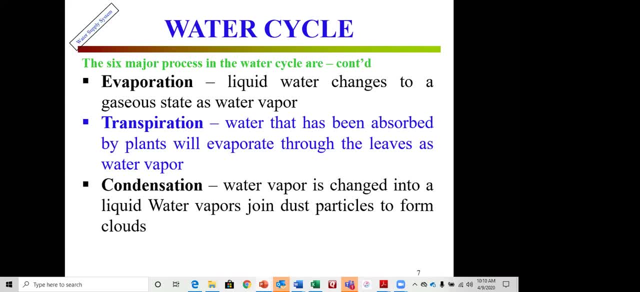 water vapor. So this is called transpiration or evapotranspiration. Condensation: water vapor is changed into a liquid water vapor to join dust particles, to form the clouds and other things like that. So these are the six major processes that a water cycle has. Okay, the watershed, a watershed or we. 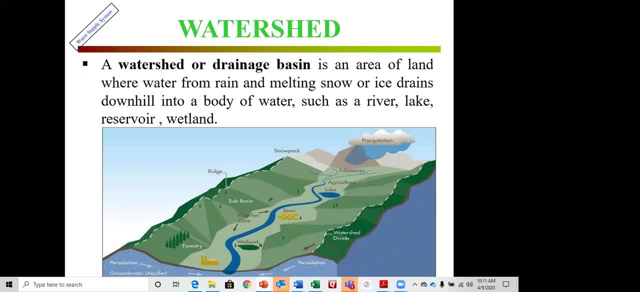 can call is a drainage basin is an area where the water come from, like, say, water when the rainfall falls around the area, come to a certain place, or discharge to a certain point. Okay, so then this could be in a body of water, it could be a river, or it could be lake, it could be reservoir, it could be wetland. So this is the catchment basin, or drainage basin, or 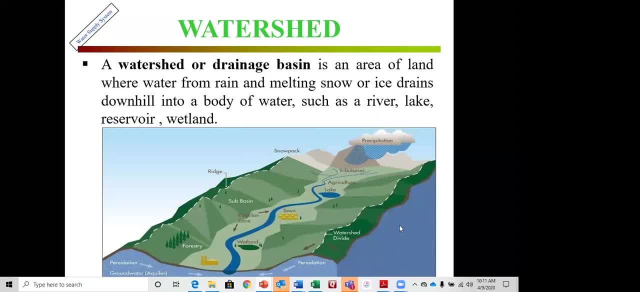 watershed and these are the lines it's called the divides. Divides means the waterfall. If the rainfall falls over here, then it will go to the other way, not just coming that way. So that's the meaning of the watershed. So we have to. 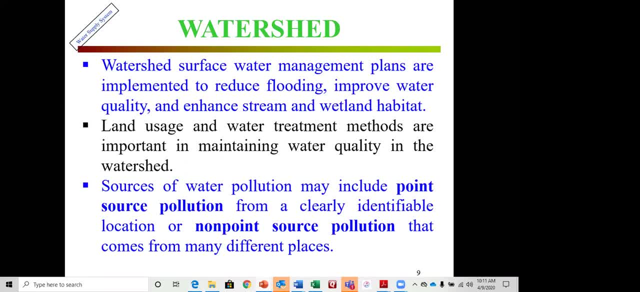 understand the watershed, the one reason to understand it because of looks like if we are selecting a source, then definitely we have to know whether the watershed water or the area the water will be getting into this river, or the source, whether it would be good quality or not. if we know there are a lot of. 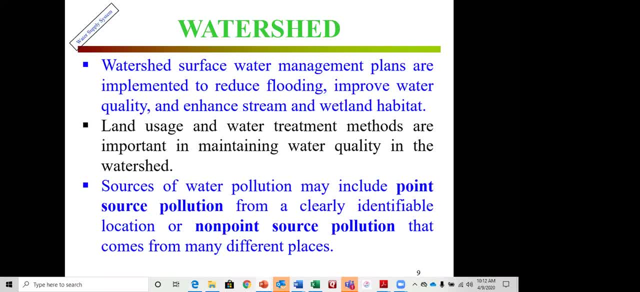 contaminants may be coming from different sources for this watershed, then it may not be good idea or you may have to think different way, maybe go for groundwater and other things. so land uses, water treatment methods are the important, maintaining water quality in the watershed. then the sources, as I 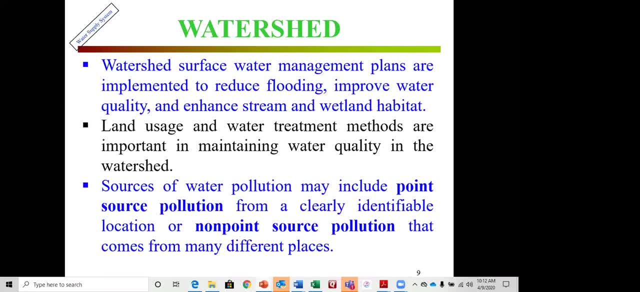 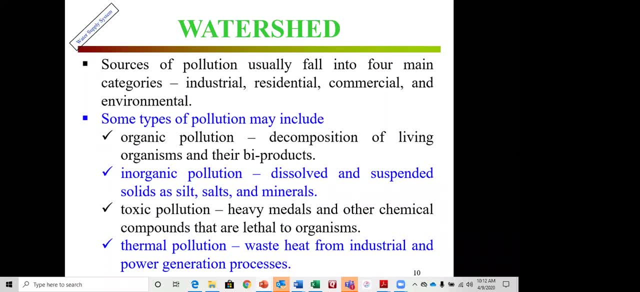 mentioned that: the point source and the non-point pollution source. these are very important to understand. so, okay, sources of pollution usually fall into four main categories that could be in a watershed could be polluted too, so industrial, residential, commercial and environmental. so some types of pollution may include organic pollution. we know that organic. 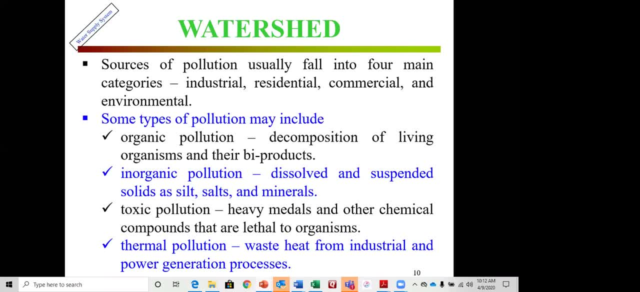 pollution is could be BOD, COD or some other biologically facts in their decomposition of living organism and their by-products. inorganic pollution: dissolved and suspended solids as sealed salts and minerals. toxic pollution: heavy metals should be metal and other commercial other commercial compound that are lethal to organism. So this would be tea. Let's see whether I can get a good color. 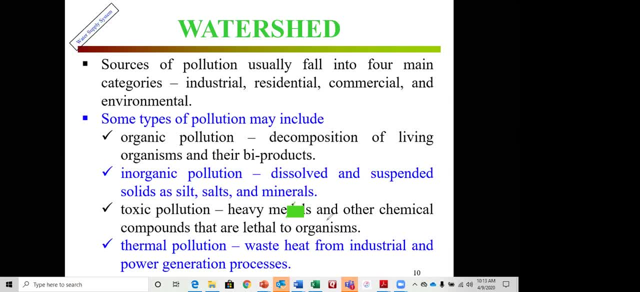 Okay, and then thermal pollution, waste heat from industrial and power generation processes, So this could be other types of pollution from there. I don't know. this system is very hard for me to understand. Okay, why I can't change the slide. what did I do? 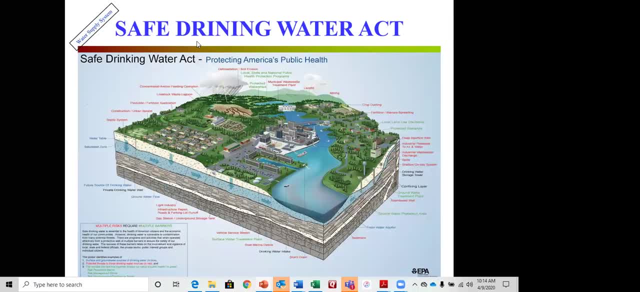 Okay, so something didn't work over there. Probably I fixed it. This is the one kind of like say, safe drinking water act shows. like, say, what are the different things we have to do to make sure that we meet the requirement of Safe Drinking Water Act, Meaning, like I said, the area that we are going, the water. 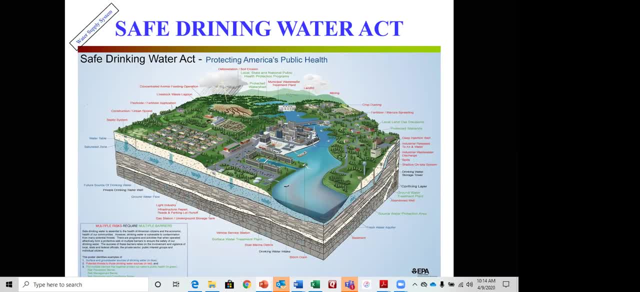 from that means the source. it has to be selected properly to meet the requirement of Safe Drinking Water Act. right, It's not really saying that that you have to have water from here and there, but the way we manage those things, ultimately it will help. 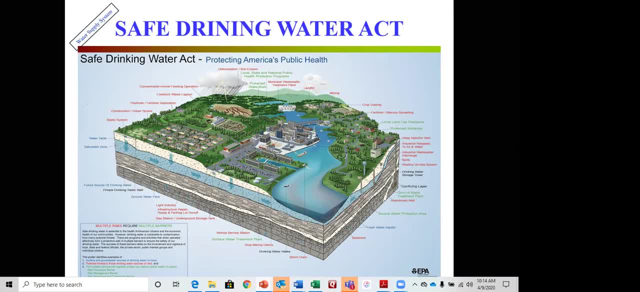 us to meet the requirement of Safe Drinking Water Act. So it's mainly to protect the America's public health and so on. This is basically showing a kind of ideal city, but all of us, this is not the case. Okay, So, all of us, this is not the case, but this can give us. 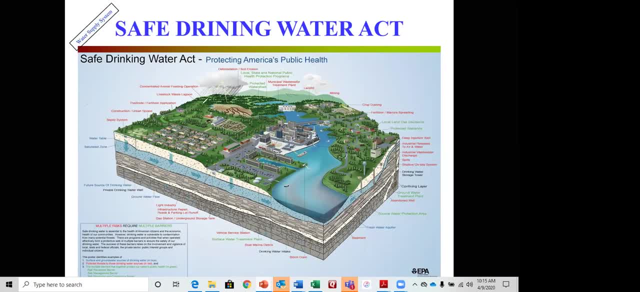 a little bit of idea how ideally it should look like. in real life you can make something happen like that. So these are the storage tank looks like. These are the different houses. These are the river that's going through this. The sources would be very good in here. 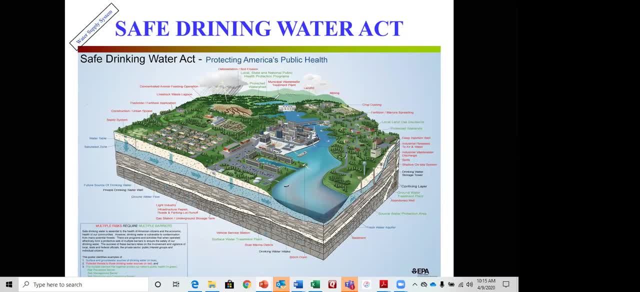 We have a dam over here, right Reservoir. maybe They're storing some water over there Here and there, So this shows a little bit of how beautiful it looks like. if you can make something real, ideal like that, So that will help us to meet the same drinking water. 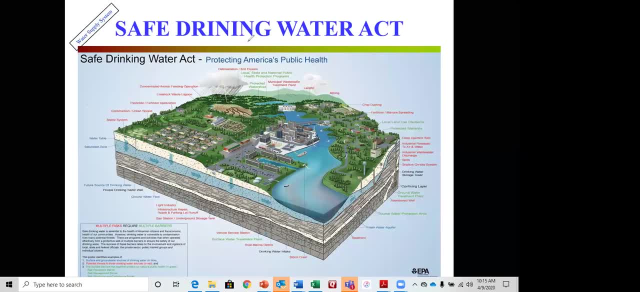 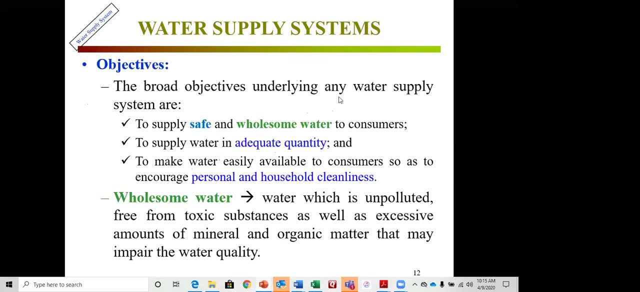 act. Okay, Okay. The broad objectives underlying for the water supply system are to supply safe and wholesome water to consumers, to supply water in adequate quantity And like, say then, personal and household cleanliness. Here is the definition of water: wholesome water, Water which is unpolluted, free from toxic substances as well as excessive amounts. 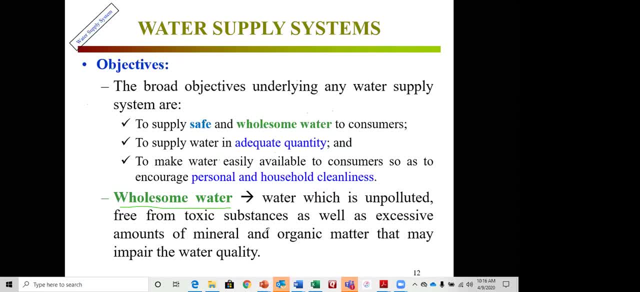 of mineral and organic matter that they may impair the water quality. So that's the wholesome water And the other two definition. I'm not sure that I have those in here, But one thing that I know that we will have here is that we will have a lot of water. So I don't have it, But anyway, I can define those. 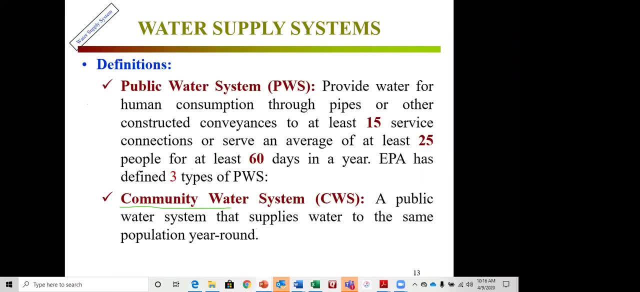 The portable water means the water that is safe to drink. That means we don't have any contaminants or anything like microorganisms or pathogens. Mainly we can define it as a pathogen. Okay, And palatable means it's pleasant to drink. I mean it's clear It. 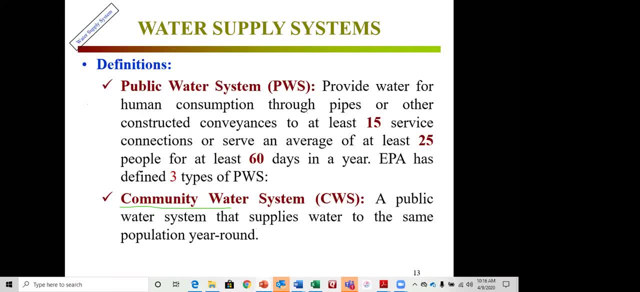 shows good, like clear view of this thing. There is no suspended materials or anything like that. It's not showing any color, So these are kind of palatable water. Anyway, here are some of the definition of the water supply system that we use in this case. Okay, So the number one is the public water. 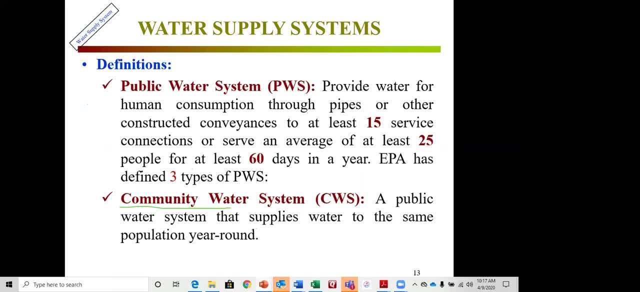 supply system. PWES Provide water for human consumption through pipes or other constructed conveyances to at least 15 services connection or service at least 25 people, at least for 60 days in a year. Okay, This is called public water supply system, So there are three different types of public. 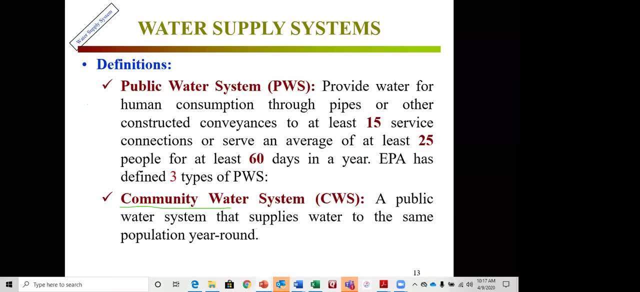 water supply system. The one is called community water supply system. The community water supply system means it supply water to the same people all year round, Mean like a permanent city or like, say, permanent subdivisions of the houses. So these are the one community water. 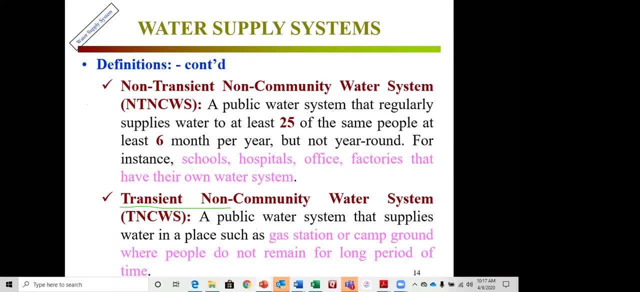 supply system. So non-transient, non-community water system. basically is a public water system That supply at least for 25 of the same people, at least six months per year, but not year around- For instance, schools, hospitals, offices, factories, and that they have their 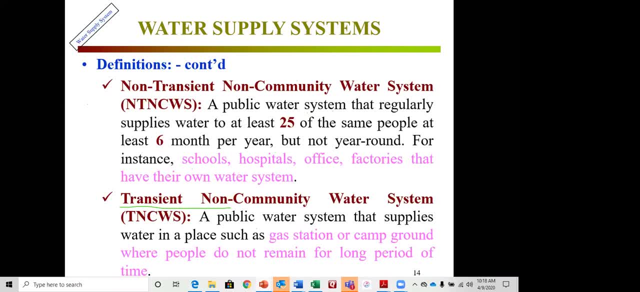 own water system. Transient non-community water system is basically public water system that supplies water in a place such as gas station, campground and other things where people do not remain for long period of time, So this is called community water supply system. 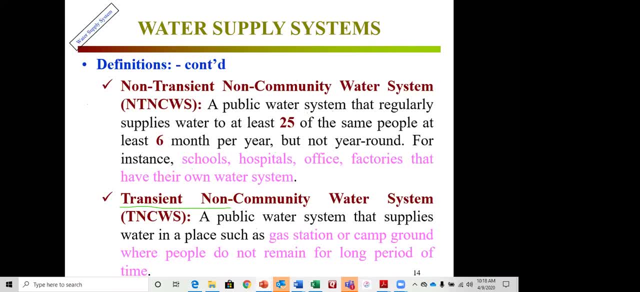 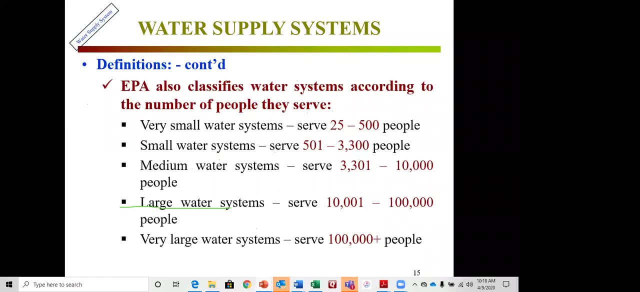 Okay, So this is called community water supply system. So this is called community water supply system. So this is called community water supply system. So this is called community non-transient community water system. So these are all public water supply system. So EPA also classifies water system according to the number of people they serve. Okay. 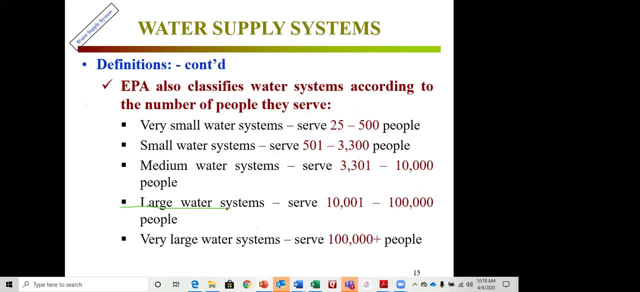 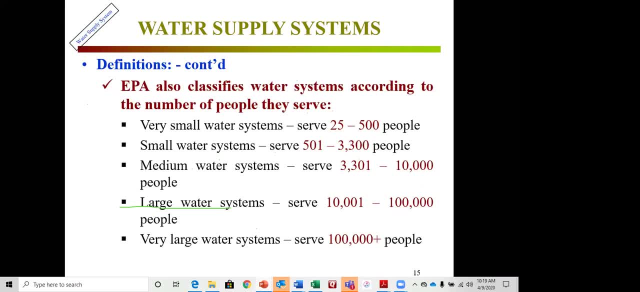 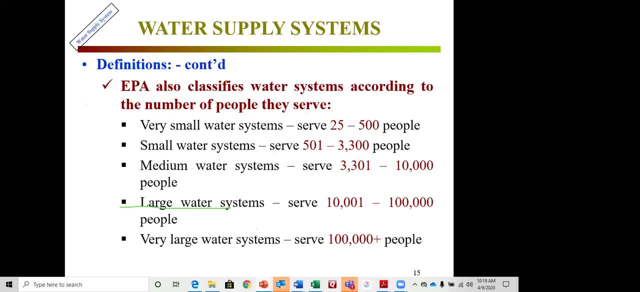 report the data for maybe once a month, whereas the other one may say report the data to every every week. so main purpose of those things like that, why more stringent? for the very large one, meaning if something goes wrong over here, hundred thousand people would be affected. and it took very hard to. 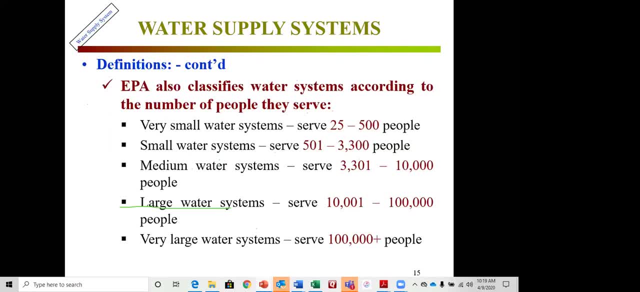 supply water with some other arrangement. two hundred thousand people if we need to shut down the the water supply system, but it's the smaller one. if it is up to 500 people, yeah, if we can find it out, we can stop it and probably we can provide. 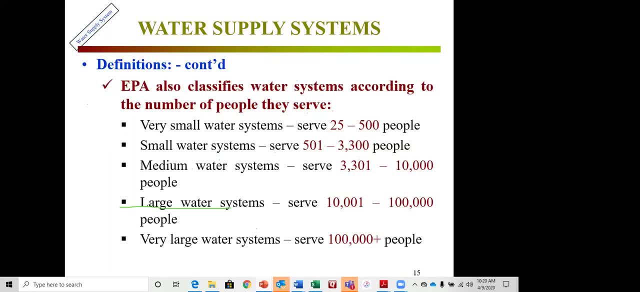 supply the water for 500 people very easily, right? so that's why probably more less stringent over there is make sense to some extent. not in terms of the regulation, and I'm saying it could be in terms of what is called the reporting requirement, another requirement. there are some other differences too, but these 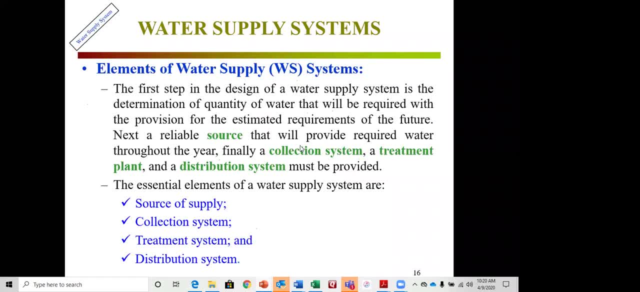 are the basic ones. okay, then we'll go to elements of water supply system. the first step in the design of the water supply system is the determination of a quantity of water that will be requiring during the time. whatever you need, that next reliable source definitely. then before another source, we have to collect it then once. 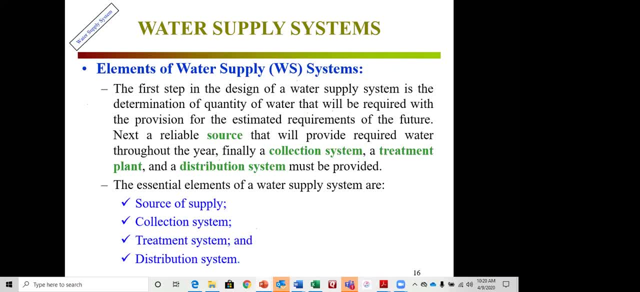 we collect it, we have to do proper treatment to make it palatable and portable, palatable and safe or wholesome, whatever you can call it. then we have to have a distribution system to supply water to the individual houses. so these are the four essential elements: source of supply, collection system, treatment system and the distribution. 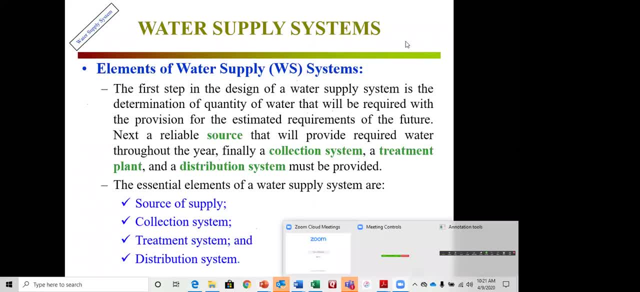 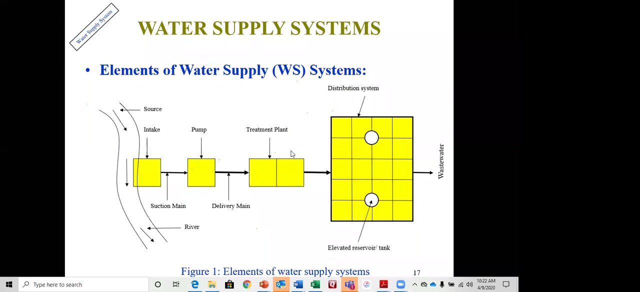 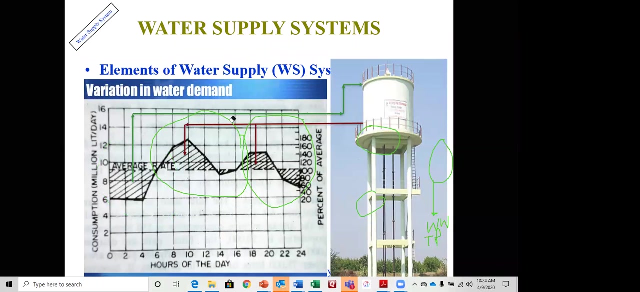 system. okay, let's see whether I can see what is called the okay. okay, looks like I'm checking the chat box. since you guys, can I talk, so do we have any questions? so far you can type the question in there. you are open, okay? okay or not okay? so let's see what that is. so what's that? 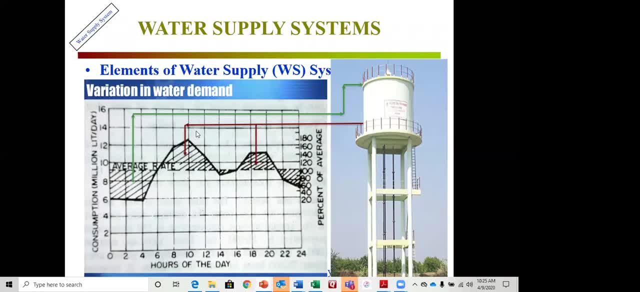 right now is going down and, okay, we are providing that much so, and this is our average providing and this. our demand is this. so this is amount of water they have excess, in this case, whenever we are pumping, so we can put this water into the tank. so whenever we. 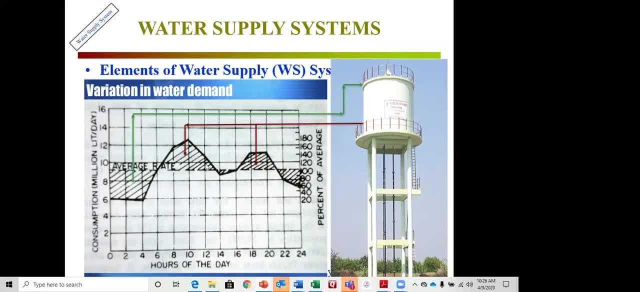 need this water. so right here, in this area, this is our supply line we are providing. this is our shortage, then we can bring this water from here to the shortage. similar things over here. we are not bringing anything here is, it looks like little, but we can also put this water in there then from here is. 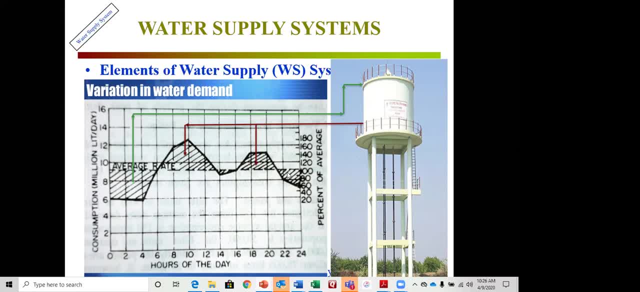 definitely. whatever we do, we will bring the water over here and from here again you put the back to that tank. so that's the way it's like. it does two things. one is basically it helps us to pump the water in the same rate, and the second 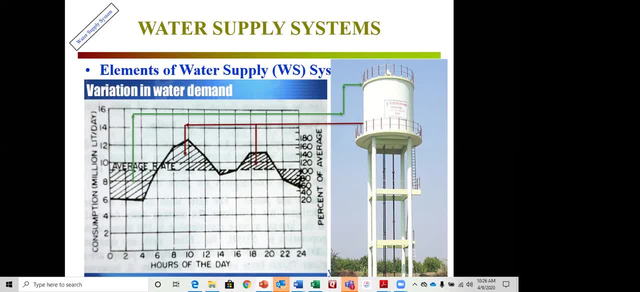 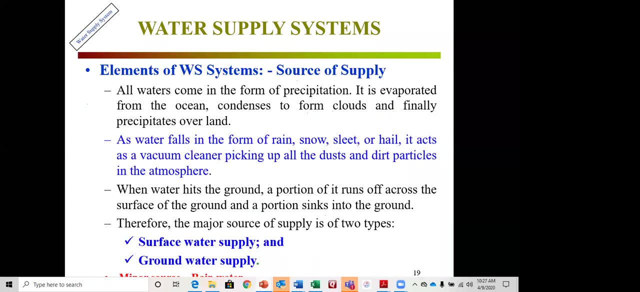 one. it also is easy of the operation and it increases the life of a pumping system because we are not doing the varying level, speed of the pumping system and so on. so that's the another important part of it why we do that way. the supply of water: okay, so all water comes from a precipitation in the 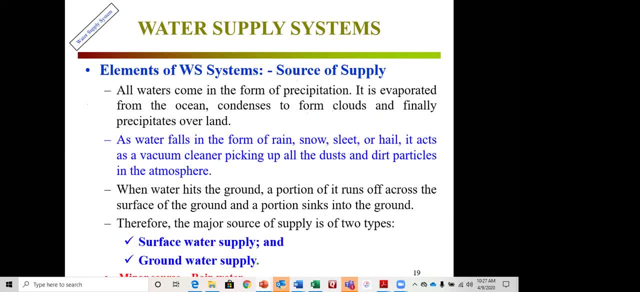 form of precipitation. we have seen that in the water cycle it is evaporated from the ocean, condensed to the form clouds. and finally, precision, we know that the water falls into the form of rain. okay, we already discussed that. when water hits the ground, a portion of its up- access the surface water, a portion sink. 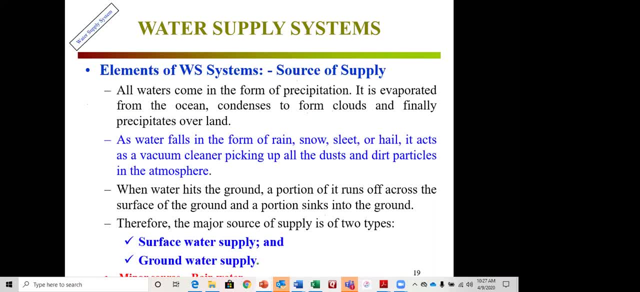 into the ground. this is the, the infiltration. so therefore the major sources of water supply is two types: surface water supply and the other one is a groundwater supply. there is a minor one. I don't know that you guys can see it in in my screen looks like it's minor source of the rain water. so the minor. 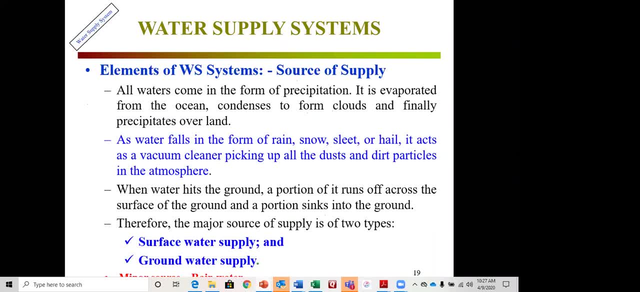 source is the main water that I mentioned because it's very important to understand that certain areas we may have a lot of rainfall. two hundred point fifty three hundred inches per year. it's a water right, a lot of rainfall. certain cases- this state that i live in. i know that per year average. 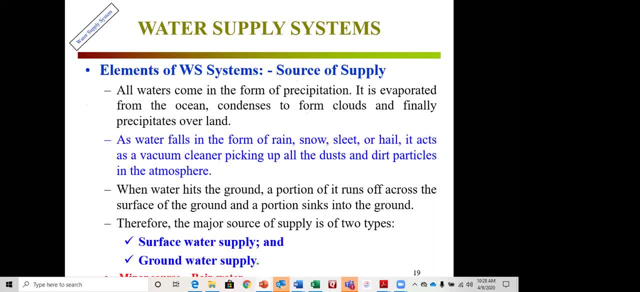 rainfall is 50 or 50 inches per year, but in this case it's not enough, right? so 50 to 60 or something. i don't think this is enough. so in this case, uh like say, it's not good source to select, or maybe anything like that. but if you have a 300 inches per year, then definitely it could be good. 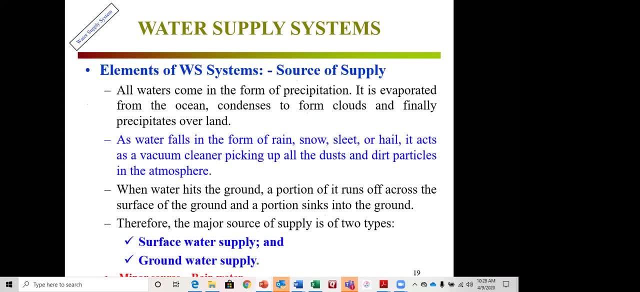 source to do that? yeah, you can do, or use a lot of rooftop to collect the water and with small uh treatment or a very simple treatment, uh, probably you can use the water watering the lawn, wash the car, watering the grasses and, and maybe some cases, using in the toilet. maybe. 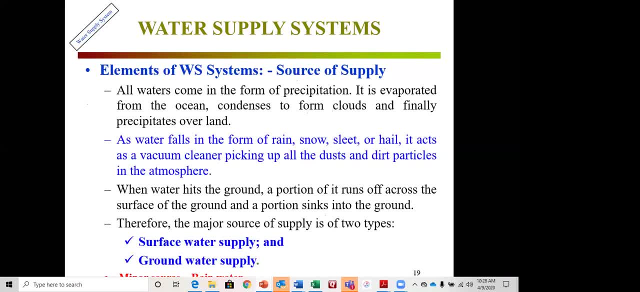 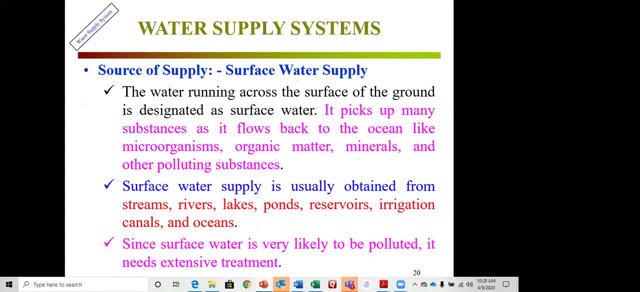 toilet flushing so you don't need to use the the supply water for toilet flushing. so, yeah, these are the things we can do if the county city allows us to do. certain cases have to get a permission to do that way also. okay, the water running across the surface of 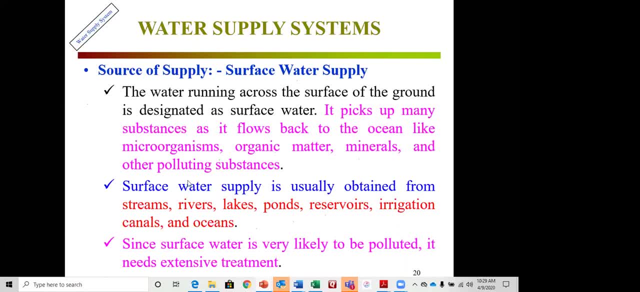 the ground is designed surface water. so the surface water here, the surface water uh mainly thing, uh coming from streams, rivers, lakes, ponds, reservoir irrigation canals and oceans. since surface water is is very likely to be polluted, it needs extensive treatment. why it is very likely to be polluted? because of uh it, it comes with a rainfall, the rainfall. 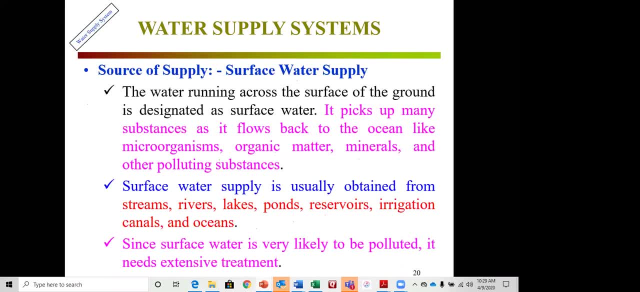 is a lot of materials from the uh our surfaces, right from the ground surfaces or anything like that, or it wash out different uh areas- uh pollution, like non-point sources from agricultural areas. it could be agriculture area, it could be parking lot that can get a lot of hydrocarbon and anything. 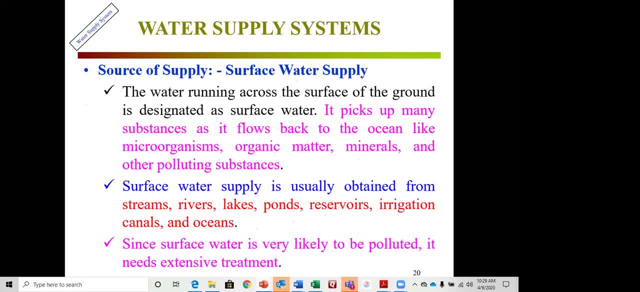 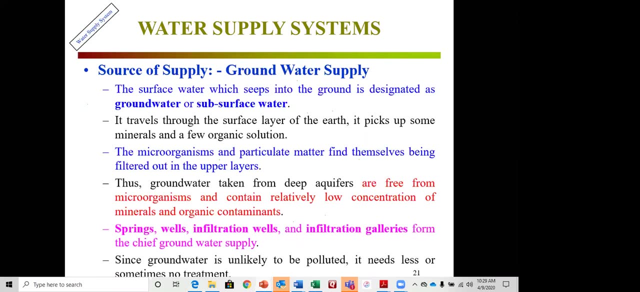 like that, so a lot of uh contamination might happen. so that's why surface water needs more intensive treatment compared to the, the groundwater, because groundwater may not have already it's the screen out, but through the soil anyway, okay, the surface water, uh, which sips into the ground, or is called 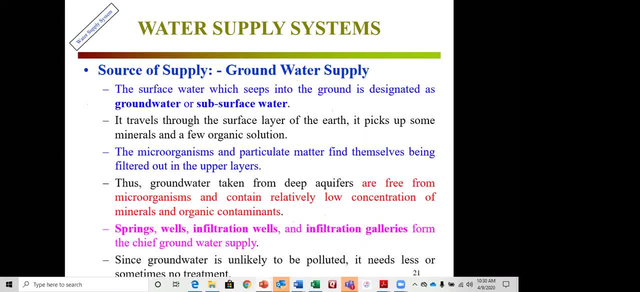 sorry, into the ground, is called the groundwater of subsurface water. it travels to the surface layer of the earth. it picks up some minerals and a few organic pollution. the microorganism and particulate matter find themselves being filtered out of the upper layers. yeah, some cases it happens there's groundwater taken from the deep aquifers or free from microorganism. 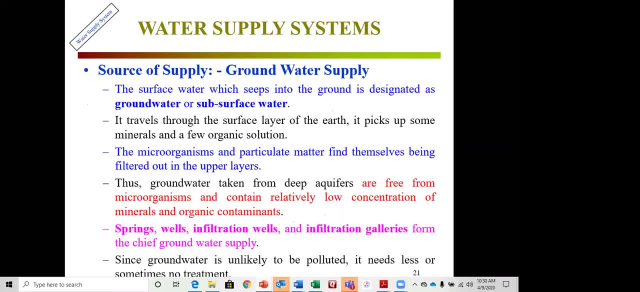 and continually low concentration of minerals and organic content means. so springs, wells, infiltration wells, infiltration galleries form the cheap- uh cheap- groundwater supply. since groundwater is unlikely to be polluted, it needs less, or sometimes no treatment before we can drink it. some of the rural areas, you guys have seen that they don't. 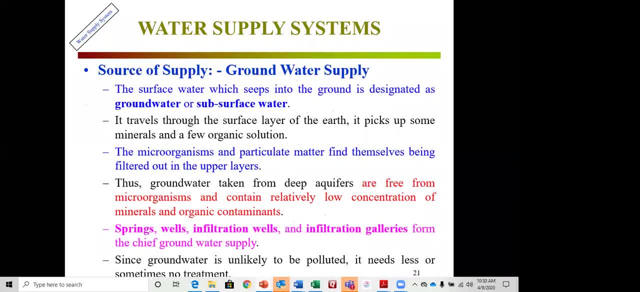 do any treatment. they're just consuming for everything. only places that i have seen they do some kind of treatment when it has a lot of hardness in there, so a lot of hardness water, like if you're taking shower, probably you're not getting any foam or leather in your 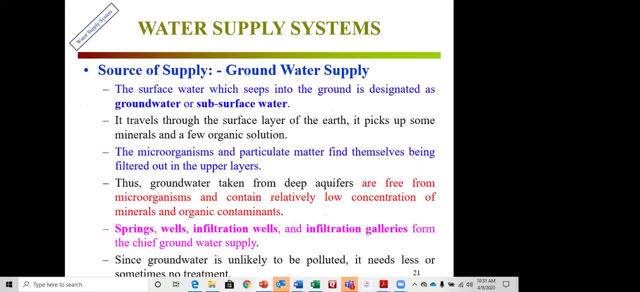 soap with your soap, because of the groundwater has a lot of hardness in there. so that's why, uh, hard water, we have to make it uh like soft water. i mean we have to remove the hardness before we can use it. so this is the only treatment that i have seen. some of the rural areas, uh, they have. 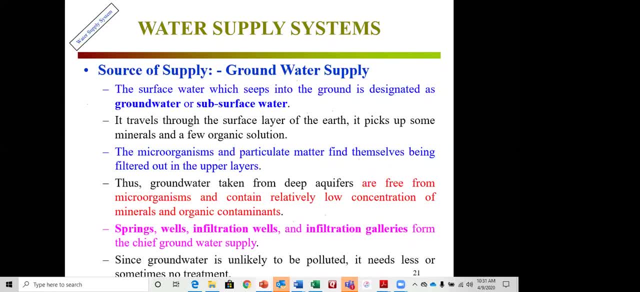 a tube to bring the water for out their drinking or other usage purpose to do the treatment- mainly the uh, hardness of the water and such. and then the hard water- 그럼 như这样来我们用这种水 first and then we remove the hardness before we can use it. so this is the only treatment that i have seen. some of the rural areas, uh, they have a tube to bring the water for their drinking or other usage purposes to do the treatment- mainly the hardness of the water and so on. so i guess 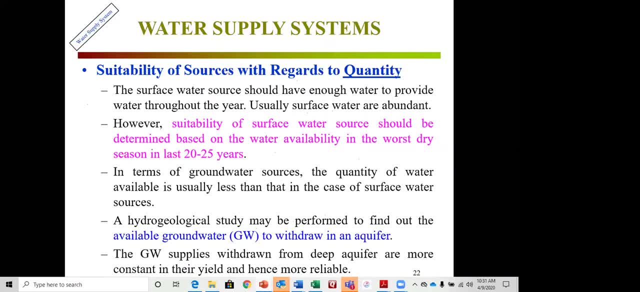 okay, then the next topic comes: once you know the source, how much quantity we need. so quantity usually the way we design any any water supply system, usually 20-25 years. so I mentioned here 20-25 years, but some of the cases that I do the design project and other things, we do something. 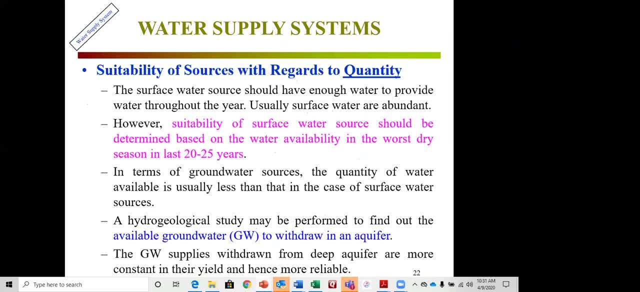 40 years, because 25 years is not that much. 40-50 is better, because nowadays there is another option. I think you guys do that too. so staging period: right, you can do the staging period. you can do the design for 50 years, but you don't need to probably construct everything in the beginning. 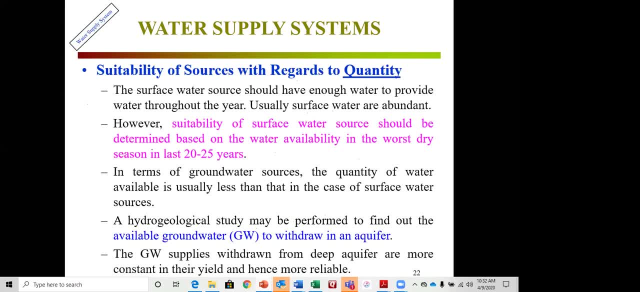 to reduce the like, say, infrastructure cost, initial involvement of infrastructure cost. so you can do every 10 years or every 15 years. so there is a calculation you can do how we can do like basically staging period. either it is 15 years or 10 years. 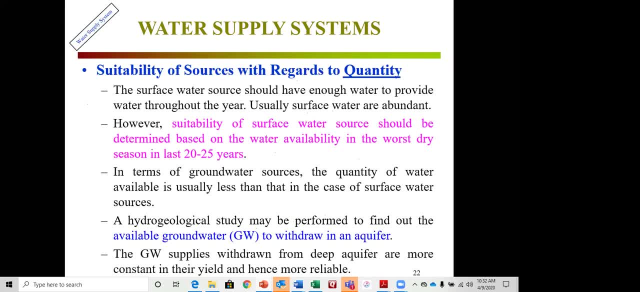 so this will give us an idea how we can do that. so in terms of the groundwater source, the quantity of water available is usually less than in case of the surface water source. it's always not the true, but it is true some cases because of the aquifer. if you have a deep aquifer, then it would be very 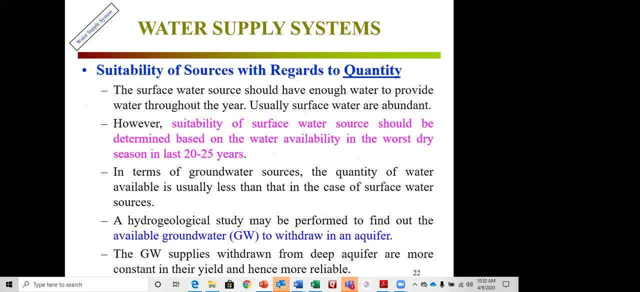 hard to extract the water through the pumping system, drilling wells and and things like that. so in this case, for a groundwater hydrologic study may be performed to find out the available groundwater to withdraw in an aquifer. uhh way, that would be part of thatी. 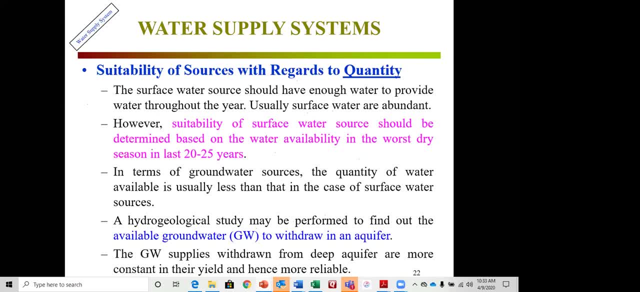 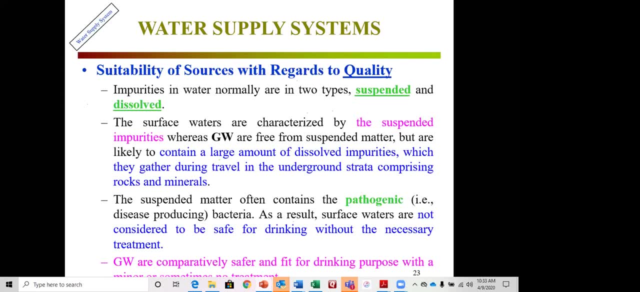 that is well, I see, alright, good bye, bye, bye, bye, byebye, bye, bye, bye, bye. quantity, then the other terms that come is the quality, so we know quantity. if we have a quantity, do you have the quality of the water? with that we need some cases, very important because of if the quality is not good, then what is going? 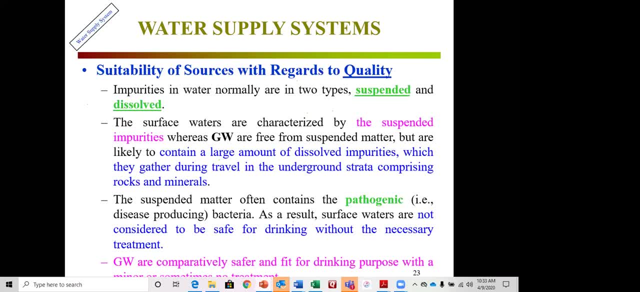 to happen probably if we use this source tail, then we have to have a lot of treatment, and treatment cost money and if it costs money to treat the water, the ultimately it will be passed on to the consumers. so the consumers will not be happy. that means the business may not be a good way. so these are all part of 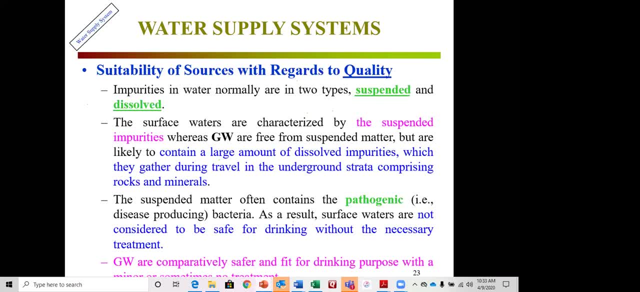 the consideration of the system design and other things like that. so impurities in the water there comes in two forms. one is called suspended, other one is dissolved. suspended: the material that can be probably separated by physical process. physical process: one of them could be sedimentation. they're settling. 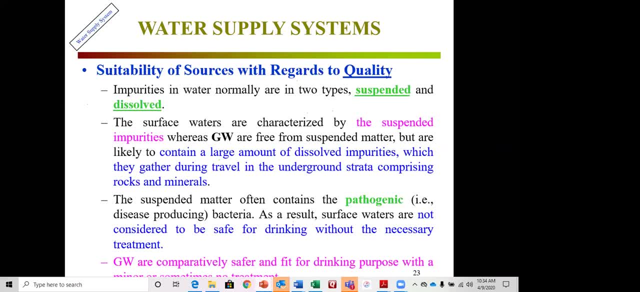 in the bottom. other one could be filtration right. so this is suspended if it is colored out, yeah, we can still do that, but we may have to do population population a little bit and and go from there and the dissolved one. a lot of iron materials, minerals, they could be. 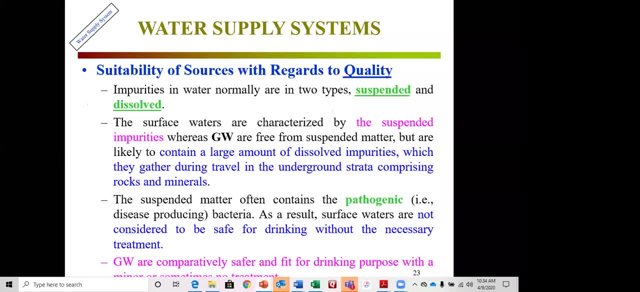 in dissolved form: iron plus, chromium plus, maybe calcium, magnesium plus. those will give us kind of hardness of the water. so in this case these are the dissolved, dissolved form. in order to treat the dissolved form definitely we have to have a chemical process, chemical precipitation and other process like 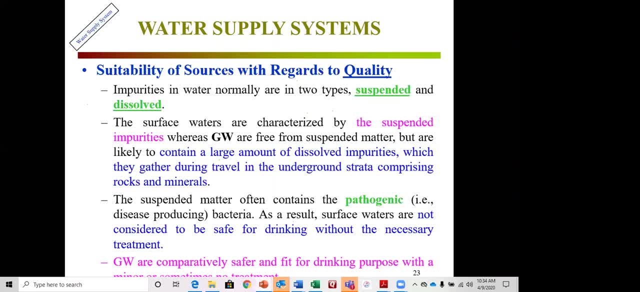 that in the treatment area. so we'll see a little bit of treatment for the surface water. we are suggestive of a brief description of that. so in this case the surface water might have a lot of suspended materials, or his ground water might have a lot of dissolved materials. the way that the process works, that's what most like. 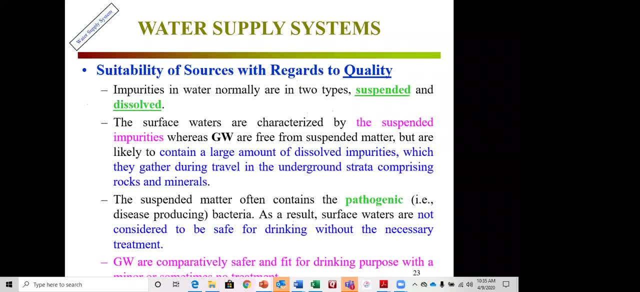 disenable to think the suspended metal open contains the pathogenic materials. pathogenic bacteria is a result of surface water. I'm not considered to be safe for drinking without the necessary treatment. so surface water we never recommend to drink. although it looks like in third world countries a lot of people they are drinking water directly from the river. 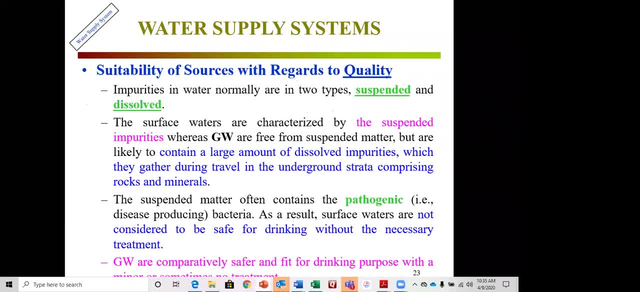 they take the water from the river and and do everything with this water at their home. still, they are surviving because of something: their water doesn't have any any bacteria or bacteria in there because of the natural processes being used in there. however, if it happens, then the lot of people who dies 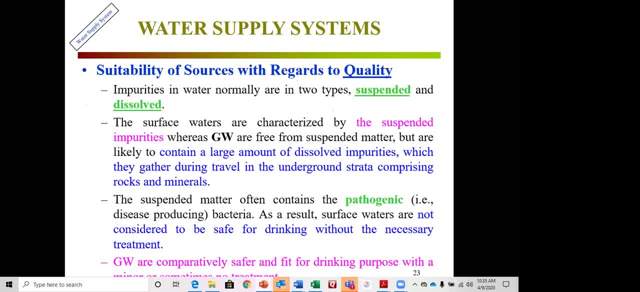 like a cholera. one time cholera was one of the epidemic right- I think it's long time in 1940s- around things like that. so at that time a lot of people died because they used to use the surface water, and surface water has a cholera. 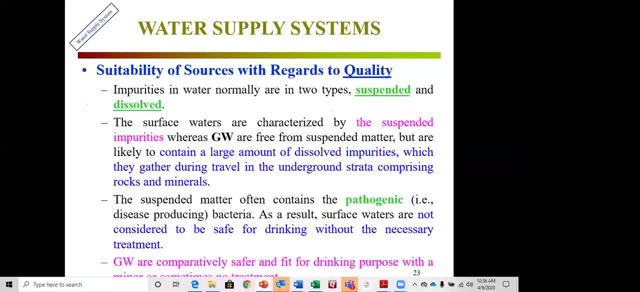 virus or bacteria, whatever is in there- pathogens mainly there- and they died. so groundwater, or compartmentalization of the water, is a very important part of the life of the people. so it's a very important part of the life of the people. so it's not completely safe to and fit for drinking purpose without any kind of treatment. 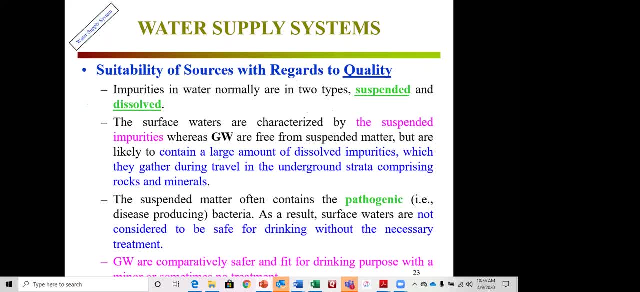 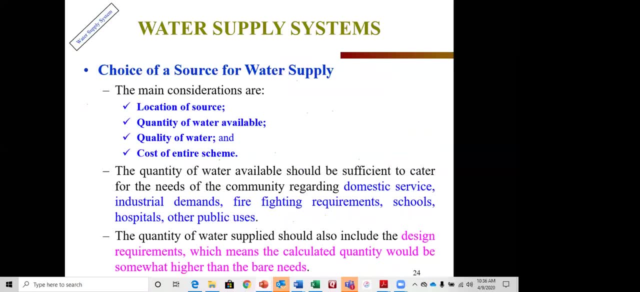 but better to have a treatment, at least the disinfection process, because you never know, there may be some contamination after you extract the water from the groundwater. okay, so then the the choice of supply, how we can choose one: either surface water or groundwater. if the surface water, if it. 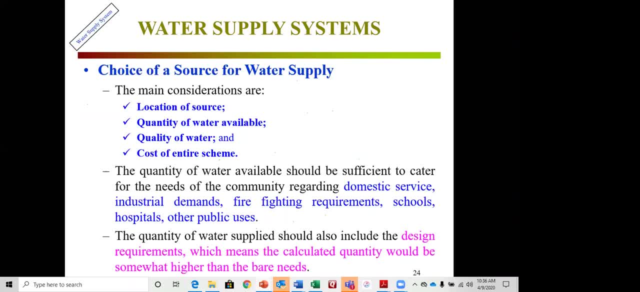 is the river, lake, pond and whatever we have surrounding areas. how we can select that location is very important location in terms of how much cost would be involved to get the water from this location to the treatment plant right. so meaning, if it is, uh, we are doing the. 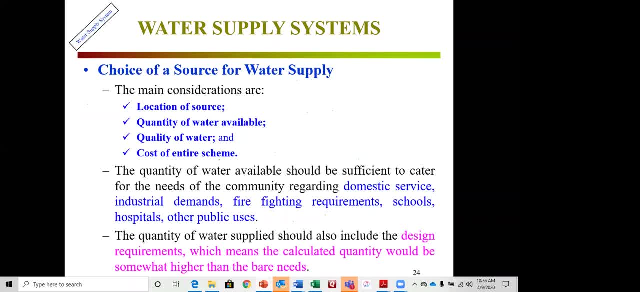 piping system, if this piping system is five mile, 10 miles, 15 miles or one mile, okay. so if there's a uh, if we would like to bring, do we have any hill in between? so we have to, uh, do a trance, maybe right to bring that, or maybe to above the uh, above the hill and other things like that there are. 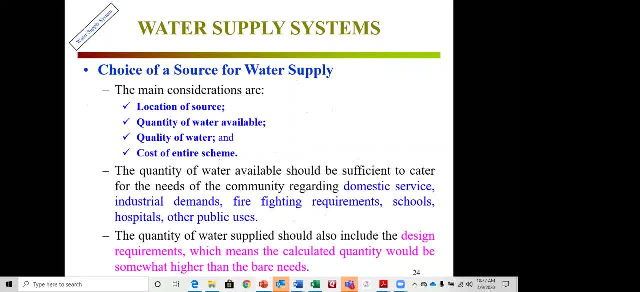 a lot of considerations in there and quantity of outer available. so we have to know how much water would be there in the source and quality and the last of all, cost of the entire scheme, meaning if it is a pipeline, how many, how long pipeline, what is the size of the pipeline? then what are 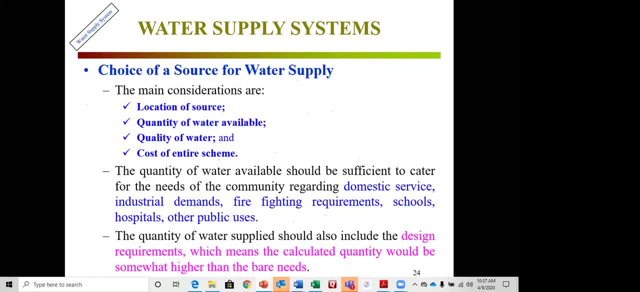 the different things. is a right-of-way bringing with somebody else property or if you bring it through that pipe? then you have to know what the right of way bringing with somebody else property is. uh, what is the right of way bringing with somebody else property or if you bring it through that? 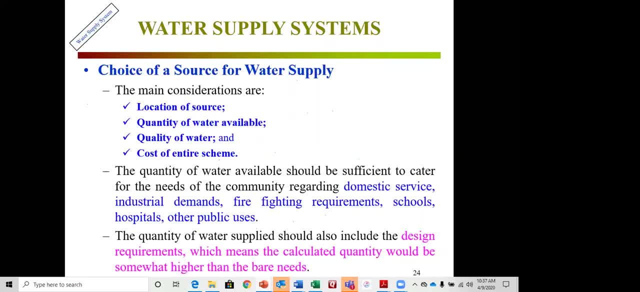 road system, is it? the road system could be like, say, too uh far away means if we bring it to the road system, then we may have to do a pipe system of, uh, maybe 25 miles, whereas if we can bring in the straight, straight line then probably only 10 miles, maybe, right. so if this is the case, 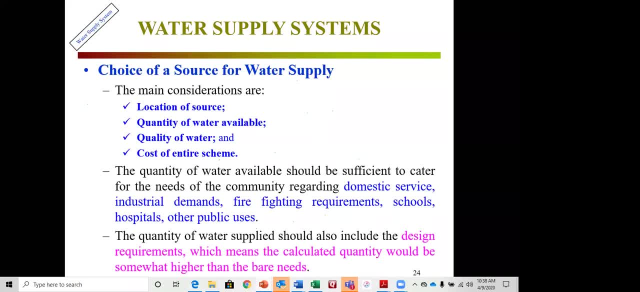 then state is better, but again the right of way, acquisition of the land and other things. so it would be a lot of consideration. so that's why the cost comes in there. the quantity of water available should be sufficient to cater for the needs of the community regarding domestic. 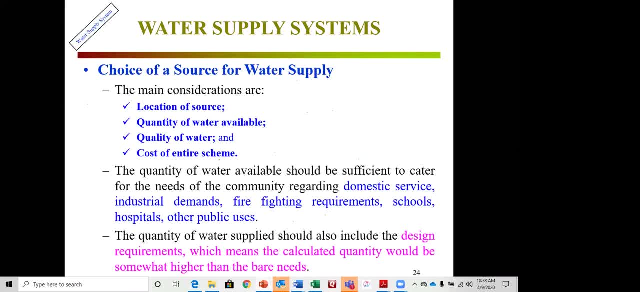 services, industrial demands, firefighting requirements, schools, hospitals and other public usage. so these are the kind of basically uh usage. they're necessary. the quantity of water supply should also include the design requirement, which means the calculated quantity would be somewhat higher than the bare needs. yeah, we are needs, uh, if we have a 100 million gallon per day. 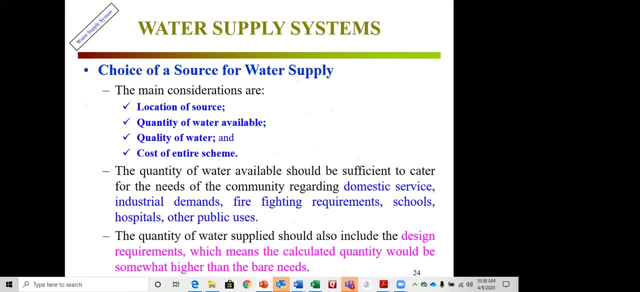 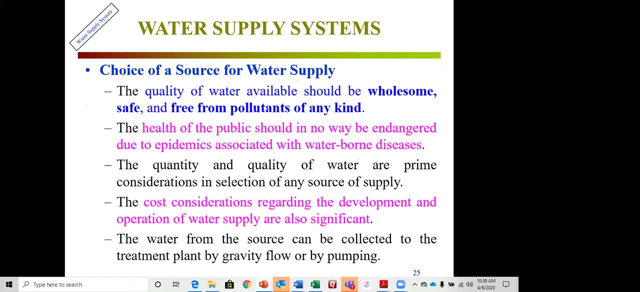 so probably we should shoot for 120 million gallon um per day, right? so that's why it's a little bit uh different requirements. so the quantity of water available should be wholesome, wholesome, you know that there should be uh exact amount of minerals and other things and should not be any toxic part of it. safe, safe. 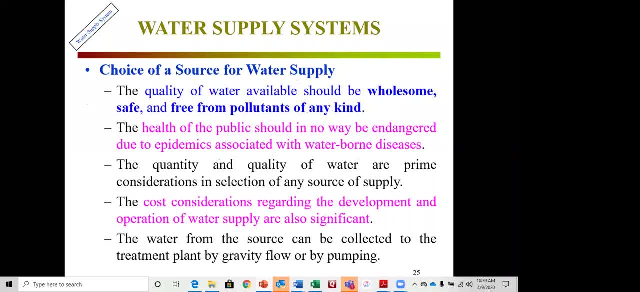 means, uh, portable, right, portable means there is no organism or pathogens there that can kill people and free from pollutants of any kind or other way. we can call it a wholesome is basically defines a very close to a palatable. okay, so the health of public should be, uh, should in no way be. then 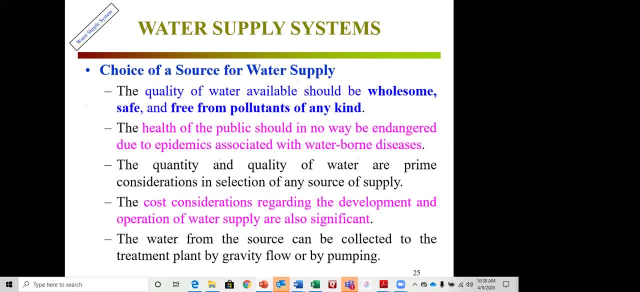 endangered due to the epidemics as well with the waterborne diseases. so in this case waterborne disease, we can control. that way the quantity and quality water are prime consideration and select selection of any source of supply. and the cost is definitely uh first consideration, but the the quantity and quality also are the kind of important. 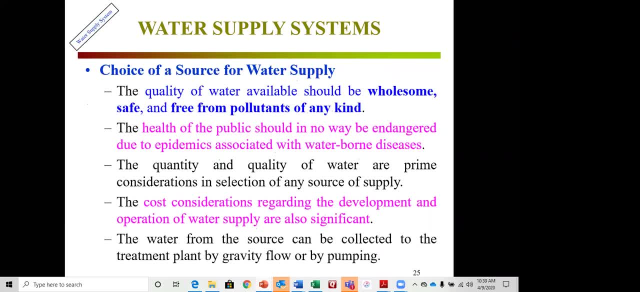 parameters to consider during the selection process. the water from source can be collected uh to the treatment plan by gravity flow or by pumping. so again, the gravity is not always we can desire, because if we have any, so far i have seen only one gravity lifestyle system. in my lifetime i have been going through a lot of water treatment plans and i have 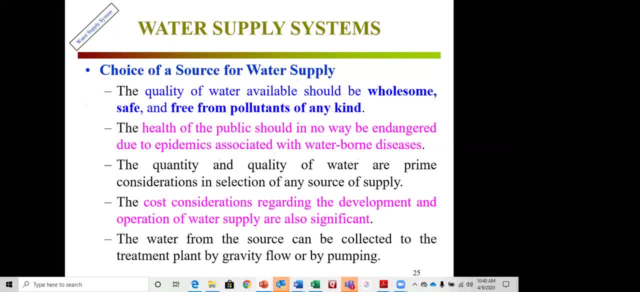 very few tenants that follow my plastic source treatment plan. i can sign up. позвол Portal. ona treatment plant was for a treatment plant with my students to visit and I have a field trip for them, but I have said so for only one in the current. 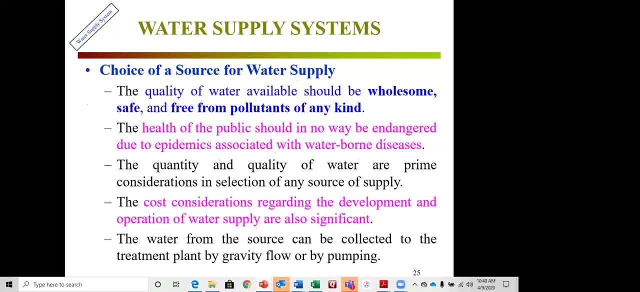 state that I have been living and they have a good one. they don't need to have any kind of pumping system because they are. river is a kind of the high elevation the area they are getting the water from and their water treatment plant is. I think it is almost 100 feet or maybe 120 feet down, so it has an 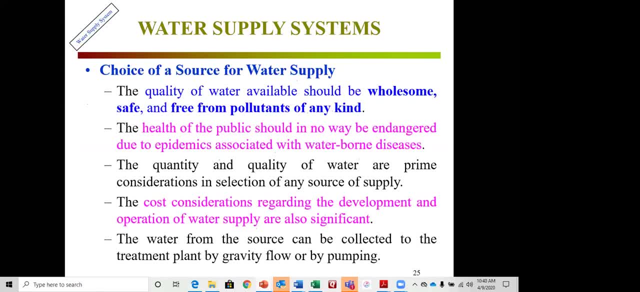 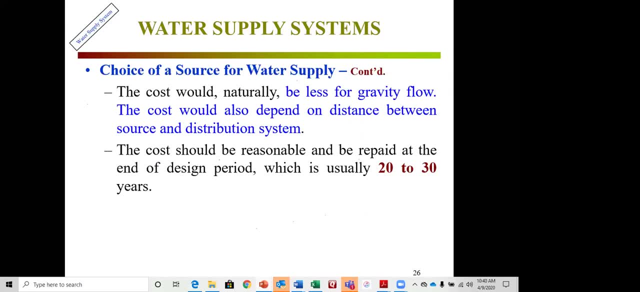 operation then to bring the water from there. yeah, so okay, the cost would naturally be less for gravity flow, obviously, because we don't need to build the pumping system as well as the other things. but the drain line- definitely pipeline- has to be there, so we have to bring the water. to make it kind of say, 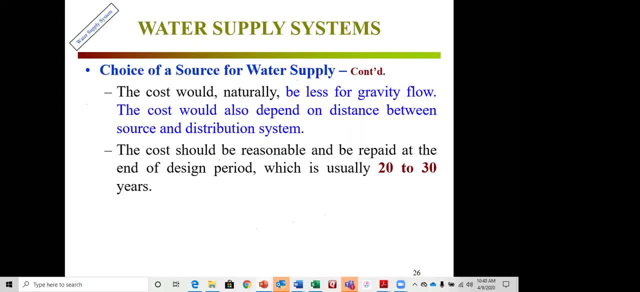 we don't want to bring with the surface drain right. that was didn't want to be good because a lot of people might trash something in. there would be kind of pollution being to get there. so again it'll be a distance and other things. okay, the cost should be reasonable and be repaid at the end of. 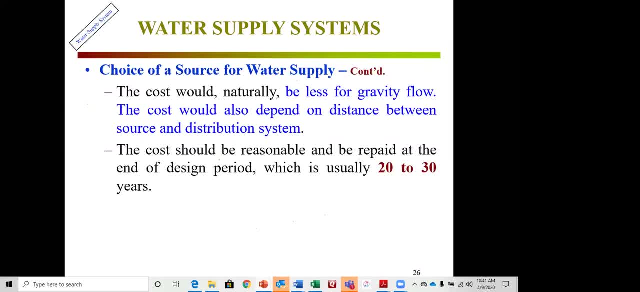 the design period, which is really 20 to 30 years. so with 20 to 30 years design period we have to equal the cost, all the cost. after that we have to make some profit, otherwise there is no benefit, even some of the company the way they do. 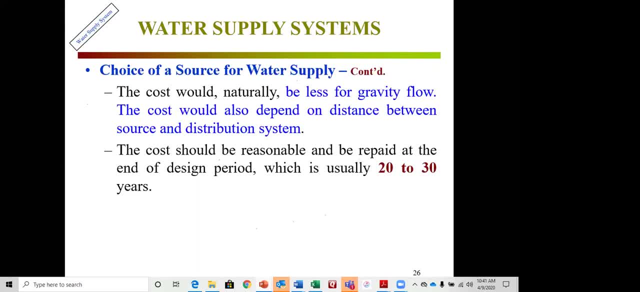 it and probably within a year or two they will have to make some profit. otherwise there is no benefit, even some of the company the way they do it, then probably within a year or two, then they would like to see the profit, otherwise it will not make any. 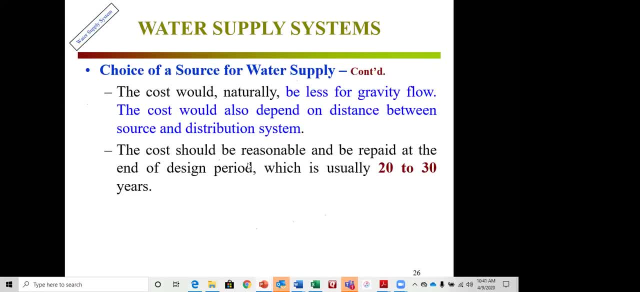 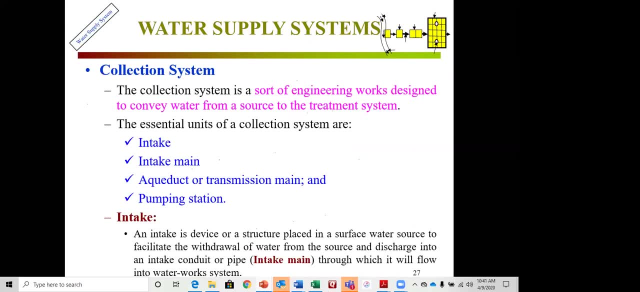 sense to them, in business sense of them. so collection system. next one is the collection system. so collection system I mean in here that we mentioned. this is the collection system right, the pump house suction main and the delivery main. so these are the one. so essentially units of collection system are intake. so 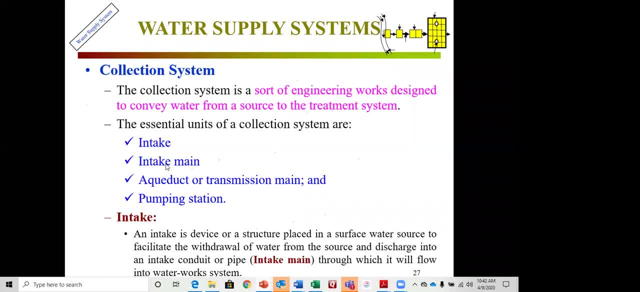 intake is one of them here. right Then, the intake main means the pipe system that is coming from intake to intake main, aqueduct or transmission main, and the pumping station. So these are the ones. I have an explanation for each of them. The intake: that is the conduit or an arrangement that we put into the surface water. 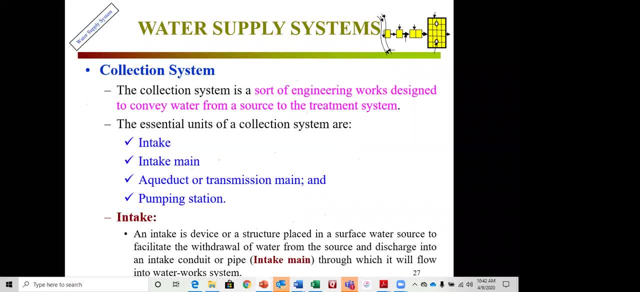 or we drown the water. So this is called the intake And the pipe system I think we have defined over here. So this structure right, The structure that we place in the surface water source to facilitate the withdrawal of water from the source and discharge into an intake conduit or pipe, is the main thing is the intake. 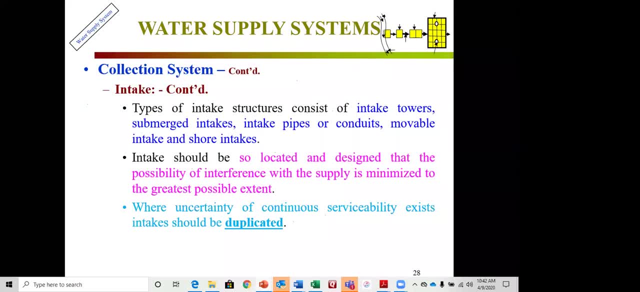 And whenever we put the pipe, it's called an intake main right. So then, the types of intake structure consist of intake towers, submersed intakes, intake pipes or conduits, movable intake and the shore intakes. As I mentioned, there are different ones. 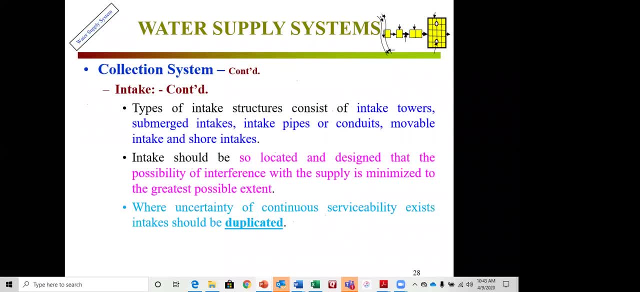 I think I have seen so far Five or seven, five, six, seven, something like that. So these are very good to design, But we have to design because it has to be customized for different areas, different ways. So intake should be so located and designed that the possibility of interference. 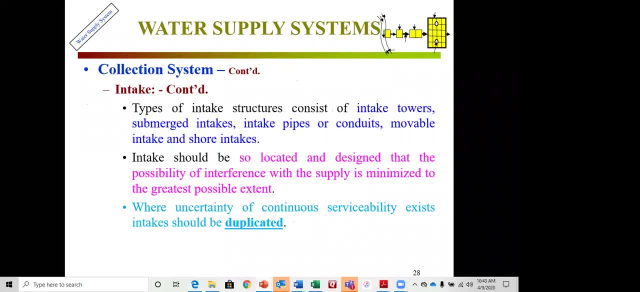 of the supply is minimized to the greatest possible extent, Meaning any damage or anything from the moating, swimming and other activities in the water and other things like that. But uncertainty of continuous serviceability exists. intakes should be duplicated. If we have two, then one can be serviced and the other can be still active. 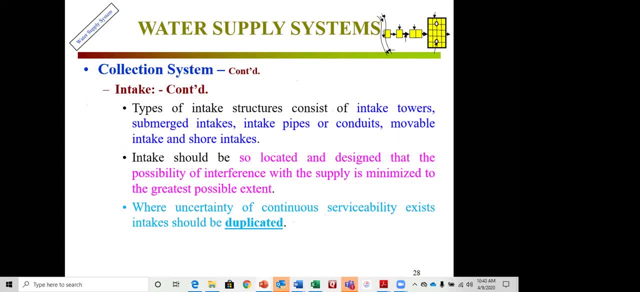 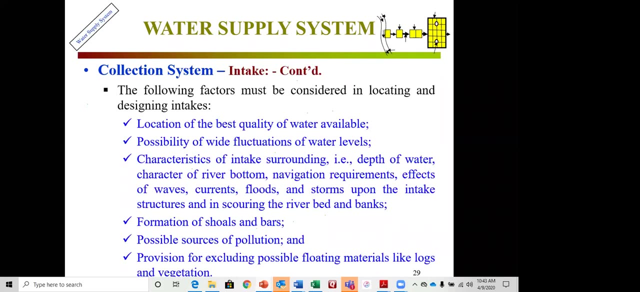 So that's why it's very important that we have two different intake and they are duplicated in there. So then the collection system, location of the best quality of the water available. we have to think that one. So these are the few factors that we have to consider. 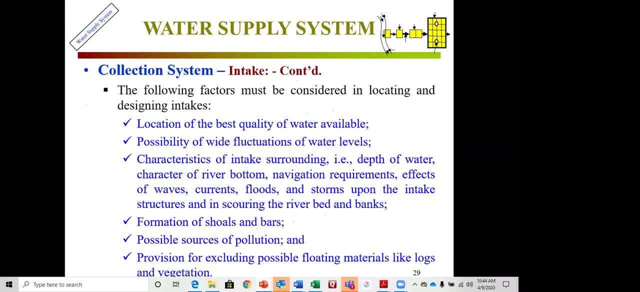 Okay, So for the collection system, wide fluctuation of water levels, maybe it's not a good idea, right? So characteristics of intake surrounding: So yeah, whether it's a, if it is the river, if there's stable area or too much current in there. 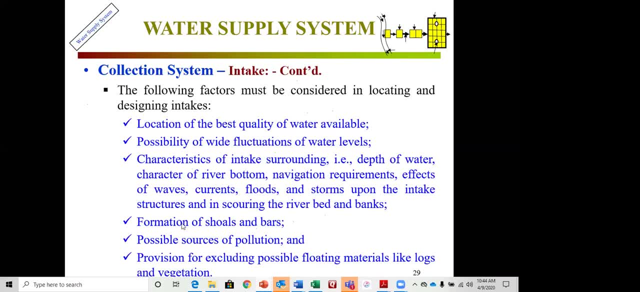 So their permission of showers and bars and possible sources of pollution. If we select something that is downstream of a discharge, then it's not a good idea. It would be- and if the more discharge is maybe allowed, then it's not a good idea. 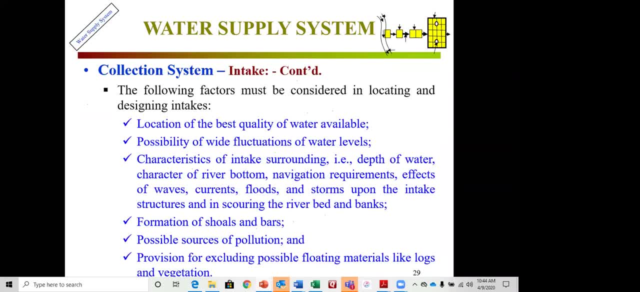 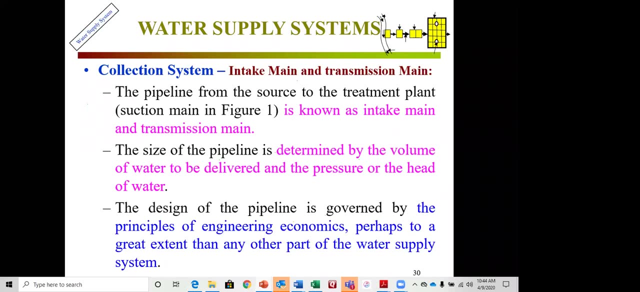 If it's not allowed in the future, then it could be a problem too. And provision for excluding possible floating materials like logs and vegetation That might damage the intake system inside the water. Okay, Then the intake main and transmission main. as we've mentioned before, the pipeline from 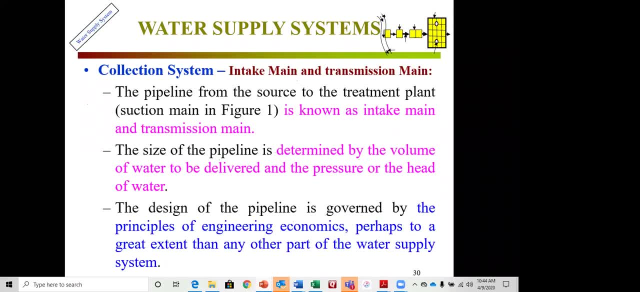 the source to the treatment plant. section main and figure is known as the intake main or transmission main. The size of the pipeline is determined by volume, order to be delivered, The ratio of the pressure or head of the water, Basically in this case Q equal to area times, velocity A, B. 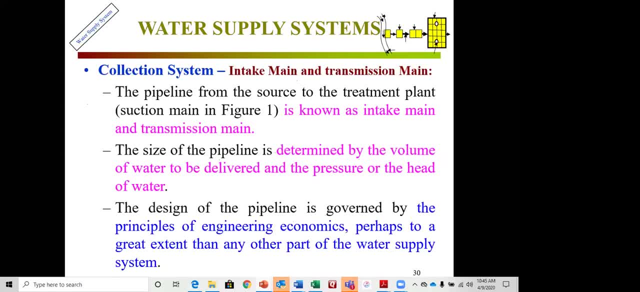 Right. So if we can have a velocity, certain velocity, we need to provide for certain Q. then we should be able to design the pipe size and other things. Design of the pipeline is governed by the principles of engineering economics, perhaps to a great extent than any other part of the water supply system. 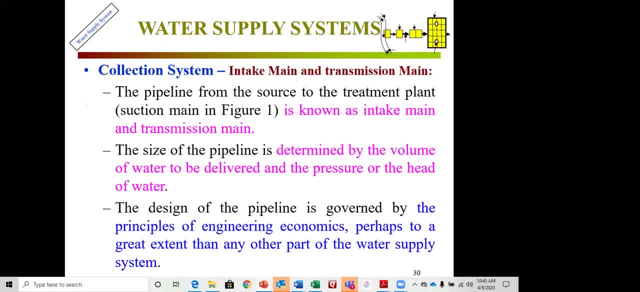 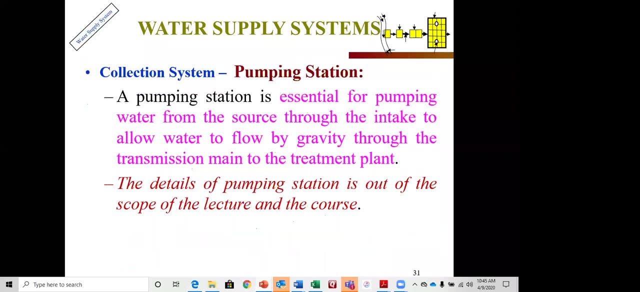 Yes, engineering economics is very important because of so this driving our cost, the cases, even business point of view and other other technical point of view, and things like that. Pumping station: pumping station is essential for pumping water from a low elevation to the high elevation where the gravity doesn't work. so in this, 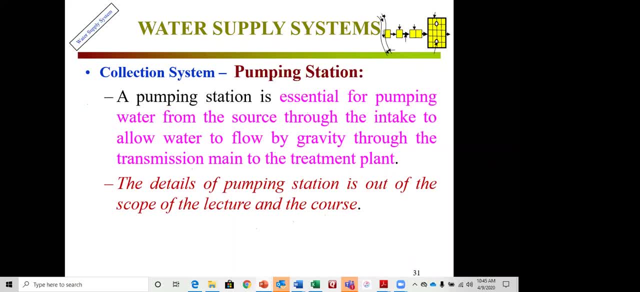 course of pumping. we are not going to discuss more about the pumping in this course. Okay, before we go to the treatment process, let's see whether we have any questions in there. I'm going to go to chat box, Okay, so no questions, looks like. If you have any, 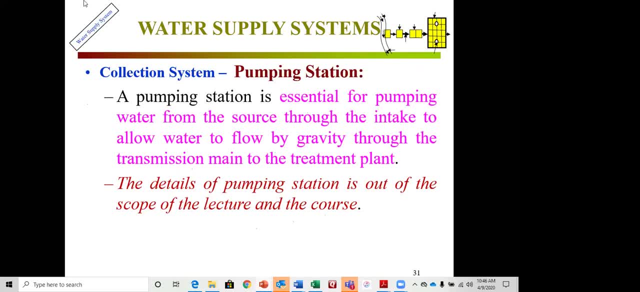 questions. you can type in the box now and we can discuss. So far we covered right a little description of the the elements of the water supply system. I think I have come up up to the collection system. then we have two more treatment and distribution system. 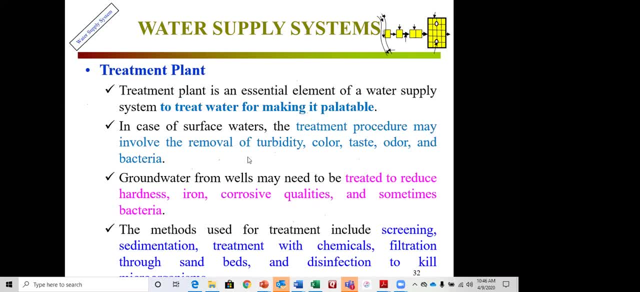 Okay, our next one is the treatment plant. As we mentioned that, the third element in the system is called a treatment plant. So treatment is necessary to make the water portable or safe, whatever we call it, and the whole sub maybe palatable, right? So that's why we need the treatment process. So 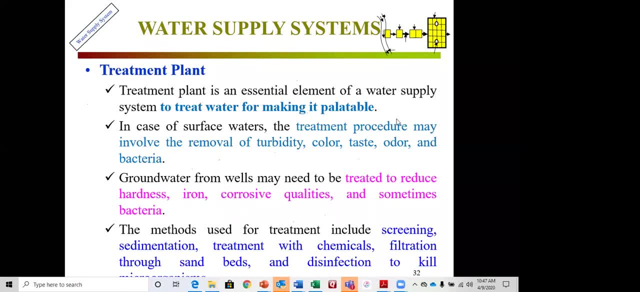 here I use the word palatable. Palatable means pleasant to drink, pleasant to see. Okay, it doesn't have any color or anything like no suspended material In case of surface water treatment procedure may involve the removal of turbidity, color, taste, odor and bacteria. Yeah, definitely, there are maybe few more. 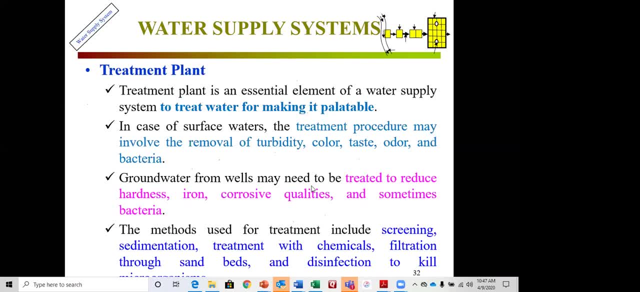 things in there. The groundwater from wells may be may need to be treated to reduce the hardness. I mentioned that. the iron means another kind of minerals in there, Corrosive qualities and the sometimes bacteria, Not always, as I said, sometimes depending on what layer you. 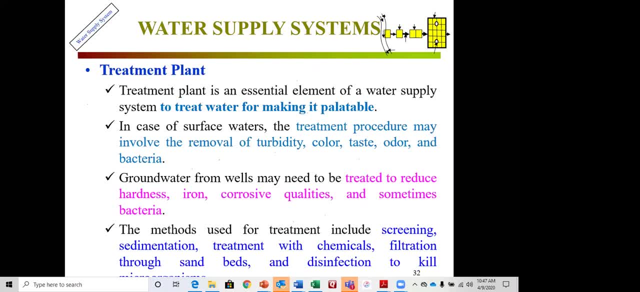 are getting the water from and how well the aquifer is being managed in different ways, or whether any leaks anywhere. directly that can microorganism can go, or bacteria can go, or maybe what is called the pathogens can go. The methods used to for treatment include screening, Screening. 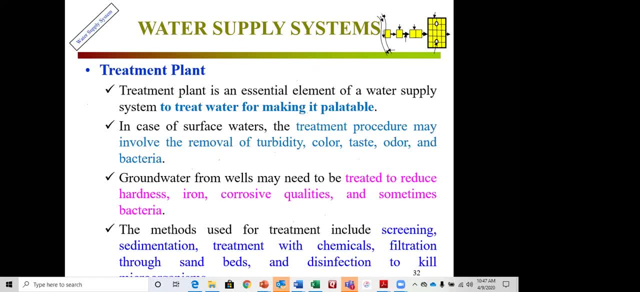 means basically taking out the bigger part from the sedimentation of the surface water. You can also do treatment with chemicals. that mean chemical treatment like coagulation, flocculation, filtration, you know, to send bags, and disinfection to kill microorganism and other things like that. 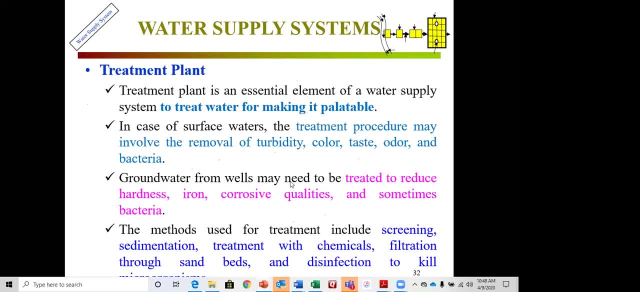 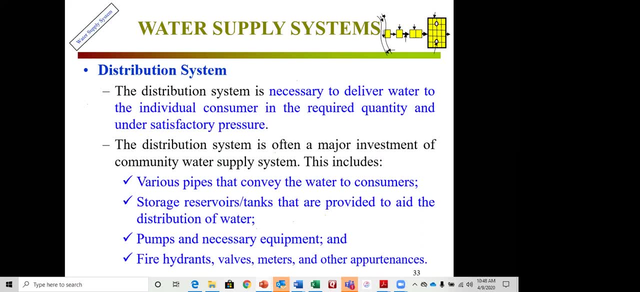 So disinfection is the technical last one. Okay, then the distribution system. The distribution system is necessary to deliver water to the individual consumer in the quantity and under satisfactory pressure. whenever we say pressure means you guys understand. the 50 to 60 psi pressure is a kind of recommended for the houses. if 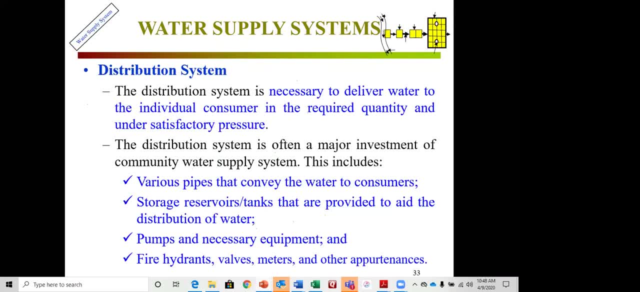 you have a 15 psi in your house, then I don't think you like right. or if you have 100 psi, then everything would be kind of your pipe system and other thing may be damaged, those things like that. so our distribution system is often a major investment in there because we have seen that this is the one in here. 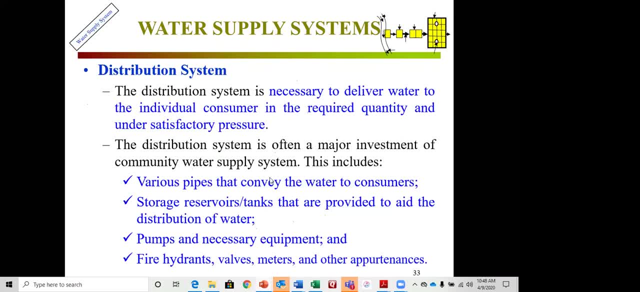 this is the one right. so it is a major investment, definitely so. it's a combination of various pipes that convey the water to the consumers, storage reservoir tanks that are provided to aid the distribution of water, pumps, and necessary equipment, fire hydrants, balls, meters and other opponent appurtenances. so these are the one definitely is a part of distribution. 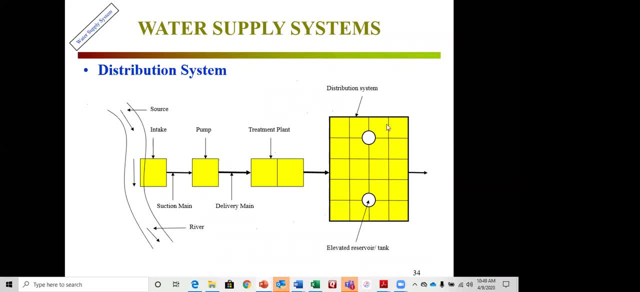 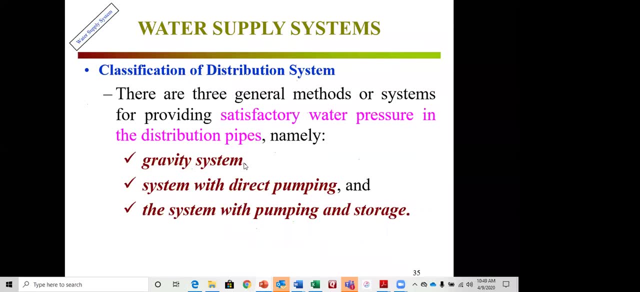 system. okay, so in this case this is the distribution system, right? this is. I'm showing it again, repeating this picture, just to make sure that we understand that. okay, then classification of distribution system. then there are few. classification gravity means directly coming from the higher elevation to the lower elevation. okay, that means we are not pumping there. 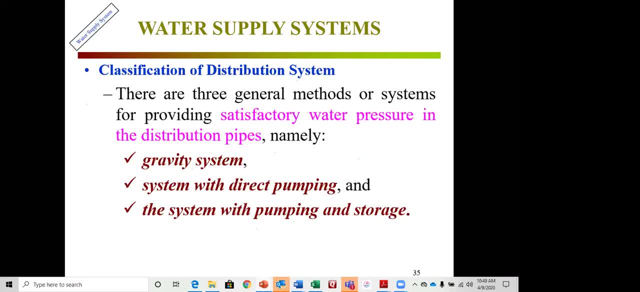 is no pump involved, so gravity. then the second one is the system with direct pumping. so I think most of the US cities in a district cities they use this one right, so they use this this one anyway, the system with pumping and storage. are some of these city counties? 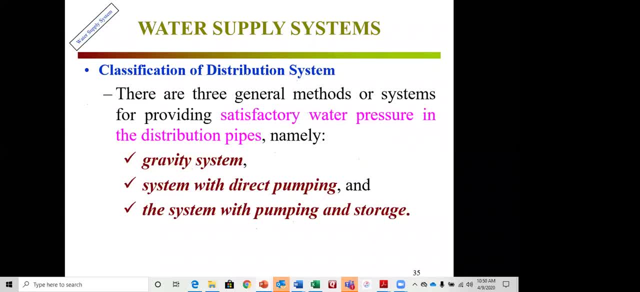 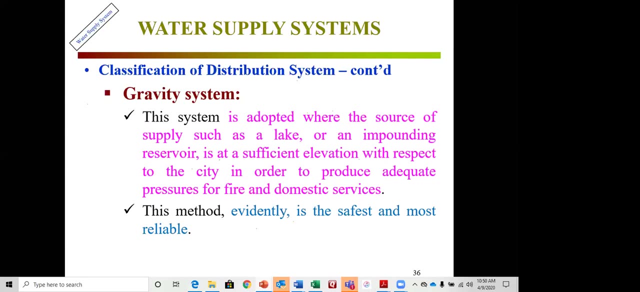 they use that. if you see a water status tank in there for different citizens, counties, that means they are using the third one right and not for the whole area, maybe, maybe certain part of the area they serve. okay, gravity system is the easiest one. okay, gravity system is the easiest one. it is adapted for the. 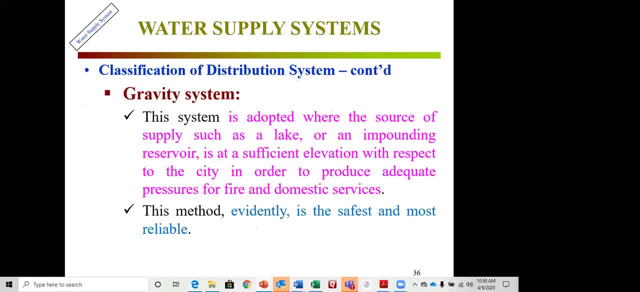 source of supply as a lake or the impounding reservoir at the sufficient elevation with respect to the city to provide enough pressure in there. This method, evidently, is the safest and the most reliable, and more cheapest also could be cheapest- Safest, most reliable and cheapest because a lot of energy. 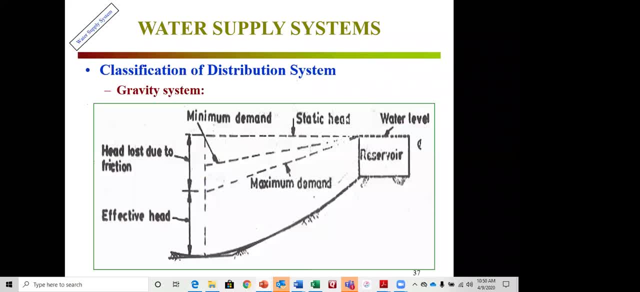 involvements are not there. So this is the one shows, like, say, gravity system, because if we have a reservoir, that means a reservoir or anything like that- water level is there, then definitely you can get the water in here. So this is the effective head and this is the total head right. So head loss due to the 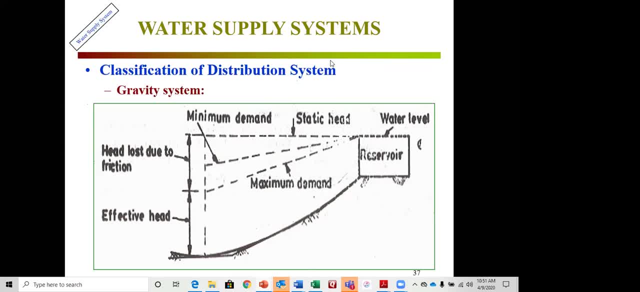 friction. So if we know that it's a pipe, you know how to calculate that friction loss, right? So using Darcy Weisbach equation. we'll see it later on when we'll solve some problem using the energy equation and other things like that. So 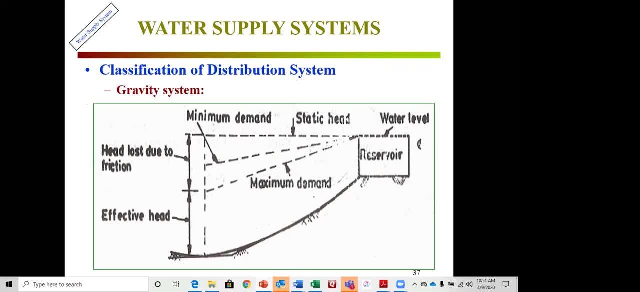 we should be able to see it in there. Now, I don't know that you guys know it, but usually what happens is that the water level is there, So if we have a reservoir, that we have to provide pressure to the pressure. So what happens is like, say for 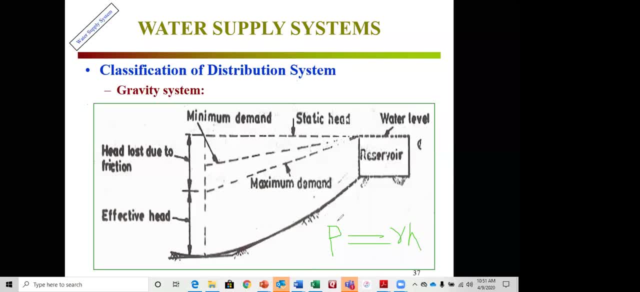 P equal to gamma H, right? So if we know P equal to gamma H, then if we need to provide the pressure, say, for example, 50 psi, say 50 psi in there, So how much height we need, So how high it should be. this one compared to that, So it comes out to be around: this one is 115.. So how I got it, like say it would be 50.5, is the right. 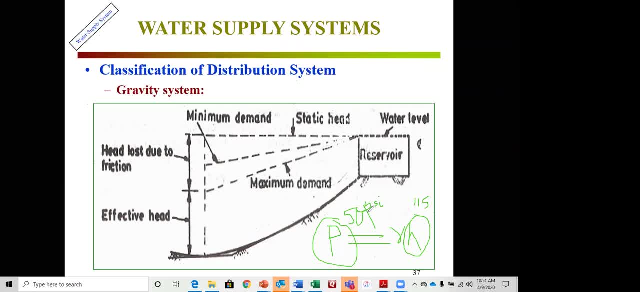 times 144, converting to PSF 50 times 144. then divided by gamma, right, gamma is what? gamma is 62.4. so then it comes 115 feet. so this is 115 feet is without the last part of it. that means this is showing the whole. I mean just this thing. 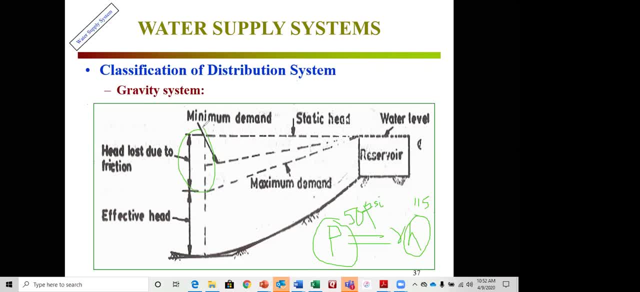 right, just this. so if we consider the this part of it, then definitely may have to add few more feet in there. I would say another 10 to 15 feet, meaning in this case 25 to 30, 30 feet right 133 down that we need. so if we have, 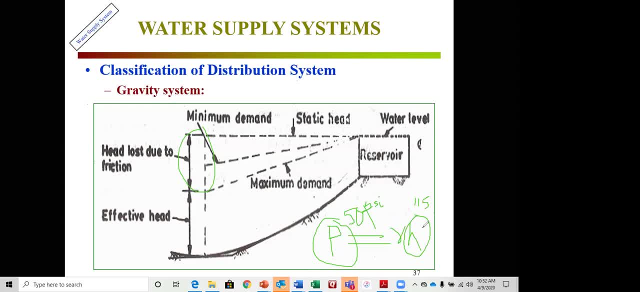 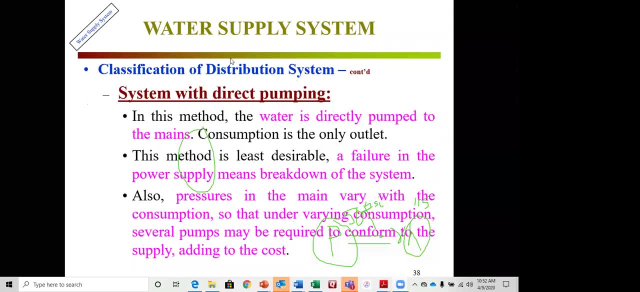 elevation, that one. that much then. yes, we should be able to use it as a distribution system, you okay? so then the system with direct pumping: the method: water is directly pumped to the individual houses, the mains and other things like that. so the this is least desirable. why the failure of power supply then break down the 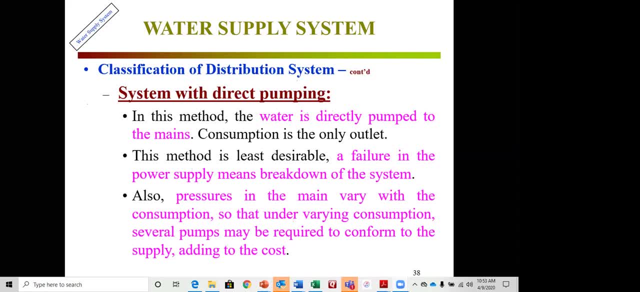 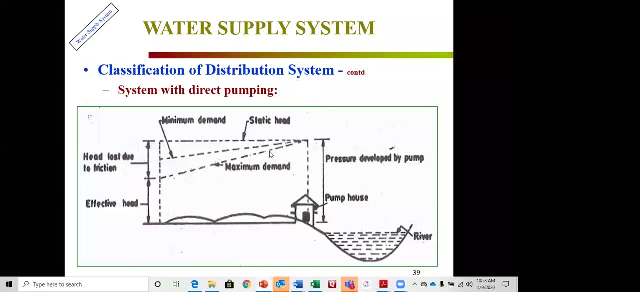 whole system ratio in the main vary with the consumption, so that they, under varying consumption, several pumps may be required to conform to the supply adding to the cost. yeah, it's a lot of pumping in there. so I think I have a picture- that one- to show you. so this is the picture here looks. 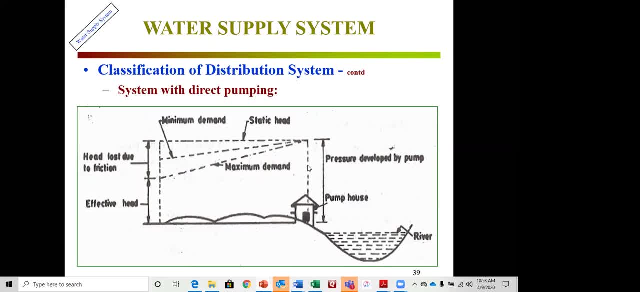 like. this is the pump house. they are pumping water from there and providing the high this pressure head by the pump. okay, so this is a loss. this is the effective one. so somebody here is getting the water. this is a direct pump. another one. I showed you the picture right. see the we are pumping, putting the. 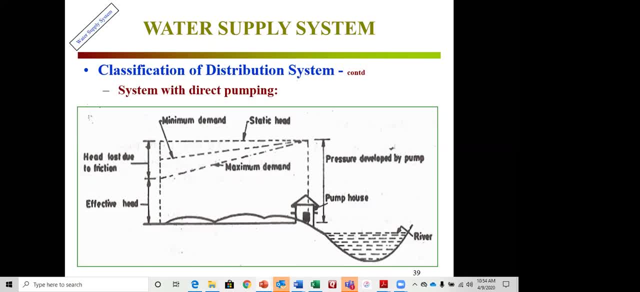 water back, when back to the tank or what is first and when we don't need it and also we didn't the other way. we are bringing it back whenever we need it, based on our demand changes and we know that whatever is demand or whatever is supply that we may have. 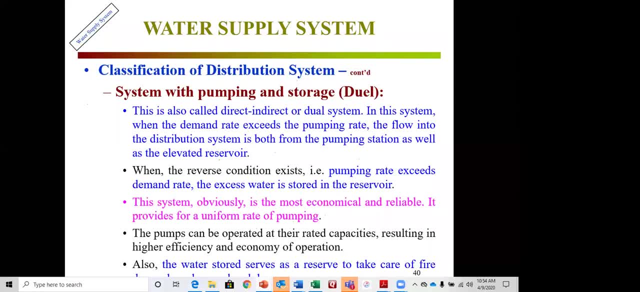 you. okay. the system with pumping and storage is a dual system. this is called direct, indirect and dual system. in this system, when the demand race exceed, like this is explanation already I did before- is our reserve condition exists, pumping race exceed, demand rate, the excess water is stored in the reservoir right. I already 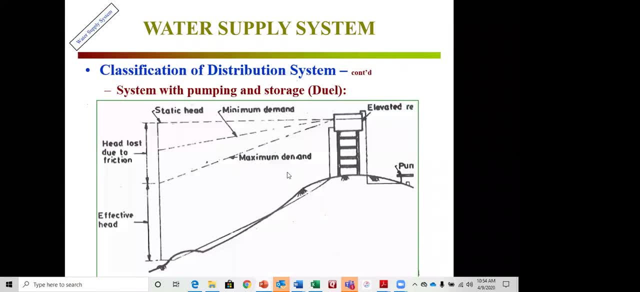 explained one with the picture that I had in there before, so here is the one. that's happening. this is the pump house. we are pumping it here as well, as we pumping directly to here. so, and this is the pump house, we are pumping it here as well, we hand this to the top. thank you, Mr king, speaking out for us. 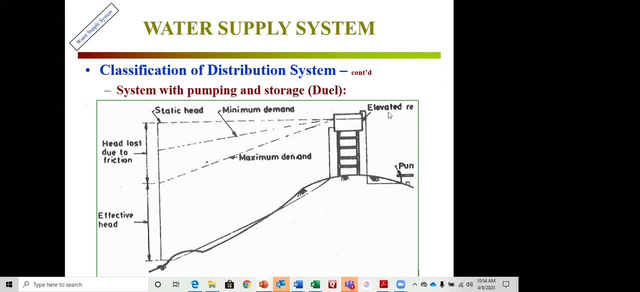 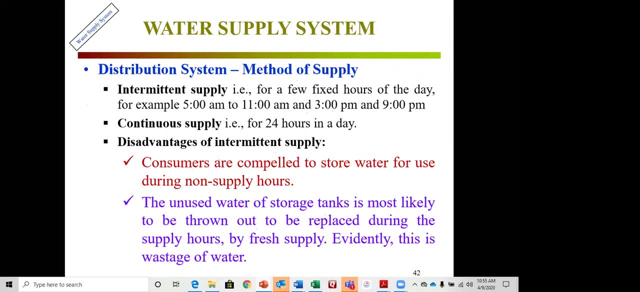 uh, third, um, so, and we are supplementing or something like that whenever we need more water that we are not like pumping. so this is basically the dual system. okay, the distribution system, method of supply- also method of supply could be intermediate- and the continuous. that's what we see most of the time here in the 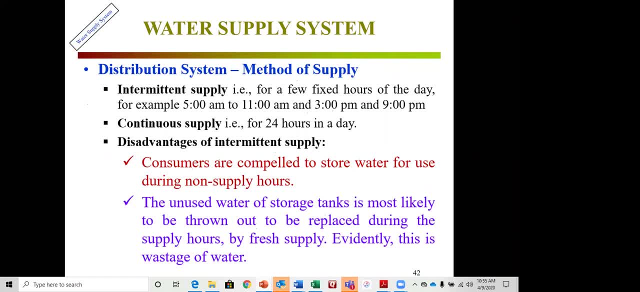 the water supply will be there. So some of the disadvantages of intermittent supply are consumer are compared to store water. whenever they don't, they feel like the water will be gone in a few minutes. And the other one is unused water. sometimes they don't use the whole water during the off time. 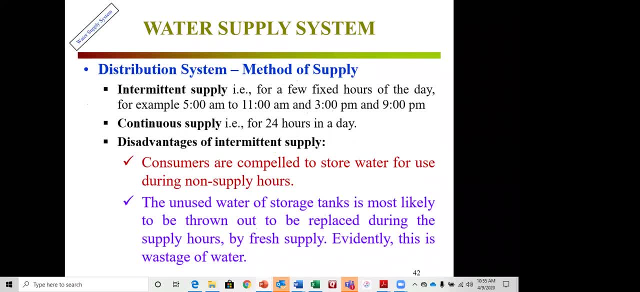 then they trash it. when the new water comes in, then what they do- definitely they what is called they restore the water- right, They trash the old water and restore the water. So this is kind of waste. It's again mentality issues and other things like that. 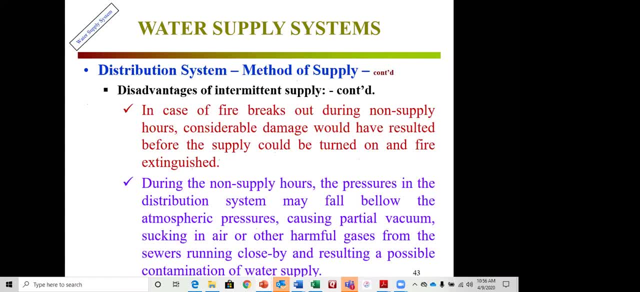 Okay, disadvantage In case of fire breaks, breaks during the non-supply hour, then it would be very dangerous for us. During non-supply hour the pressure in the distribution system may fall below the atmospheric pressure and they create some vacuum. 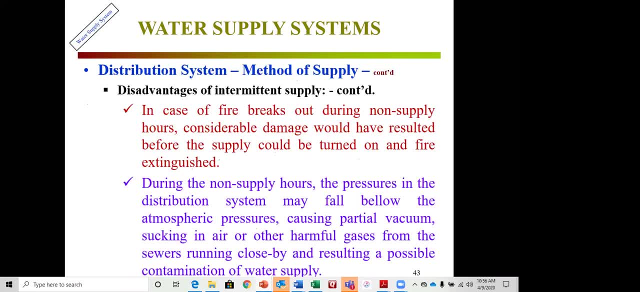 Means. they can have a lot of air in it in there, So that means in this case is very harmful. very vacuum can create a lot of suction and other things. Ultimately it can damage the pipe system and other things like. So this is another bad part of it. 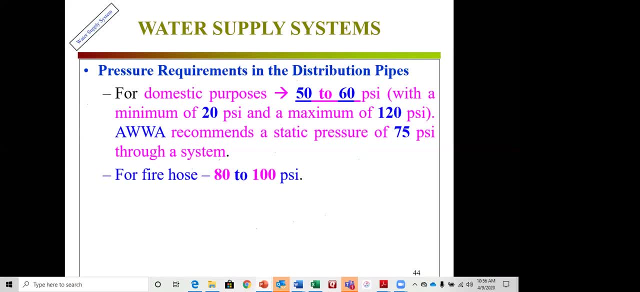 So pressure requirement in the distribution pipes is, as I mentioned before, 50 to 60 PSI, with a minimum of 20, maximum of 120.. I don't think 120 is really necessary, because 120 can give us very hard time. 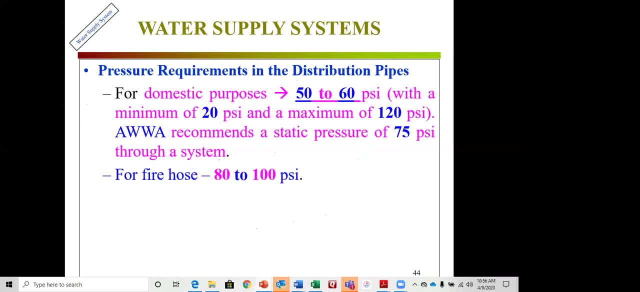 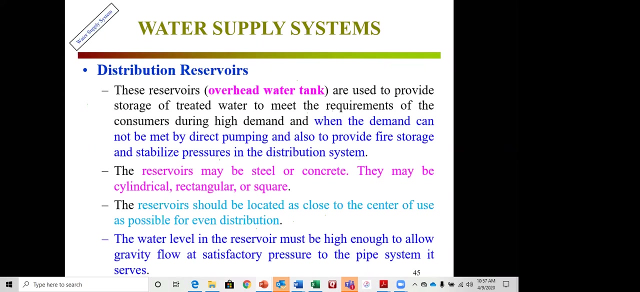 And AWWA recommends. They recommend 75,. okay, And fire hose requires 8,200 PSI because they need a little bit bigger pressure to take out different areas and other things like that. Okay, distribution reserve work means overhead storage tank are used to provide storage of treated water. 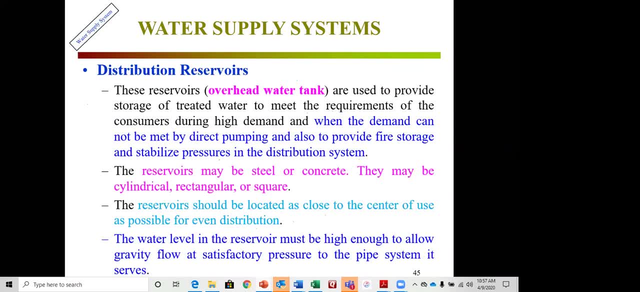 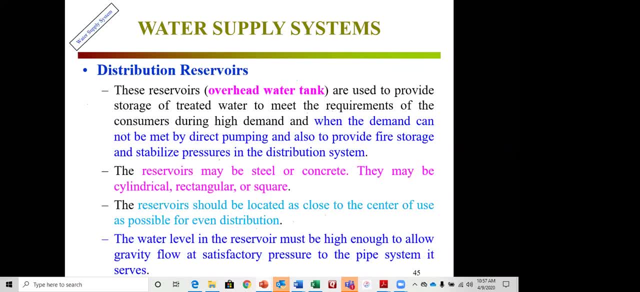 So this is another bad part of it- And also prepared fire storage and stabilize pressure in the distribution system. Okay, that sounds very good. And the reservoirs? maybe steel or concrete, They may be cylindrical, rectangular or square. Most of the time the picture that I show you. 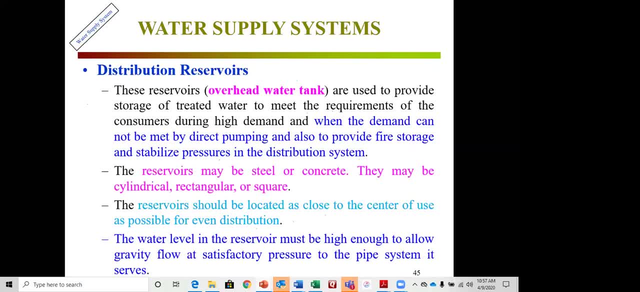 is the cylindrical, So I'll design it also a cylindrical one, not the rectangular one, but you can use any shape, because of this is basically what is it? arbitrary, right, arbitrary of the designers. so you can use it, but there are some advantage disadvantage on those. the reservoir should be located as close to the center of use as possible. 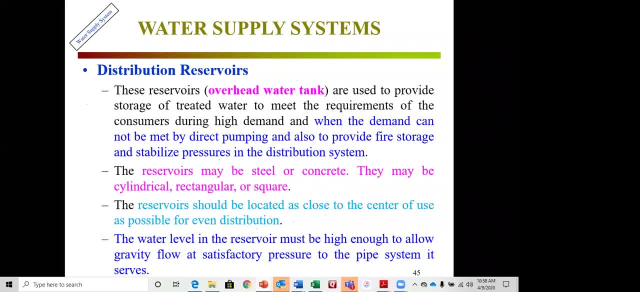 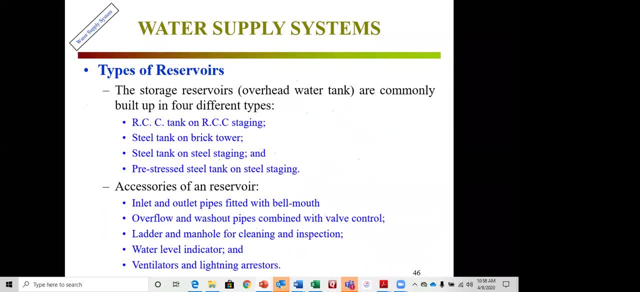 for even distribution, the water level in the reservoir must be high enough to allow gravity flow at satisfactory pressure to the pipe system. it serves okay. so here are the different types: RCC tank on RCC staging, steel tank on reed tower. a steel tank on steel staging and pre-stressed. 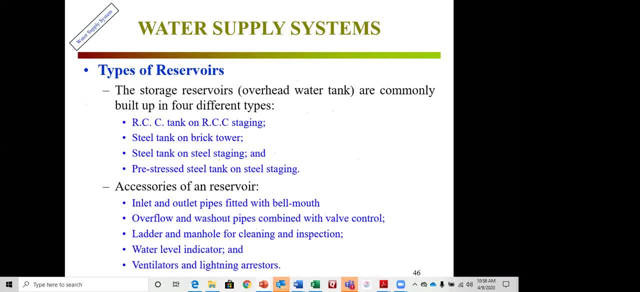 steel tank on steel staging. so whatever works out right. accessories for in reservoir is inlet outlet pipe speeding with Bell mouth, our flow and washout pipes combined with mouth control later, and manual for cleaning and inspection. water level indicator- I mean the way the water level is. I think this. 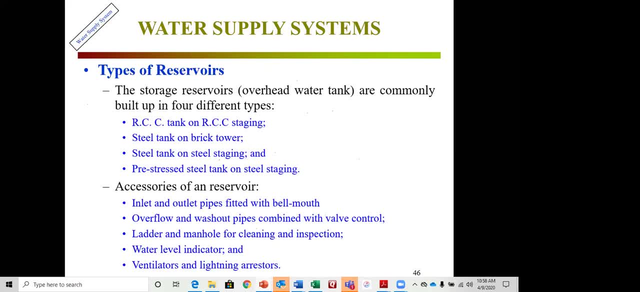 is a automatic system. you guys can. I think most of the time we do it from there, from floating point of view, how much water we have in there, whether we need to put more water there or not, and the ventilators and the lighting and restores, and also I think there is overflow is already. I. 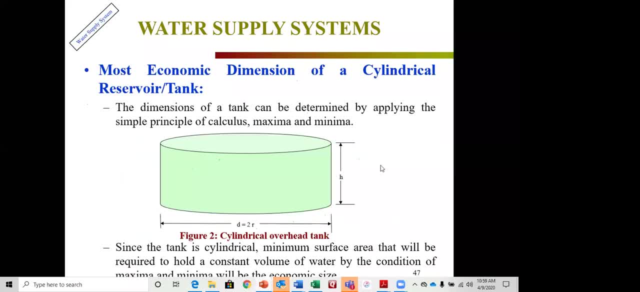 mentioned over here. the overflow thing is there. okay, mostly economic dimension of the cylindrical reservoir. as I mentioned that the reservoir could be any size, like said, any shape and cylindrical, rectangular, triangular, right another other shapes of all. so we'll do the cylindrical one, most widely used, and it gives us kind of better hydraulic section also. so in this case 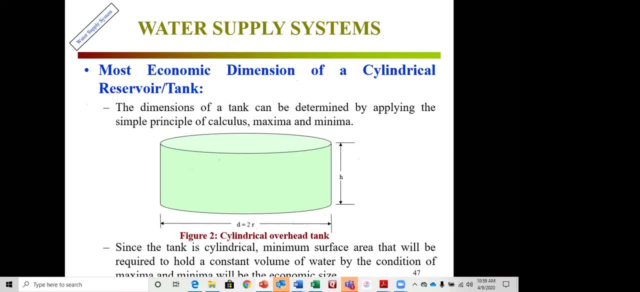 we'll design something most economic. the dimensions of a tank can be determined by applying the basic, simple principle of calculus makes him a minima. so, since the tank is cylindrical, minimum surface area that will be required to hold the constant volume water by condition makes a minima will be required to hold the constant volume water by condition makes a minima will. 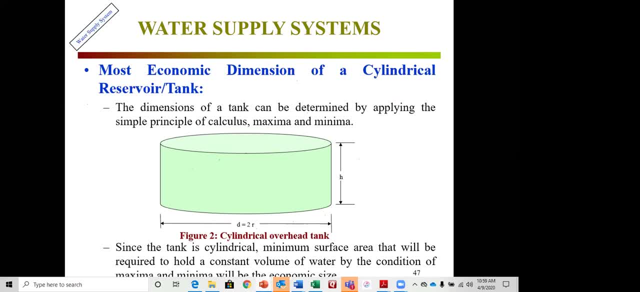 be the economic size. so in this case, surface area would be our main thing. there are two surface areas. one is the bottom, other one is the side right circumference on the side top. I'm not going to use it because top is a kind of like, say, it's not in contact of the water anyway, right, so we 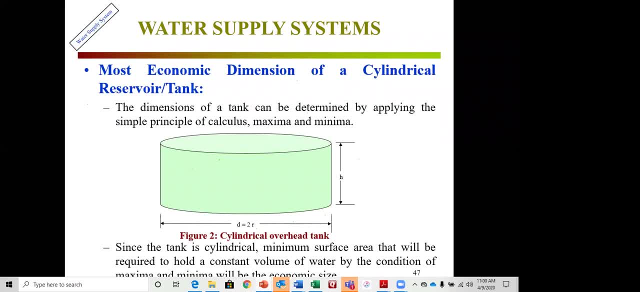 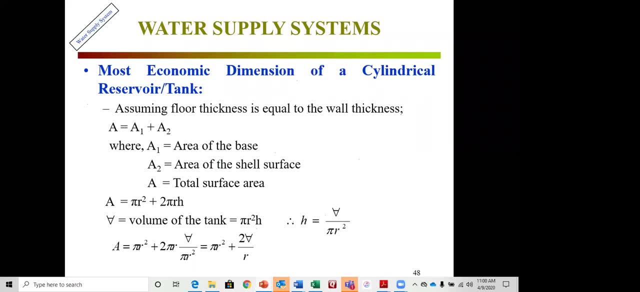 put some freeboot and it's just covers it so it doesn't get the rainfall and produce the water. so assuming the floor thickness is equal to the wall thickness, then the surface area of the total surface area equal to a would be a1 plus a2, where a1 we can consider the base right. 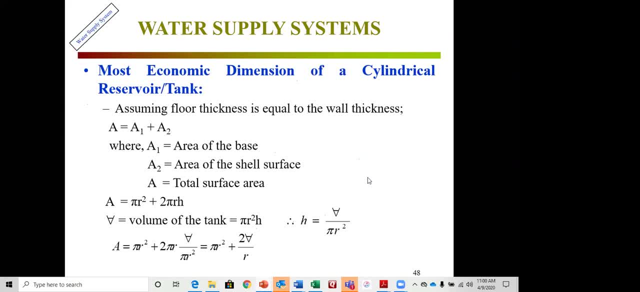 you consider the base and the a2 is the surface. is that wrong? so then that means to the linear, a would be surface, would be pi R square right or pi D square by 4. but I have used pi R square here. okay, pi R square here, and 2 pi R. 2 pi is the circumference, says H. if I multiply with H will give me the air, the, the. 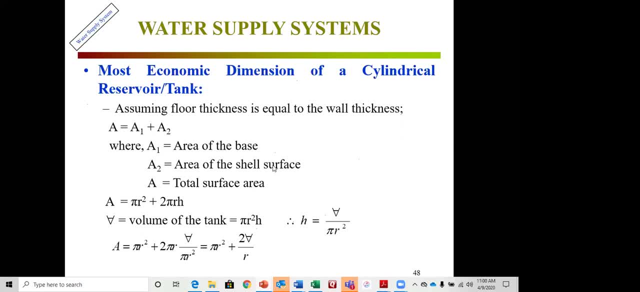 area circumference length is 2. pi R then multiplied H will give me the area. so in this case the, the V, can be defined as pi R square H volume. okay, pi R square into H is the volume. so then the H can be replaced by volume. volume is a constant V, by pi R square. then we can replace- here I had two parameter. 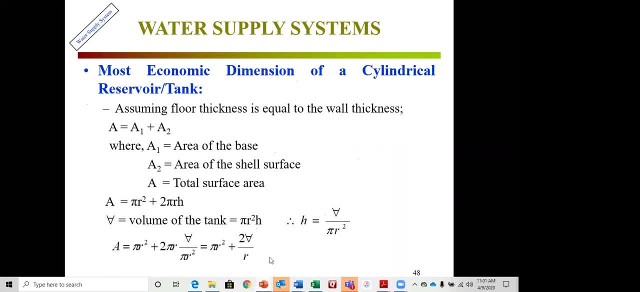 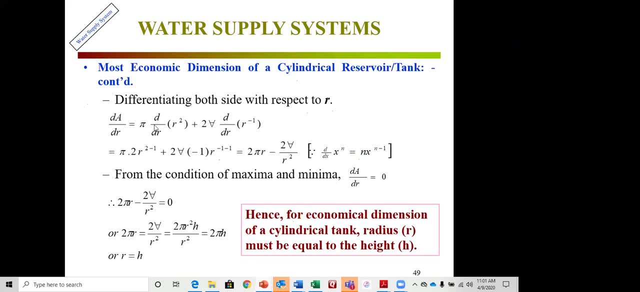 here R and H. if I replace the H, this equation becomes only: a is a function of R. now we'll take the derivative with respect to R, da over dr. so we get something like that: ultimately, this is the one. okay, this is the one. now we'll put, uh like say da over dr, equal to zero. if we put equal to zero, I. 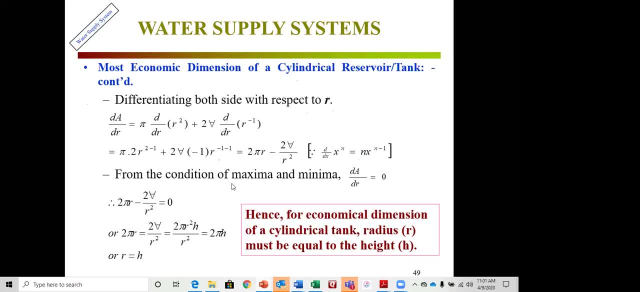 can, uh, we get r equal to H. that means the radius of the the cylindrical tank is equal is equal to the height of the tank, okay, or diameter is the double of the height. so that's why, hence, the economic dimension for the cylindrical tank radius must be equal to the height. so that's what we'll be using. this is the. 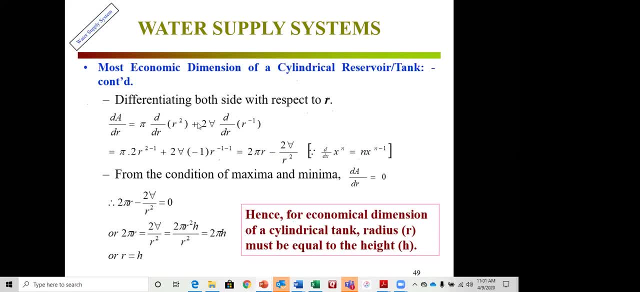 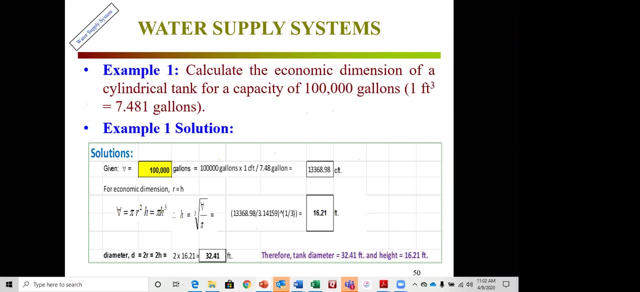 basic principle and it came from uh, mathematics like maximum, minima and differential equation. I mean, the best hydraulic section could be another way to think about it. and for the mechanics point of view, okay. so here is the problem that I would like to solve: uh for designing the overhead. 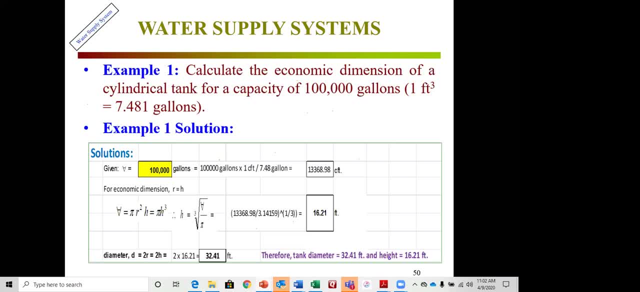 storage tank. so we are requiring: calculate the economic dimension of a cylindrical tank for a capacity of 100, 000 gallon. one cubic feet equal to seven point four, eight, one gallons. so calculate the economic dimension. and here what I did: here I convert the, the gallon into cubic, excuse me, gallon. 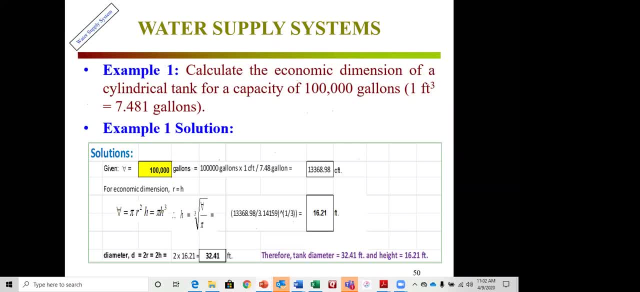 into cubic fit. so what? I had a hundred thousand gallon. then, uh, divided by seven point four, eight gallon, equal to one cubic fit, I got thirteen thousand three hundred and sixty nine about nine cubic feet. now we know that for economic dimension, right, for economic dimension, here we 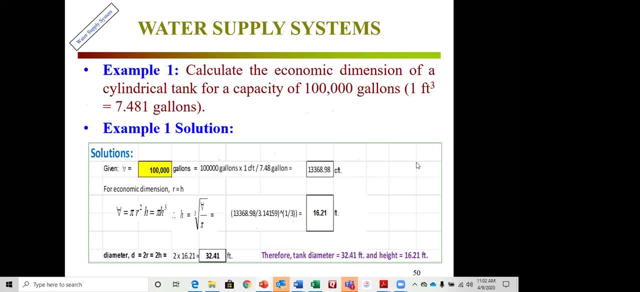 have to use r equal to h. now we know v equal to pi, r square h right by r square h. so if we replace r equal to h or h equal to r, I did here r equal to h, so in this case, v equal to pi, h to the power. 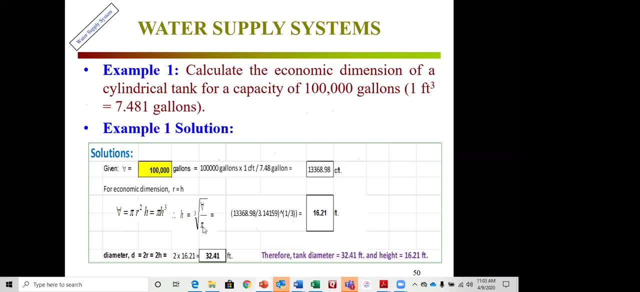 phase. so h, equal to cube, root of volume divided by pi. so you know my case is. the volume was this: h and pi is 3.14159, to the power one third. so I got 16.1 feet, meaning my height or radius is the. 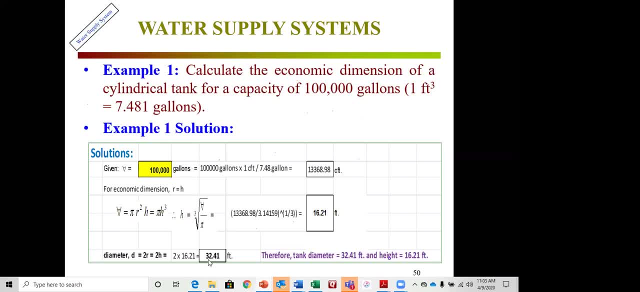 same right would be this: so my diameter has to be double, so it would be 32.41 feet. so my design would be 10: diameter is 32.41 feet and height is 16.21 feet. so this is. I'll keep this problem in a screen. 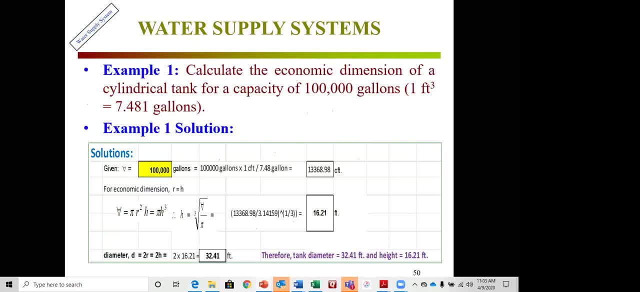 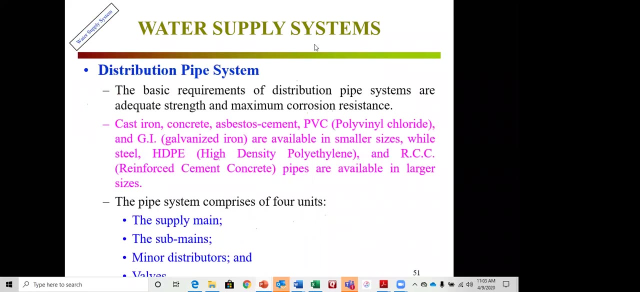 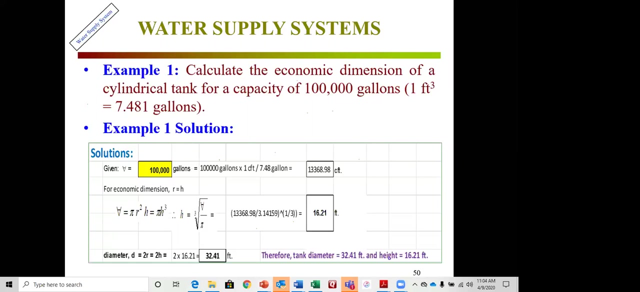 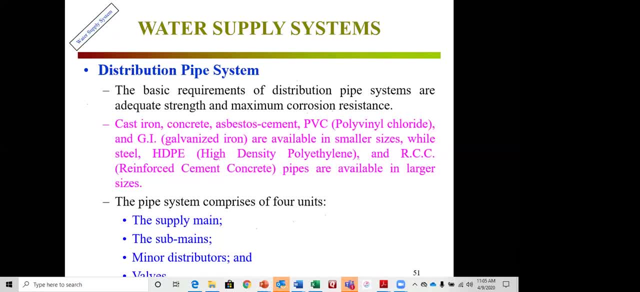 that's what we are going to discuss right now. the basic requirement of distribution pipe systems are adequate strength and maximum pollution resistance. so we need enough strength and it has to be non-corrosive and other things like that: cast iron, concrete, asbestos, cement, PVC and GI galvanized. 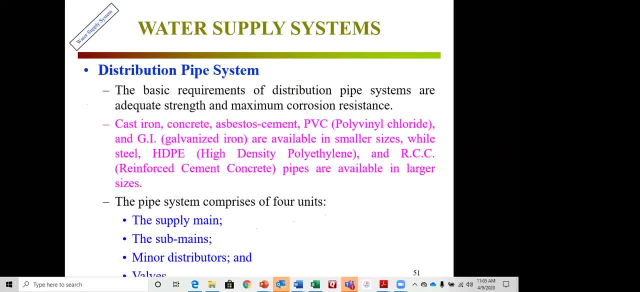 iron are available in smaller size, while the steel, HDPE and the RCC reinforced concrete, cement concrete pipes are available in larger sizes. so these are the one looks like suitable for that. it pipe system comprises of four units: the main supply main, sub main, minor distributors and the bulbs and a pertinence, as we can call it, a pertinences bulbs and a pertinences. so this is. 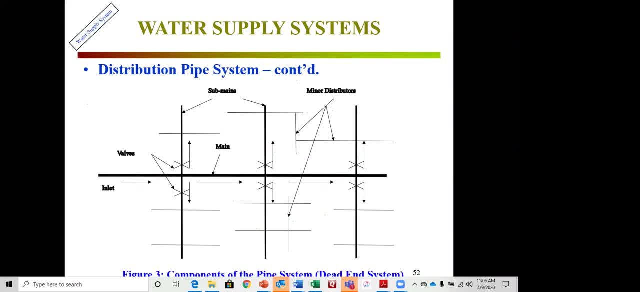 the one typical example that I'm showing here. in this typical example the distribution system is called the data system. so this is the main pipe coming in. we call it main. then there is a branches going a little bit smaller size is called sub main and some of the pipes like coming out of the 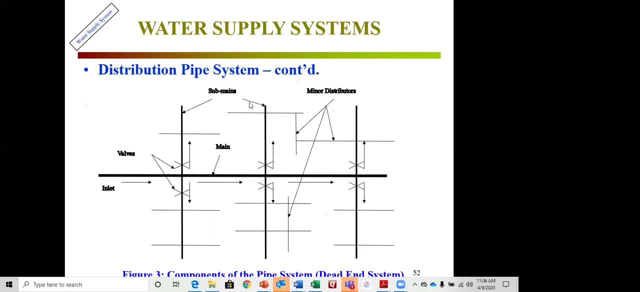 sub main, going left to right or up down, things like that. these are called the, the, the kind of minor distributors. okay, these are kind of minor distributors. these are the part of system, okay, so anything else other than this and this, so rest of them are kind of minor distributors. distribution. 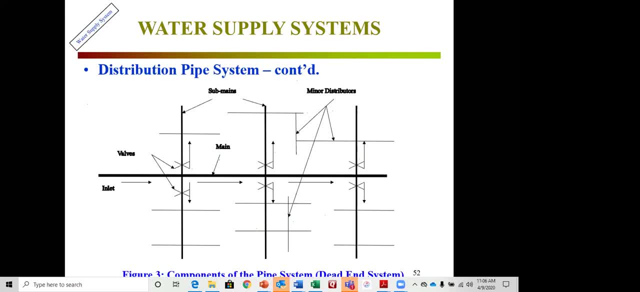 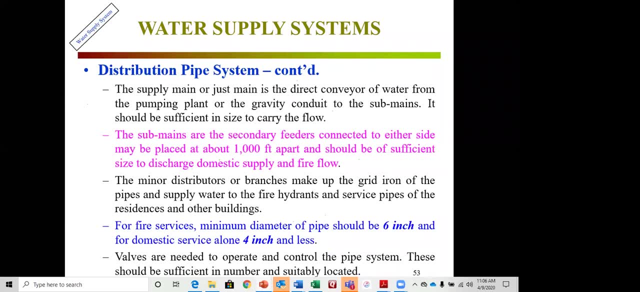 system or distributors, things like that. okay, the supply main, or just the main, is the direct conveyor of water from the pumping plant to, or the gravity conduit to, the sub mains. it should be sufficient in size to carry the flow. whatever the flow you need, the sub mains are secondary. 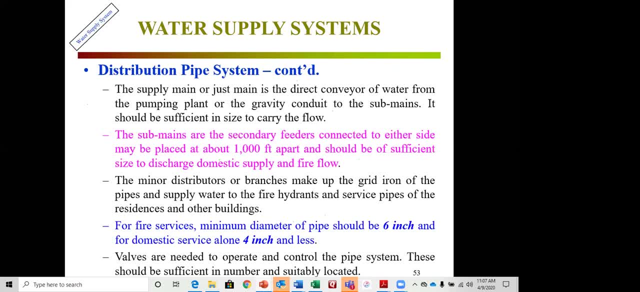 feeder connected to either side may be placed at an one thousand feet apart and should be sufficient size to discharge domestic supply and fire water, things like that. so the, then the minor distributors are the branches coming out of from the sub, sub main and things like that, the fire. 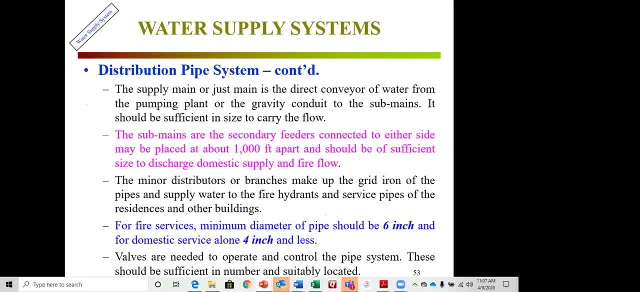 services. minimum diameter is six inch, for that is very domestic area, so in case we can use four inches or less, valves are needed to operate and control the pipe system. this should be sufficient in number and suitable, suitably located so we don't have a lot of losses and other things. 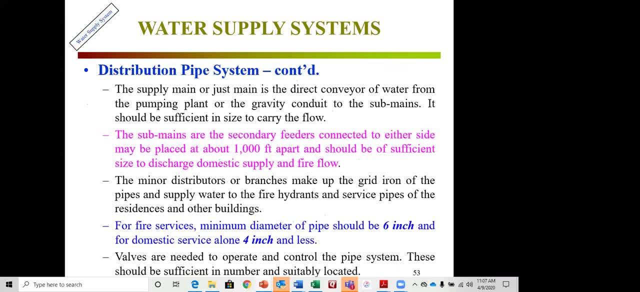 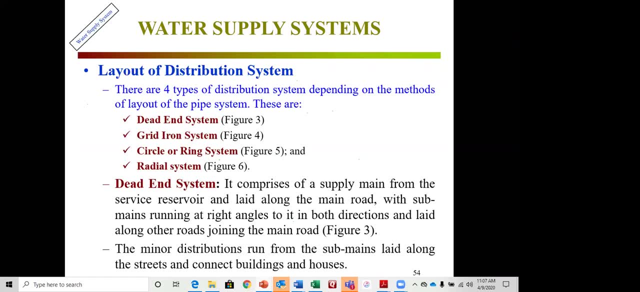 due to those things in there. layout of the distribution system. there are four different layouts of the distribution system, so one is called the dead end that I showed you in the picture three before then. the second one is a grid, iron system, circular room system and the radial system. so dead end system, the figure three. 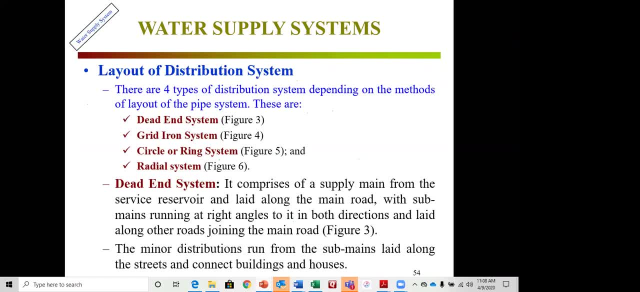 that I showed you already this side are kind of open dead end right. the minor distributor run from the building and connect building and hoses houses in this case. so definitely the the minor distributions are the one that connects to the housing with the houses and other things like that. 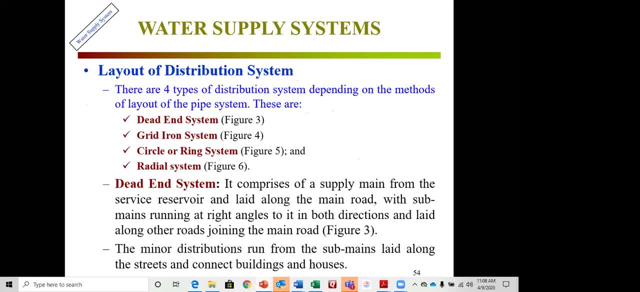 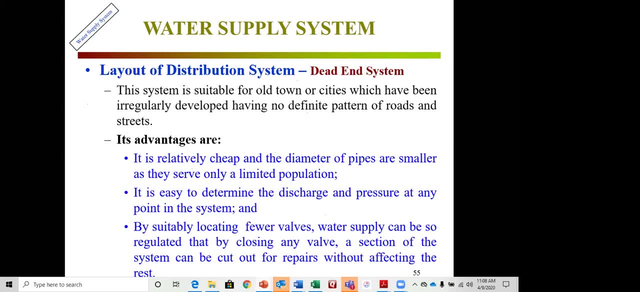 I already showed that one in there in the figure three right. okay, here are some of the advantage for that. this is one of the advantages is kind of uh, relatively cheap and diameter pipes are uh, the diameter pipes are smaller and easy to determine discharge and pressure at any point in the system. or we reconnection to the newer housing near Lucasio is 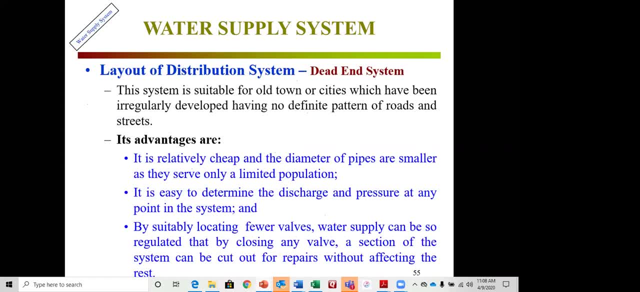 easy, for that is more suitable. by suitably locating pure bulbs, water supply can be so regulated that by closing any valve a section of the system can be cut out, for various appears without affecting the others. that's the main idea of those bulbs and other systems. In This Case, definitely they have some. 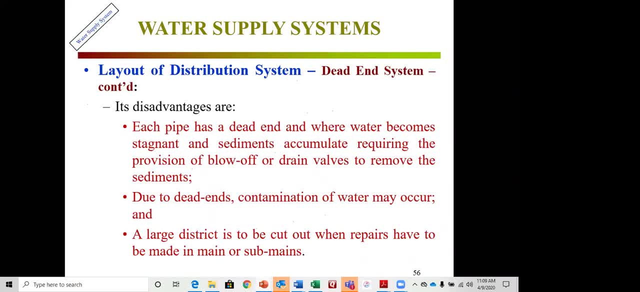 on that too. okay, there are some disadvantage is pipe. each pipe has a dead end so there is a pollution in there. so there could be accumulation of pollution and some of the cases blow out thing. due to dead ends, contamination of water may occur. yeah, large district is to be cut out when? 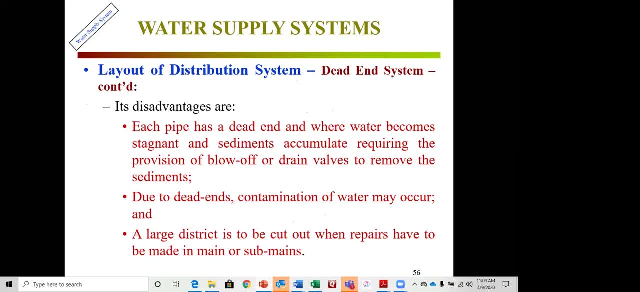 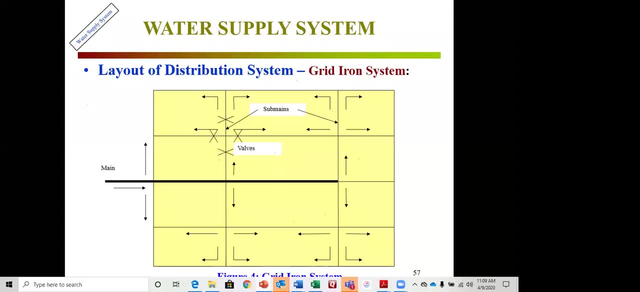 repairs have to be made in a main or sub main. yeah, this is another disadvantage, looks like the next one is the grid iron system. the grid iron system- it looks like I have a main a little bit. a main goes from connect those the the sub mains. then everything is submit as well as it. 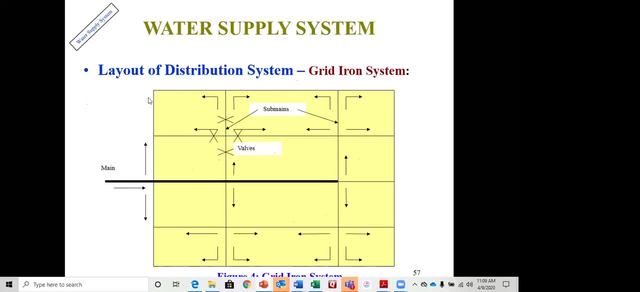 has a surrounding right, it's kind of looping. it's kind of looping, it's a closed loop. other way we can say closed loop: if we don't close all the valves, that means the water can run from this side to this side all the way back here. 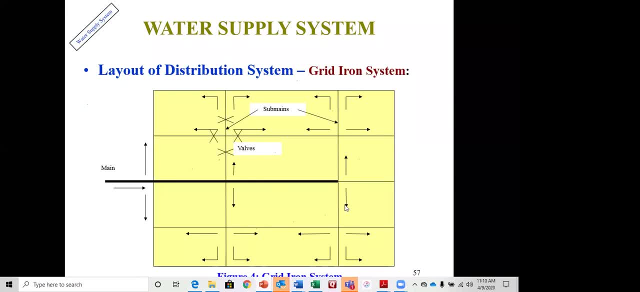 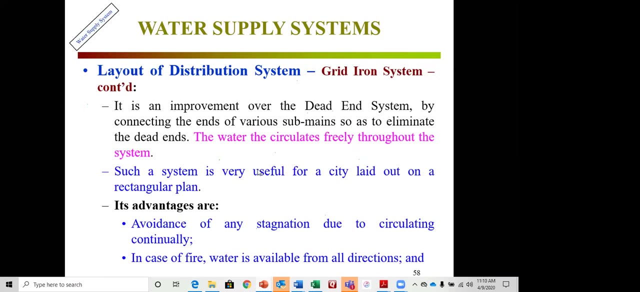 this side, this side, this side, it can run everywhere because it's a grid iron system. okay, so the main advantage of this thing would be the evidence of any stagnation due to circulating continually, because they're circulating around, because they said it's a closed end but open to. 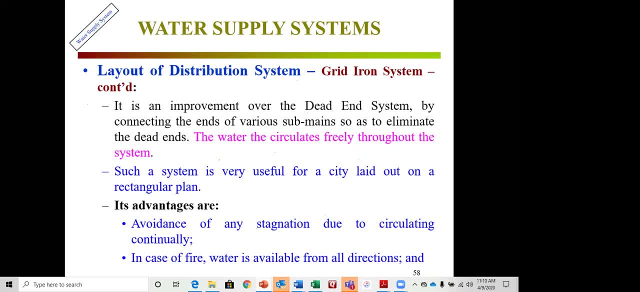 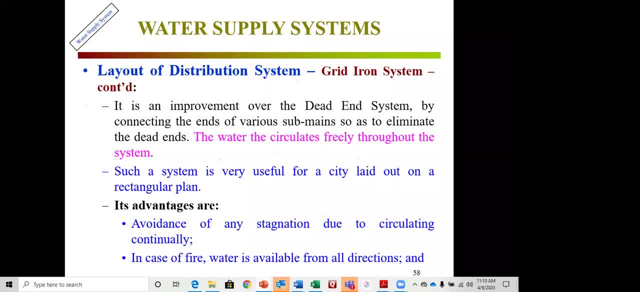 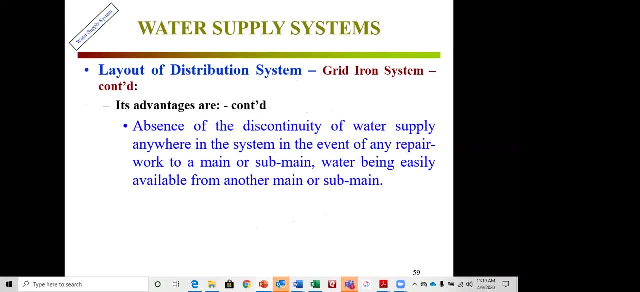 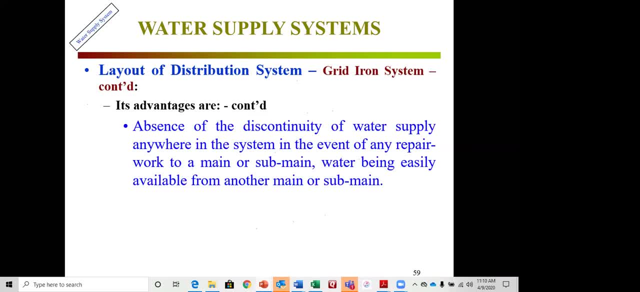 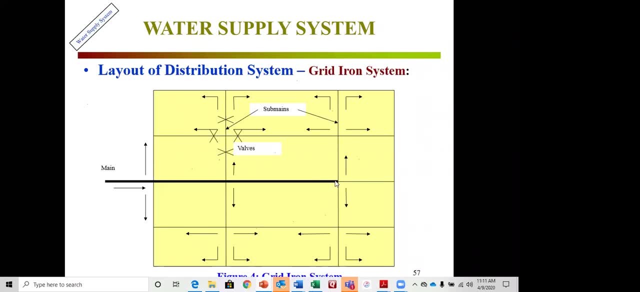 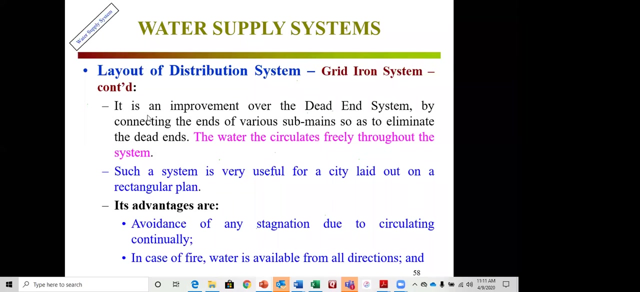 shut off. so that will take advantage, especially the main used to be repaired in this case. if it is to be repaired anywhere here when we have to cut the water here, right? so that means everything. everything will be stopped. yeah, What the disadvantage looks like. 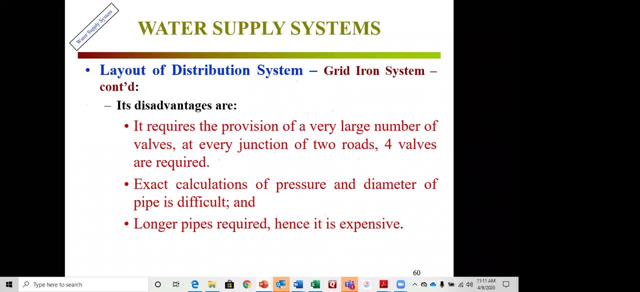 it requires pollution of very large number of valves. at any junction of two roads four valves are required. So exact calculation suppression diameter of the pipe is difficult. Who can use different methodologic to do that right? So longer pipes required. hence it is expensive. 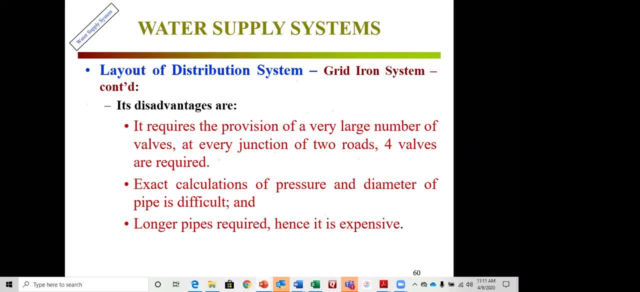 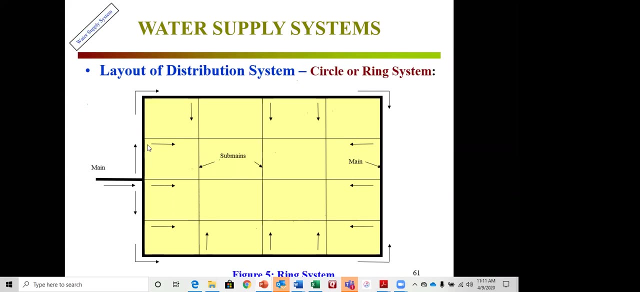 So this is cost is another factor for that In terms of the cost. this is the cost is one of the disadvantage for that for the new iron distribution system. Next one is circular or ring system. That means this is by definition. 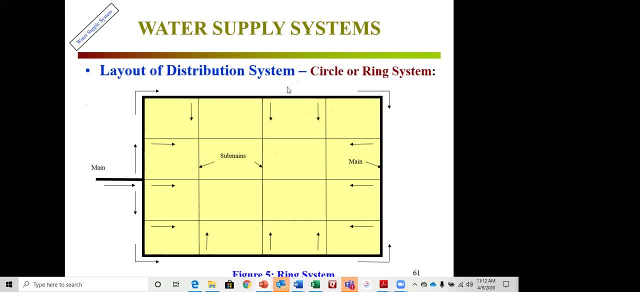 it means, like all the surrounding area has a main and all other sub mains are being fed from the main And throughout the circumference, and other things like that. Okay, so these are the differences. Okay, so let's see some advantage- disadvantage. 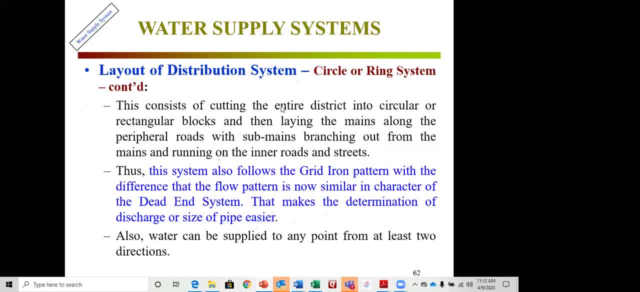 This is a little bit of description of those circular and ring system Cutting edge, cutting the entire district into circular, I think, but this can be a little bit. yeah, It's definitely better than dead-end system makes the determination of discharge. 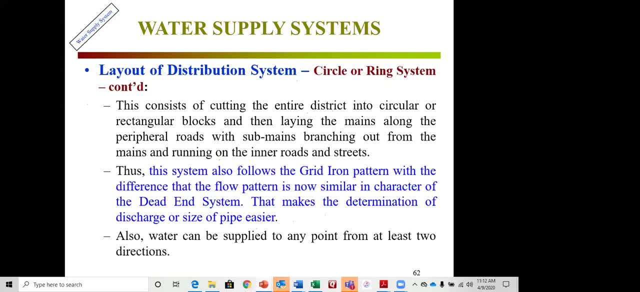 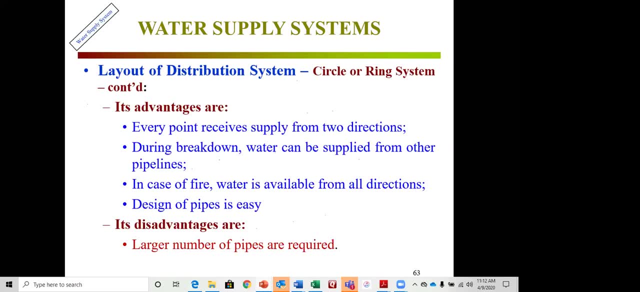 or size of the pipe easier. Water can be supplied to any point from at least two directions. in here The advantage, very point, every point receives supply from two directions. During breakdown water can be supplied from another other pipes. In case of fire, water is available from all directions. 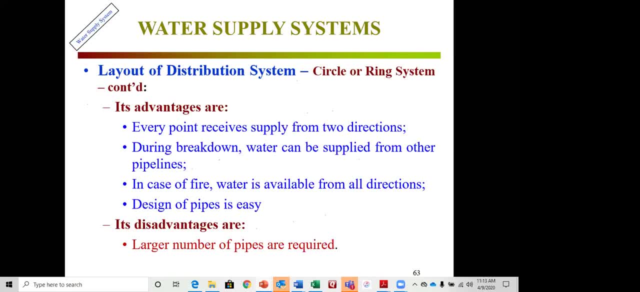 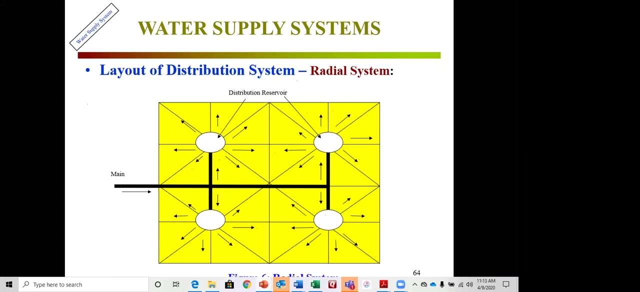 Design pipes is easy And disadvantage is large number of pipes are required, So more length of the pipe. This is the last one. Last one is the radial system. Radial system is a basically closed system, But the only thing difference is, like I said. 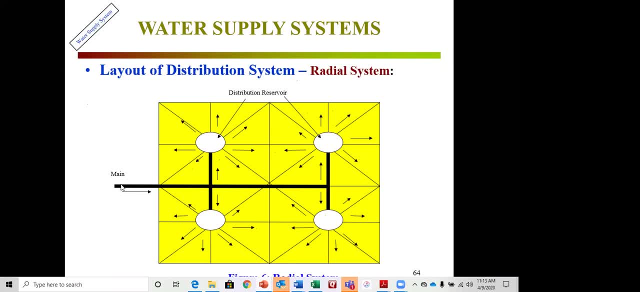 it runs the main from source to the main, other to main, that goes to the reservoir or the tank or the storage tank. So these are the only main And the rest of them are sub-mains. okay, The rest of them are sub-mains. 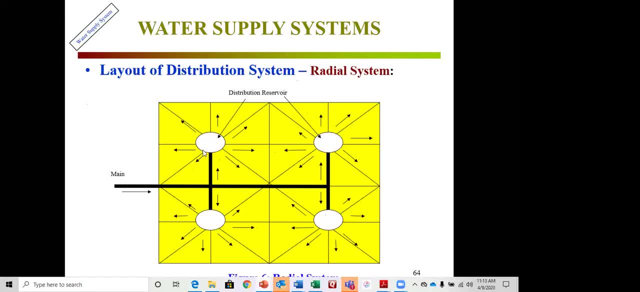 And one of the advantage of those is basically certain areas can get water from different sources, I mean different directions. It's more than two. The one that we saw before was two-direction surface, But this one can be even more than that. 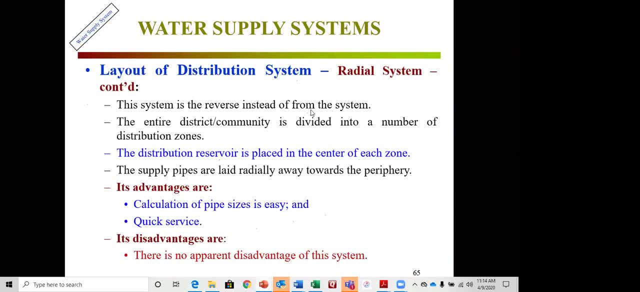 So this is one of the advantage. So there are some of the description of the entire. distribution is divided into number of distribution zone And distribution reservoir is placed in the center of each zone right. The supply pipes are laid radially away towards the 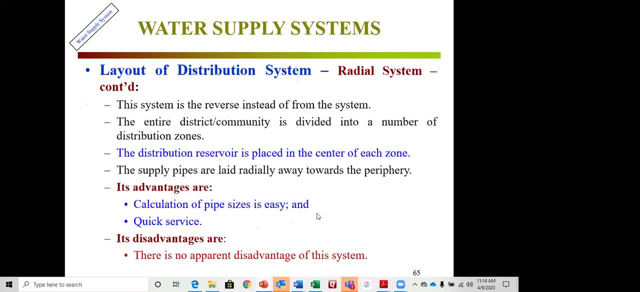 Then its advantages are: the calculation of pipe sizes is easy, quick service. Disadvantage: there is no apparent disadvantage of this system. Means it's expensive. I should say that It would be expensive Because of the design And the pipe system putting together a different way. 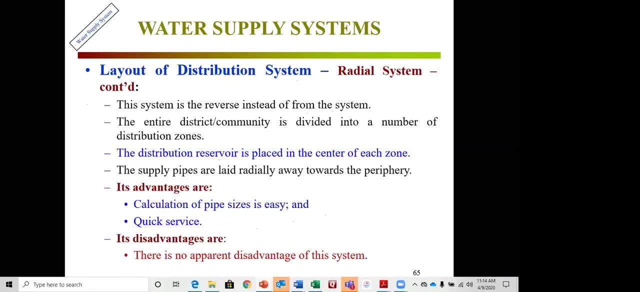 it would be. it will not be cheaper, So it would be expensive, looks like. Okay, So any questions? If you have any questions, you can go ahead and type into the windows In the chat box. So I will go back to that again at some point. 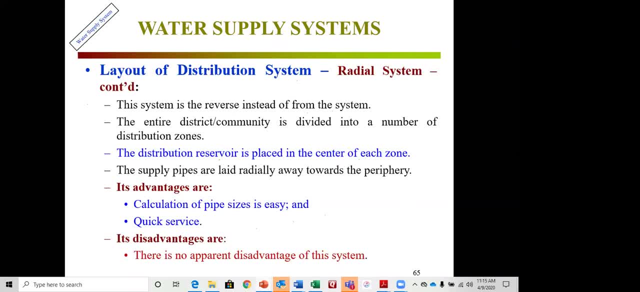 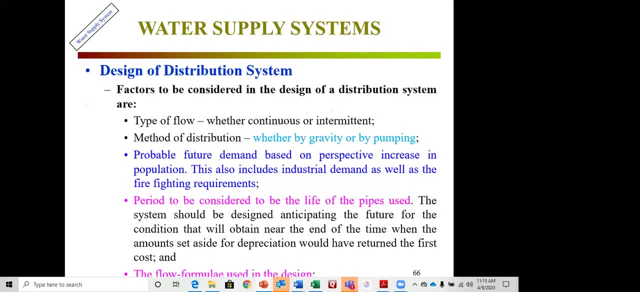 then try to answer from there. Okay, Design of distribution system: How we can design it. In order to design it, we have to consider a few things. Number one: type of flow, Then, whether intermediate or continuous, I think pipe design would be the same. 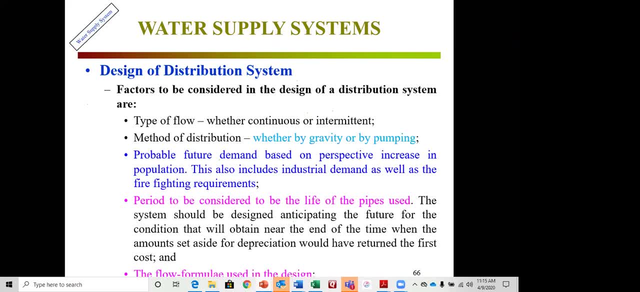 but better to know it Like. so what kind of distribution we have, Either continuous or intermediate. Then the method of distribution: either by gravity, or by gravity and pumping, Or just the pumping and other things like that. So, whether by gravity or pumping, 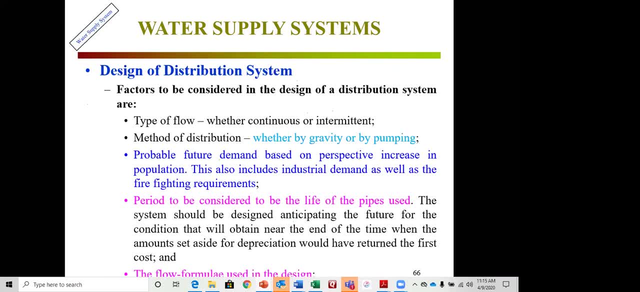 a probable future demand based on perspective increase in population, which also includes industrial demand, as well as the firefighting requirements Period to be considered to be the life of the period I've used, Either 50 years, 40 years or 30 years. 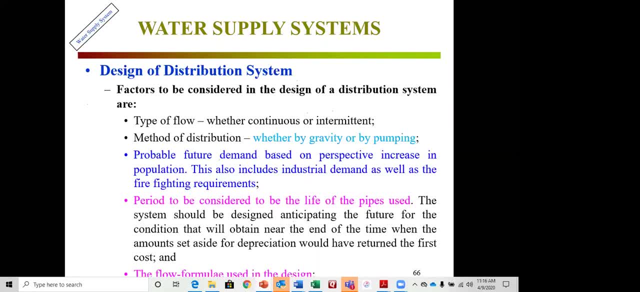 That's what we have to consider. Some of the cases The system should be designed into setting the future for the condition that will obtain near the end of the time when amounts set aside for deposition would have returned the first cost. So these are the one. 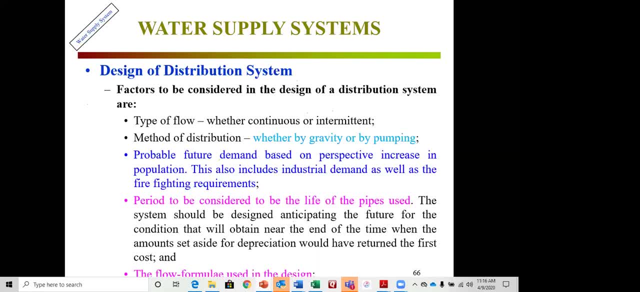 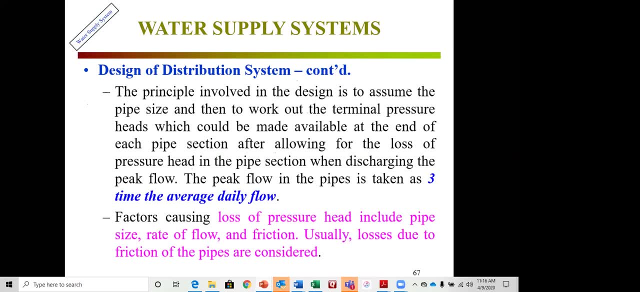 The flow formula used in the design is also another factors to consider. So principle involve the design is to assume the pipe size and then work it out, Or it you can do, assume the velocity. if you know the p keyword You can design it from there too. 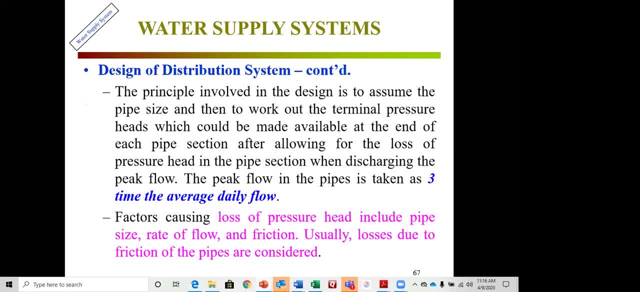 So the peak flow in the pipes is taken as three times of the average daily flow. So most of the time we supply in what it is flow. but this system has to be designed more than that- So peak- if we need to supply water during the peak time. 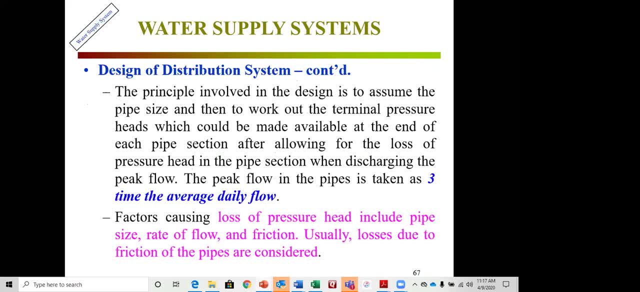 then we may have to have the the capacity of the pipe system for that. so that's why the pipe size you have to design always for the- uh, the peak one. okay, so the factors causing loss of pressure head include pipe size, rate of flow, friction- usually losses due to the friction of the pipes are considered- and the other one. 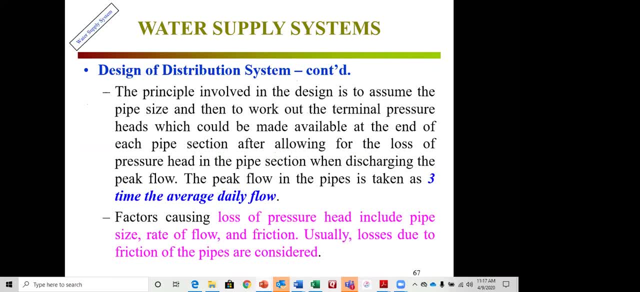 are minor due to the band and contraction and enlargement of the pipe system, connection of the five bulbs in between and so on. if we have anything like that, then i think we should be able to calculate different things. the available pressure heads, as calculated, are checked up to see. 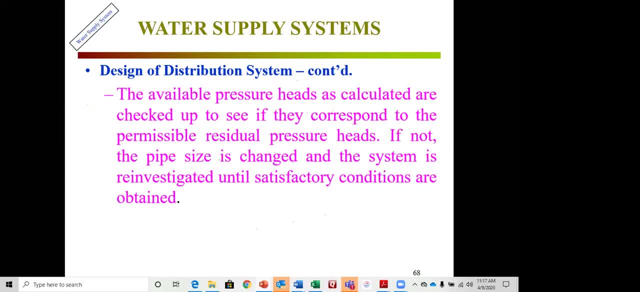 if they correspond to the permissible residential pressure heads. so that's what we are going to calculate in certain areas. if not, the pipe size is changed and the system is reinvestigated until satisfactory conditions are obtained. so it's a way of designing the pipe. uh, the back back calculation. if we consider the 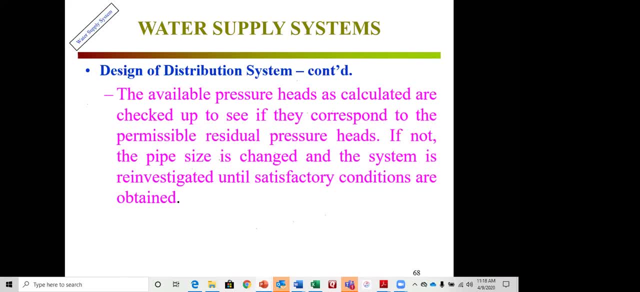 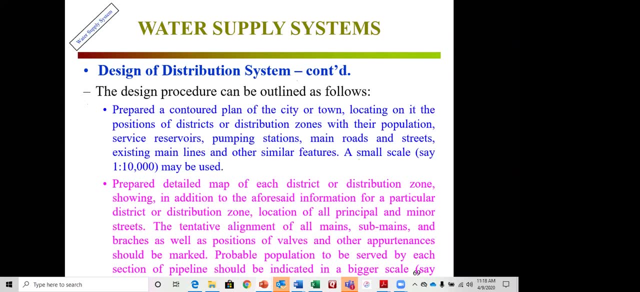 the pressure first, then go back here and then we can do that. okay, so design procedure can be outlined as follows: uh, prepare a control plan, control plan for the city at the town, locating on it the position of district and distribution zones with their population services of wars pumping. 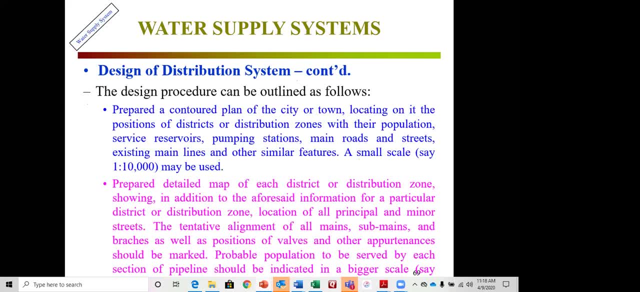 stations, main road streets, existing main lines and other features. a small scale of, say one is to ten thousand uh may be used repair detailed map of each district or distribution zone showing, in addition to the aforementioned effort set in pollution for the particular district decisions, locate all the principal and minor streets. yeah, it's very important because 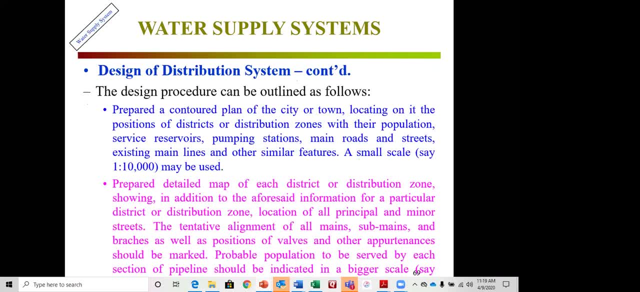 as i mentioned before, if you're bringing the water thing, can you do through the road or you have to bring it like before, that meaning somebody's house may have to be taken right if it is falling within the range of whatever we are trying to do and the water will stop our line pipe in there. 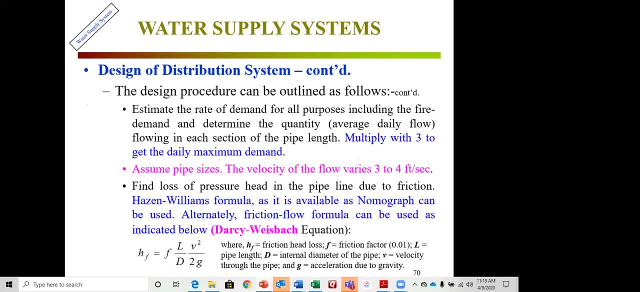 okay, so the estimate, the rate of demand. rate of demand means how much water we need. uh, it's very easy to calculate. if i know of the population in the area, then i can multiply with a certain amount. uh, like say, the water consumption nowadays is almost 100 and 405 on average, gallon per capita. 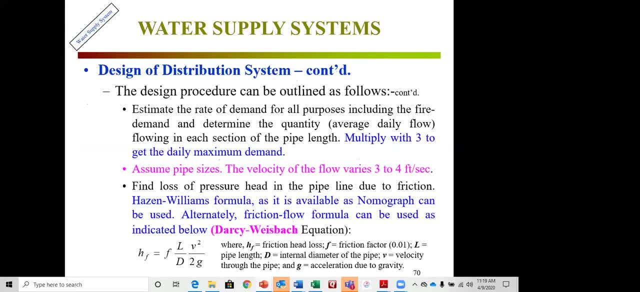 per day. that means 450 around right, 450 liters per capita per day. so then, if we know the average design, they multiply with the three. i can get the daily maximum demand. the same pipe size. the velocity of the flow varies from three to four feet per second. 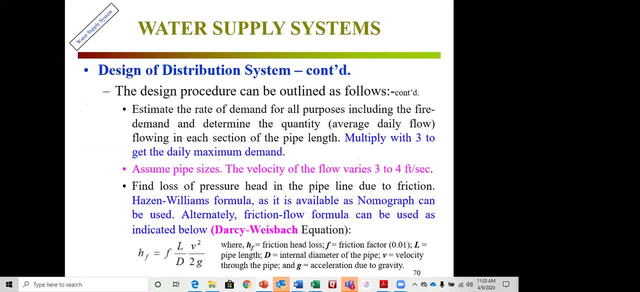 so these are flinging: self-cleaning velocity and subs, non-scouring velocity, things like that find loss of pressure head in the pipeline due to the friction. as in william, formula, as it is available as nomogram, can be used alternative friction law. friction flow formula can be used uh indic as indicated below. that's the way's big equation. 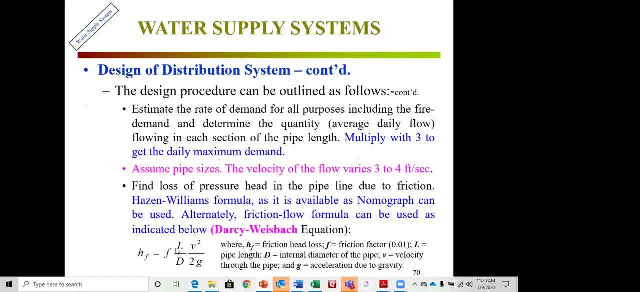 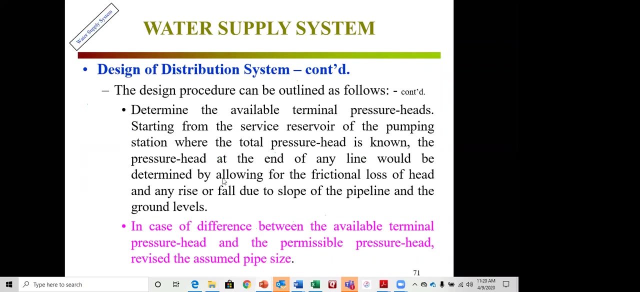 right, good, so this is darcy's big equation. f is the friction law, uh, friction factor that comes out single type of過去, az outer. well, if you take what's called the båth adventure, what's one option of a of platform? uh, е. 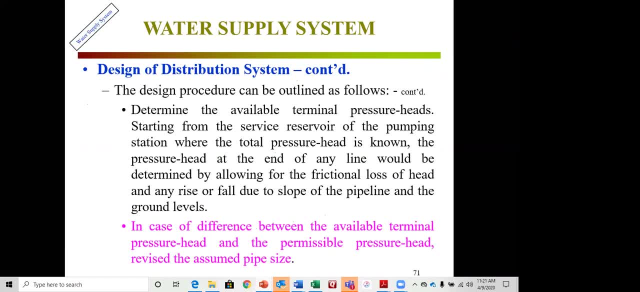 s l pressure head at the end of any line would be determined by, along for the friction loss of it, and any rise or fall due to the slope of the pipeline and in there. so that means whatever is saying there. it is kind of like, say, energy equation. so it's a very linguistic way in case of difference between the. 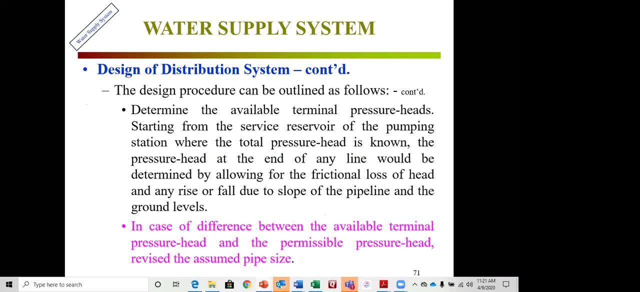 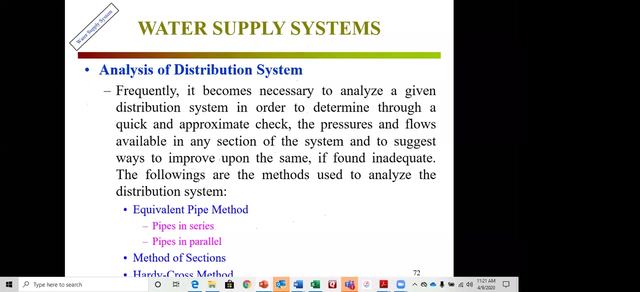 available terminal pressure head and the permissible pressure head device- they assume five sides- don't go more than whatever you need to do, it to cost you more and more because of the pipe size, materials and construction and implementation and maintenance. all of those frequently become the same. to analyze a given distribution system in order to 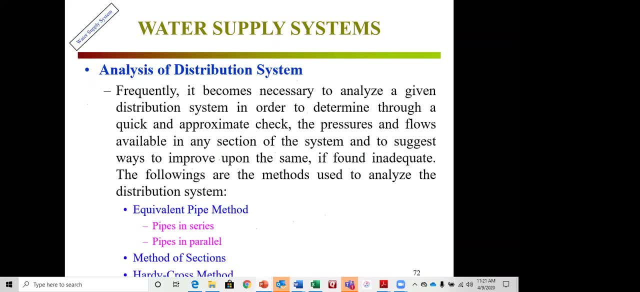 determine, through a quick and approximate check, the pressures and the flows available in any section of the system and to support a sorry suggest wasting through upon the same, if found, and a liquid then. so there can be like kind of improving there. the followings are the methods used to analyze the distribution system. one is equivalent pipe method. 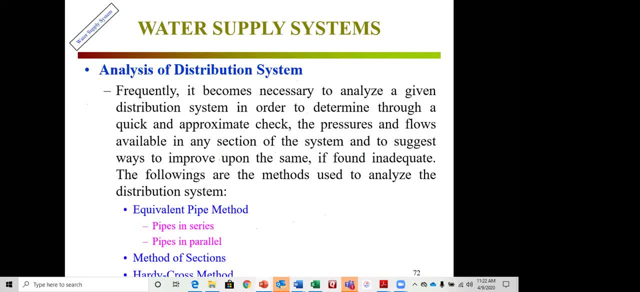 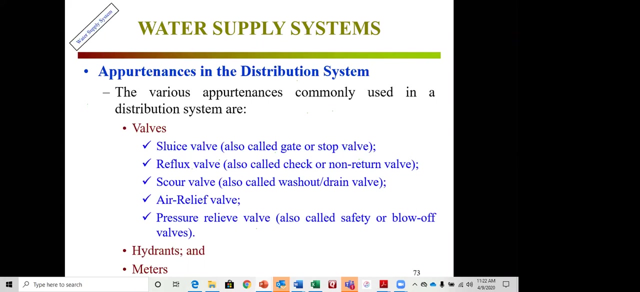 pipes in series pipe and parallel equivalent pipe methods are used. so and then the method of section and the last one is hardly cross. so the method of section and the last one is hardly cross. so the method of section and the last one is hardly cross. so, okay, there are pertinence in the distribution system, different, like say, 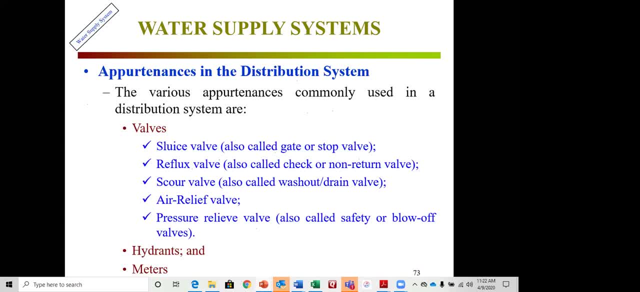 excellent accessories that we might need in there. so is Swiss bulbs also cake, called gate Bob or straw ball, it flags Bob. also called check on non return ball, then scour ball, also called wash I, wash, I, wash I, or what here? are you okay as I after la. 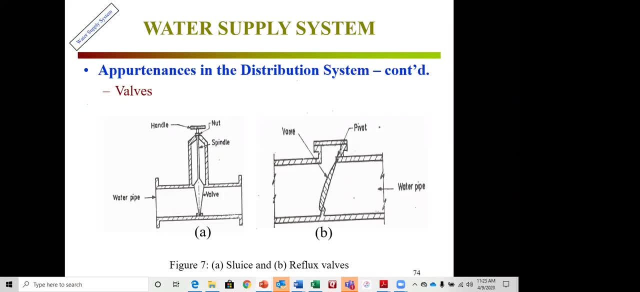 also call safety for blow of. I drew hydrants and the meters agents and the meters reflex valve. So sluice means you can probably turn it around and this can go up and turn off, but it can flow this way, Okay. And B is the, the uh. reflex valve means the water. 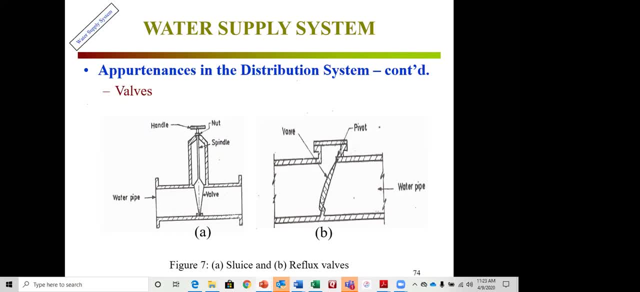 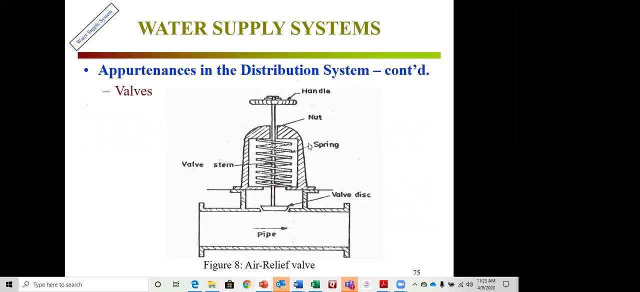 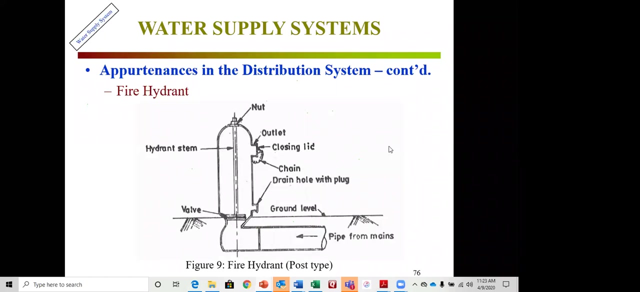 can be allowed to go this way, but it's not allowed that going from this way to this way, Right, So that's what it is. This is the valves that use. the air relief valve means just open it, air reliefs and goes this way and dissipate. This is a spring here And this is the fire. 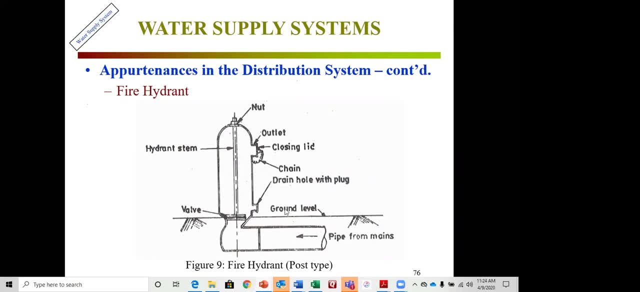 hydrant. The water is coming here and this is the hydrant, this is the ground level and this is the drain hole, with plug and chain and other things, Uh, things like that, And most of the time we had a lot of stuff over here that we could. 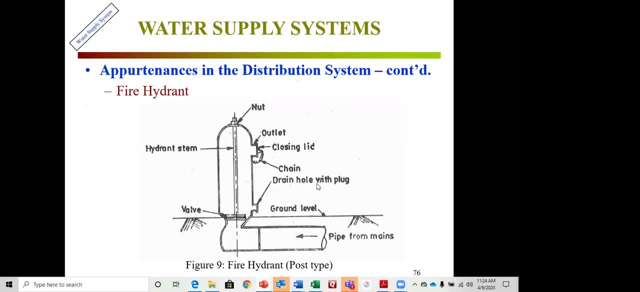 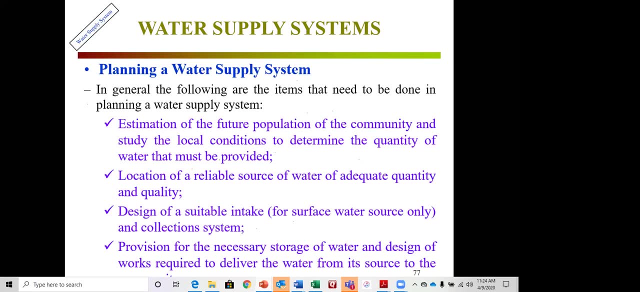 use in there. So then, planning of water supply system. So, in general, the following are the items that need to be done in the planning and order supply system: estimation of the future population of the community and the study local conditions. So estimation, we do a lot of model uh population. 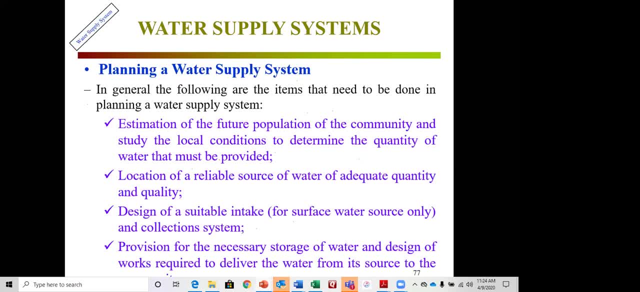 model for population estimation model and other things like that. So it's not a hard job to do. Uh, we have, uh, eight or nine different forms of model that we can use: location of reliable source of water of adequate quantity and quality. So these are the one is part. 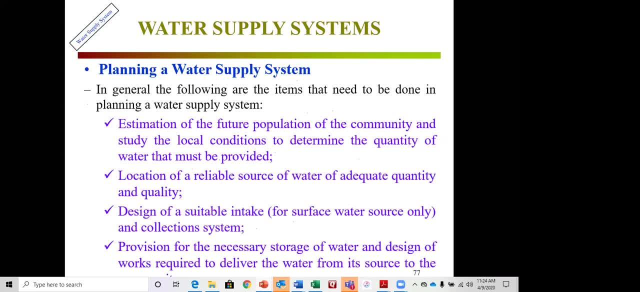 of the planning process: design of suitable intake, uh collection system, uh provision for necessary storage of water, design uh works required to deliver the water from its source to the consumers, and things like that. So we have to have all of those Determination. 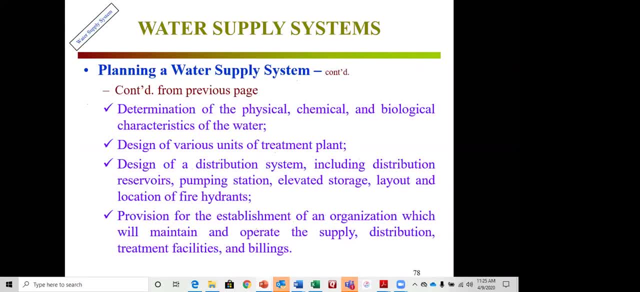 of physical, chemical, biological characteristics of water, the water that you are getting from. So what do we have to do? You have to go to these uh site, uh, grab some sample water, uh water sample and take it under other labs. Then we design those things. Design of various. 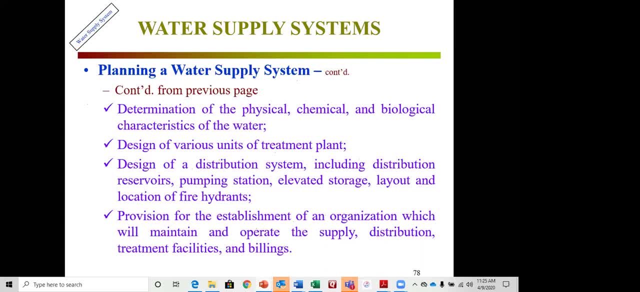 units of treatment plants, In this case treatment plants if we have a complete project, yes, but water supply System, basically uh getting the water, uh getting the water to uh individual housing right, Things like that: Design of distribution system to distribution reservoir pumping station. 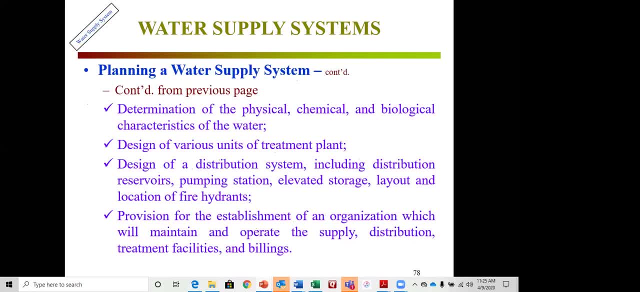 elevator, storage layout and location of fire hydrants. The fire hydrant usually I don't know, It depends on the area and other things. I see some cases every 300 feet, every 400 feet, I don't know. Is there any uh minimum required? I think the different county city. 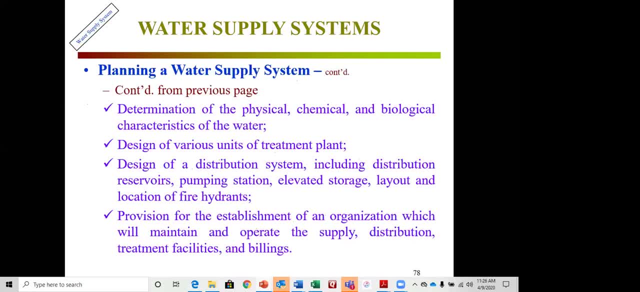 they have their own code To do that. Okay, Fire hydrant provision for the establishment of an organization which will maintain and operate the supply, distribution, treatment facilities and the billing part of it. I think it's always under organization anyway, because somebody has to build a business. 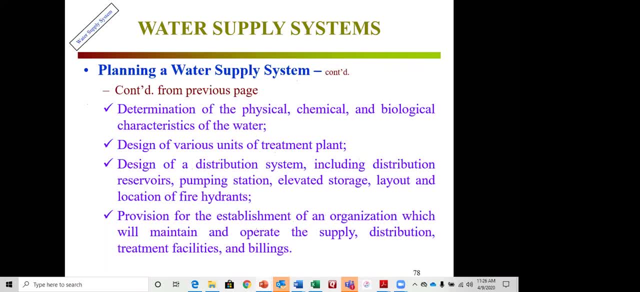 supply it and make money. Okay, To run the business and other things, Okay, Okay, That's a part of the infrastructure, Maybe. Yes, Okay, Before we go to the problem solving, uh, let's go back and see whether we have. 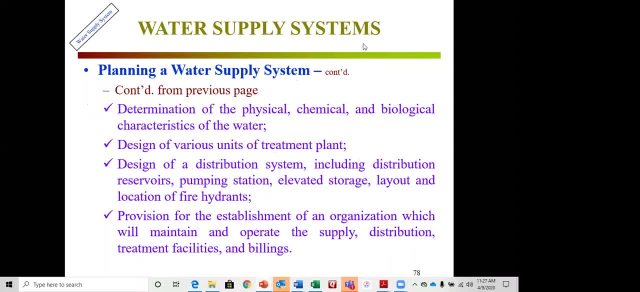 any questions or anything like that? Okay, I don't see any questions. Okay, any questions. We have 30 more minutes, so I think we have a few more problems to solve. then probably we can go and discuss a few more. I will take another 15. 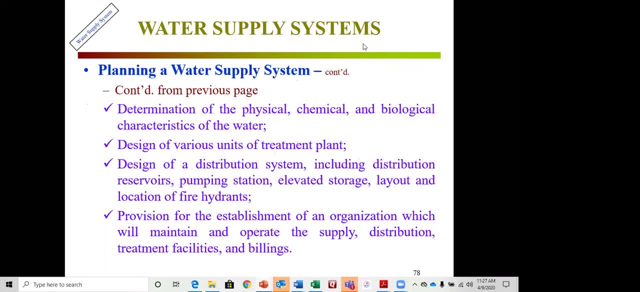 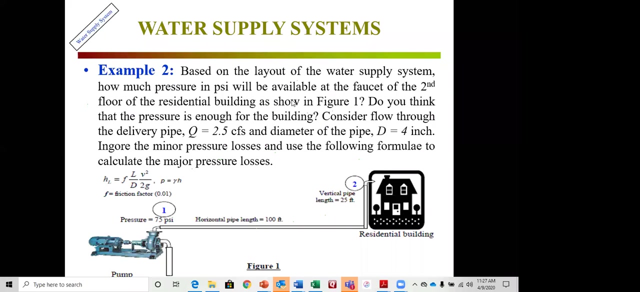 minutes or so. then from there, we'll start a discussion and question and answer session. Hopefully, at that time, you should be able to speak out on that. Okay, this is one of the problem that we'll be solving using the energy equation that I mentioned, So I'll keep this one into the screen for a minute or. 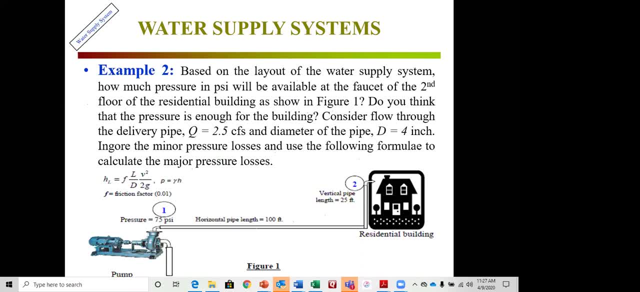 so so you guys can read it and see whether you understand that, Then I'm going to read it again and explain it and then we'll try to solve the problem, you? Okay? let us read this: Based on the layout of the water supply system as: 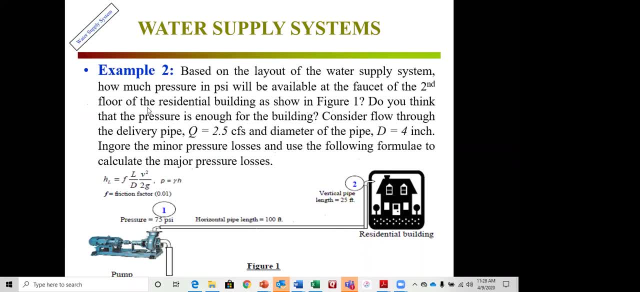 shown in the figure. I mean this is the figure- how much pressure in psi will be available at the facet of the second floor of the residential building. So that means here: Do you think that the pressure is enough for the building? Whenever I say enough means, is it within 50 to 60 psi, that 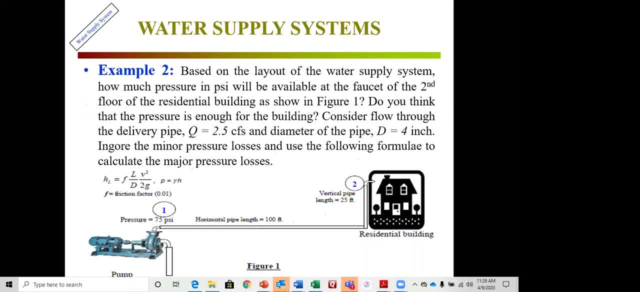 we have seen before right recommended pressure. So recommended pressure was 50 to 60 psi. So in this case definitely is it there, Things like that? Okay, so consider flow through the delivery pipe: q equal to 2.5 CFs cubic feet per second. 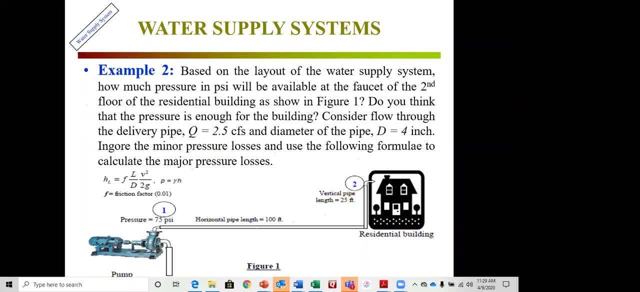 So that means the flow rate that we need to supply into, that is, from here to here, is 2.5.. five cubic feet per second. the diameter of the pipe is four inches right, four inch, starting from here to here, four inch. ignore the minor pressure losses and use the following formula to calculate: 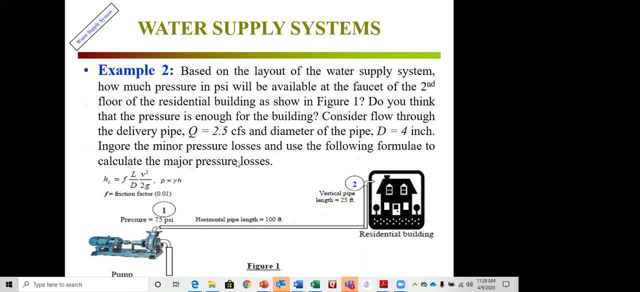 the major pressure loss. okay, the major pressure loss, so minor, would be here. we have a 90 degree bend over here, so there would be a minor here, right? so definitely there would be a minor over here, okay, uh, over here too. so this would be the minor, right. the major loss would be from here to 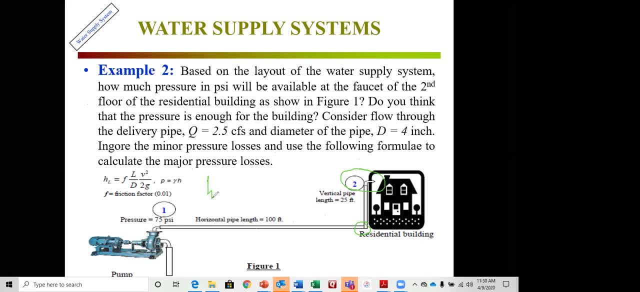 starting from here. so the total head loss. total head loss is equal to friction. this is for the friction and this is for, like say, minor. oh sorry, so we are ignoring this one. okay, we are ignoring this. so in this case, uh, and the way that we do this one, this one is summation of k, then then v square by 2g. so this is the formula we use. 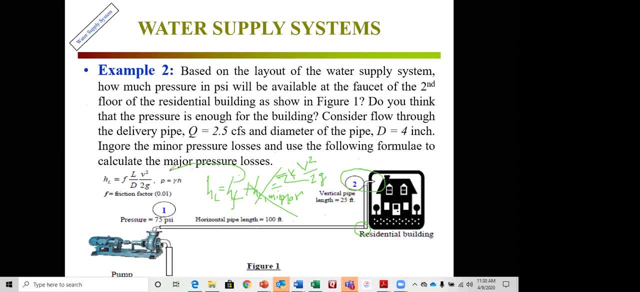 for calculating the minor loss, and this is this equation. we use this equation to calculate that. let's explain the term now. here the f is the friction factor, uh and l is the length of the pipe. in in this problem will be like, say, from here to here, 100 feet, 100, please, plus 25 would be 225 feet. right for the l diameter. 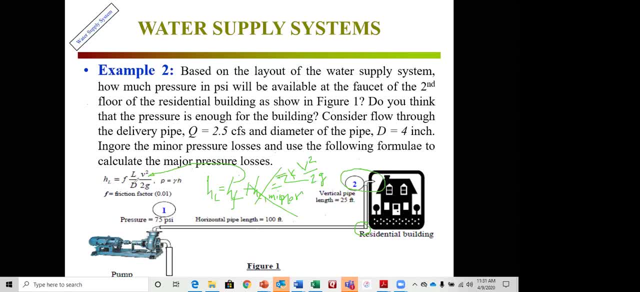 would be uh, in fit, because this is in fit, it has to be in feet also. so four inch four by twelve, four by twelve would be equal to what one third right point three, three uh feet would be here. then v would be the velocity of the flow. 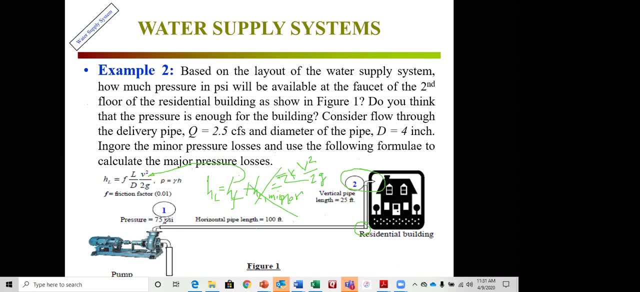 velocity of the flow, since, uh, we are not like changing the diameter of the pipe, velocity of the pipe over here. so at the v1 and here it would be the v2 and both of them would be equal. so we can say v equal to v1 plus v2. sorry, equal to v1, equal to v2, so that means v equal to v1. 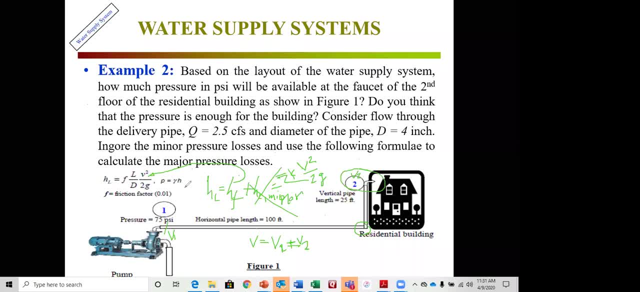 equal to v2. so we can just consider one velocity and we know g. this is the equation i think. i use it to show you how much height you need to come up with the pressure of 50 psi. we come up with 115 without the loss, right? so we could consider the, the loss of the, the friction loss calculated. 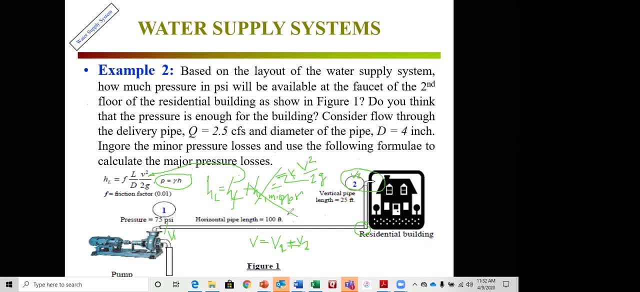 using the equation, then definitely we should be able to go from there in this problem. the friction factor is given, so we don't need to find it. for example, if the f is not given, then we should be able to get it from the moody's diagram. so if i, if i get it from the moody's diagram, i'm going to. 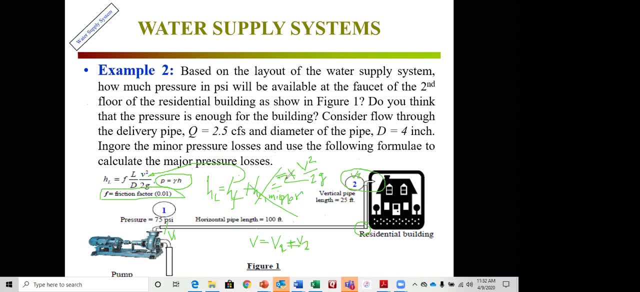 have a time i'll show you how to use it. okay, how to use it in there, uh like say, but if it is given, or certain cases, even, um, what is called the manufacturer, give it to you, the pipe manufacturer, because they know their undulation and other things like that. so we need few things to do that. 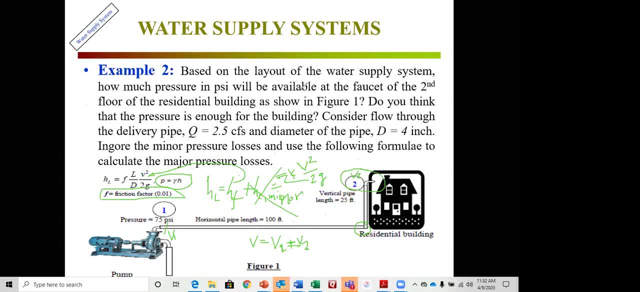 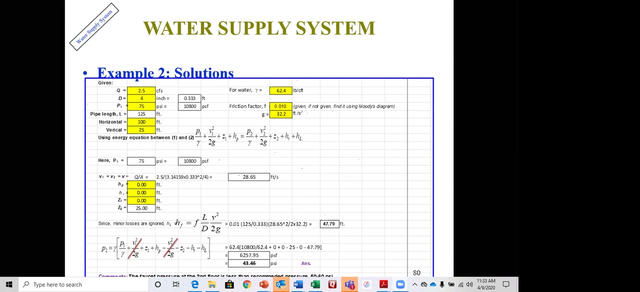 we'll show you later. I don't know, this system is not a good. it doesn't stay with this slide, so i have to see what are the other way i can. i can do things like that, okay, so here is the problem solution. i use excel to solve the problem, but anyway, i'll show you the. i just 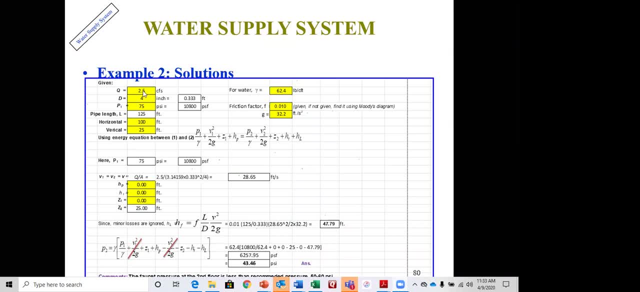 list all the values that are given. okay, q equal to 2.5 cubic feet per second diameter of the pipe is four inches equal to 0.3 cubic feet. p1 pressure at the the source, so let's go back here. it is 75 psi. we already know that. 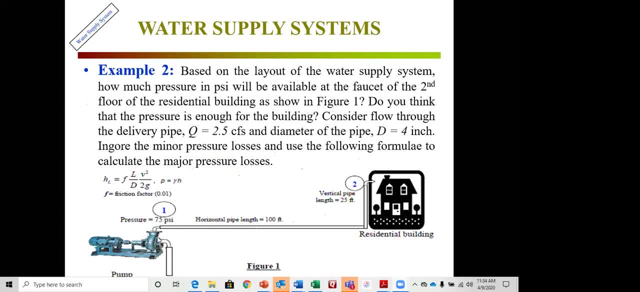 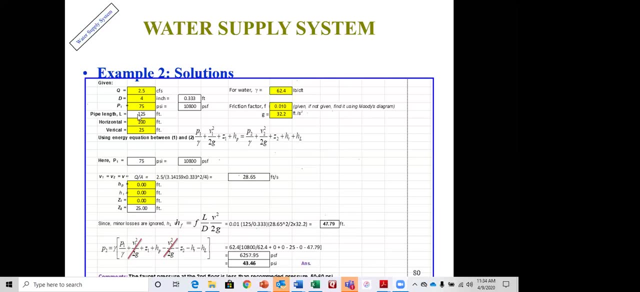 means the pump that will create pump head. so if i know my pump head, how much head this will provide, then uh, like say i can create h times gamma will give me the psi. so that means that's how i know it, right. okay, then the total length of the pipe: 100 is the horizontal, 25 is the vertical, total is 25. 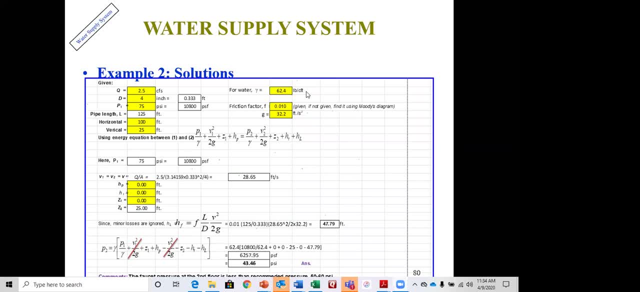 and the gamma of the water is 62.4 pound per cubic feet. friction factor f equal to 0.01 is already given- uh, if not given, find it using the moody's diagram- and g equal to 32.2 feet per second square. 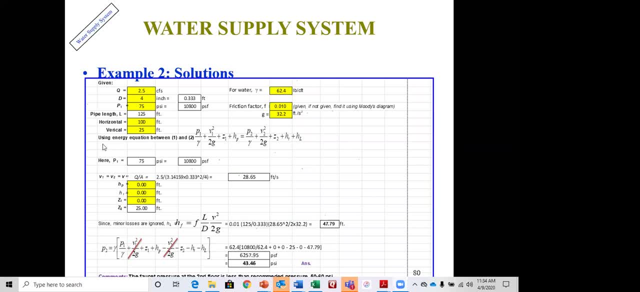 okay, now here is the energy equation between point one and two, energy equation between one and two p, one over gamma plus v, one squared by two z, two g plus z. one plus h, p equal to p to the power of zero, equal to p. two uh over gamma v, two squared by two g, then z, two plus h, t plus h l. so in this problem, 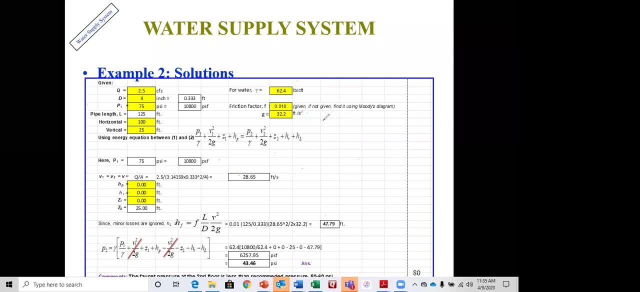 let's see a little bit, uh, if we can draw something here. so, between these two lines: right, i had here, then going to the houses. this is point one and this is point two. so we'll put a datum line over here. this is my datum. okay, so this is my datum. if this is the case, like saying here, let's explain the term. the p1 is the. 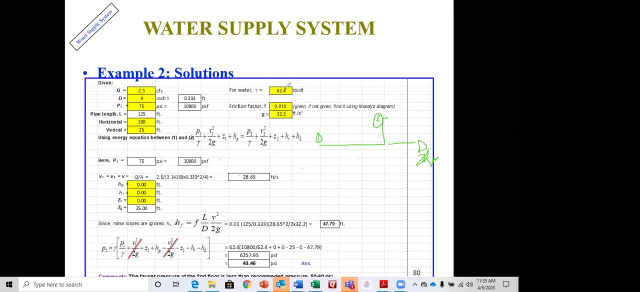 pressure at 0.1 gamma is the unit weight of the water. you know that. then v1 square b, v1 is the velocity of here, at 0.1 velocity of the flow. h1, z1 is the elevation from a certain point. if i consider this one a datum, then this would be my z1 and the this one would be my z2. 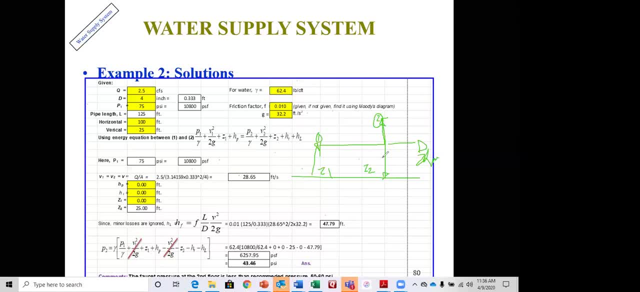 okay, so that's the, the z1 and hb. if i have a pump in between the two lines, say for example here and here, then i'll have- uh, i know that- how much pump head would be necessary? or providing it pump provides the boost the pressure in here. increase the pressure pump. that's the main purpose of pump. 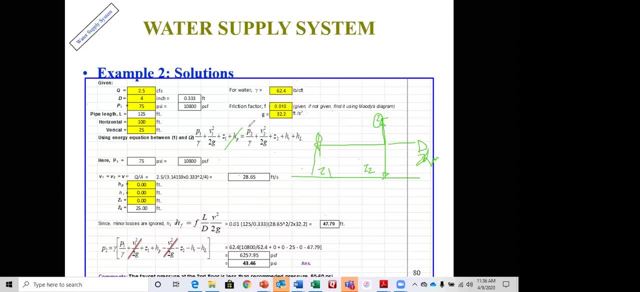 we don't have any right. so in between this, i don't see any in there. so then, uh, p2 is the z1 is the pressure at 0.2. that means that's what we are looking for, that's the problem was asking to do. and v2 is the velocity of the flow over here and z2 is the elevation from here to here and ht. 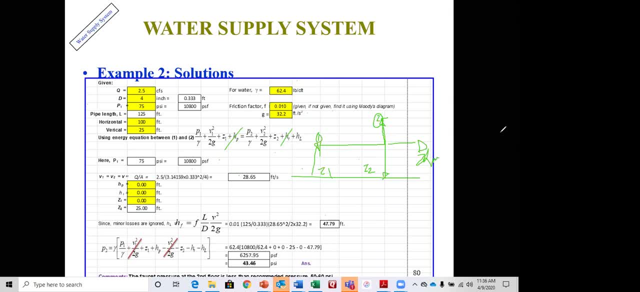 is a turbine. do we see any turbine between? turbine means that takes the pressure or the water flow and creates the energy, generate the energy. so this is the turbine. we don't have any turbine either there, right? so that means this is uh cancel. cancel means this is zero. it's not a canceling out to each other, this is zero. 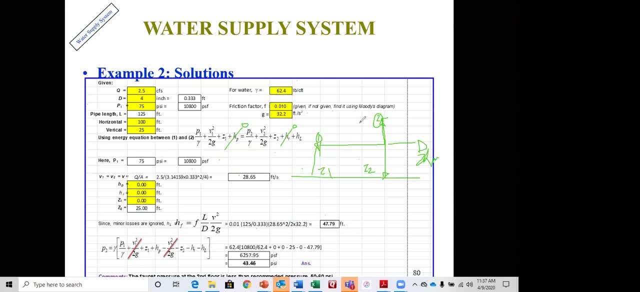 then hl. so hl definite is there. now we are going to calculate the hl. hl, since we are uh, minor losses are ignored, so hl would be hf. that i showed you before. so f into l by dv square by 2g. f is given 0.01, l is 125 over 0.33 d then multiplied over v square v. how we calculate the v: 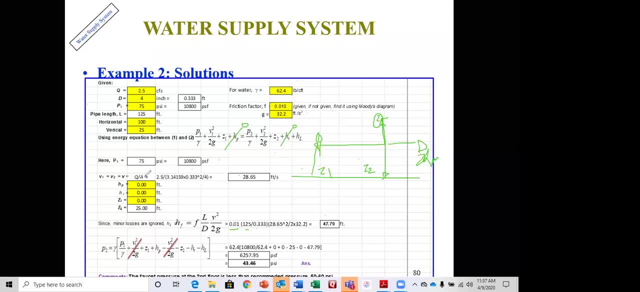 v1 equal to v2. equal to v2. equal to v. q over a. q is 2.5 feet per second. a is pi d squared by 4. okay, or yeah, pi d squared by 4.. this is pi. this is d squared by 4.. i got 28.65. 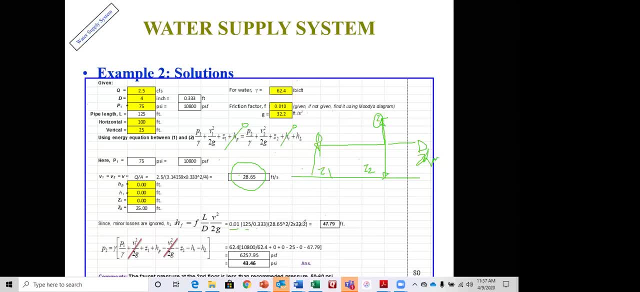 so that's what i put it in here. the velocity square, uh, divided by 2g, so i got 70, sorry, 48 feet, almost close to 48 feet, of the fish loss, head loss loss, mainly. so then, once i put this one into this equation, into this equation, so you see the other, 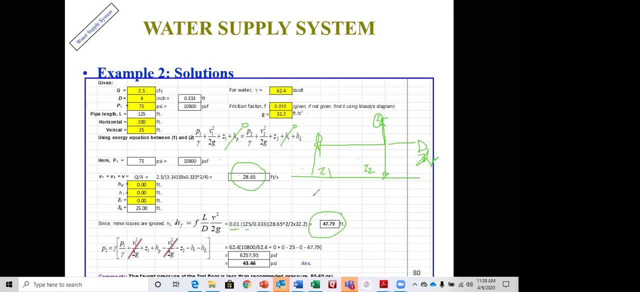 two terms already. i cut it right. other two terms already, i cut it, but still, i may have it here, but it could be. uh, i have it here, but i can put zeros in there. so if i rearrange this equation for p2, that's what it becomes. gamma, then p1 over gamma, v1 squared by 2g, v2 squared by 2: these are minus. 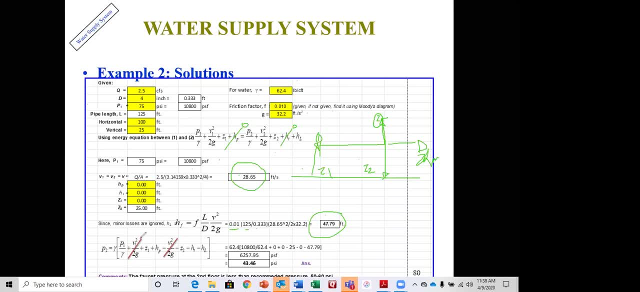 okay, and this is plus, this is minus, since b1 equal to b2. they are canceling out and this is also gone. this is also gone. zero, right, this is zero, zero. and this one would be what? uh, we have it already: ten thousand eight, eight hundred, ten thousand eight hundred, right, and z one would be equal to what z one. 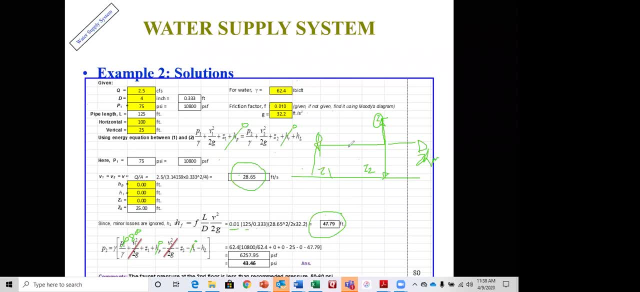 in this case, uh z one would be equal to zero if we consider the datum over here. z one equal to zero, equal to zero, okay, and this, this one is basically: uh hp, equal to zero, right then? negative v square is not there. the negative z2. negative z2 is 25, because this was 25 right from here to here was 25. 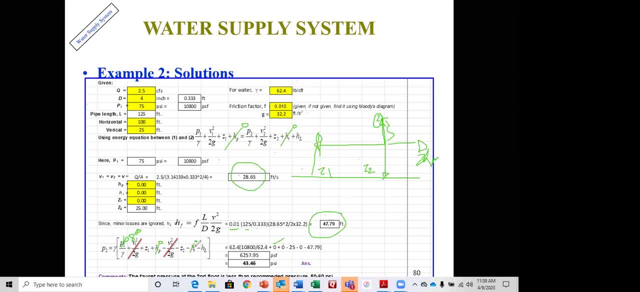 then minus uh, again this one hd, a turbine head, equal to zero, then h, l, hl is the same as the hf, so we get 47.49. so if i do the calculation i got uh 62, 57, 58 fps almost, and then 43.46 is the psi, my pressure. 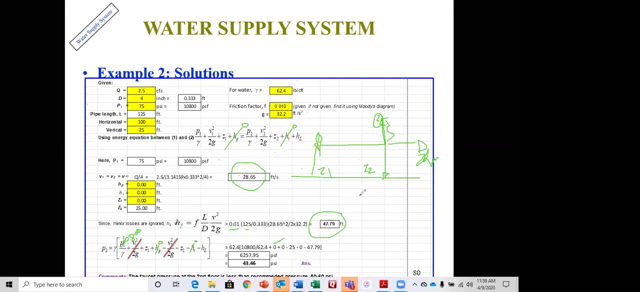 at the house in the second floor, facet is 43 psi around, so our this one is kind of good calculation. only thing is we missed the minor loss. minor loss could be another, uh, maybe 0.5 feet to one feet in here. so that means it will give me a little less pressure here because it's subtracting right. 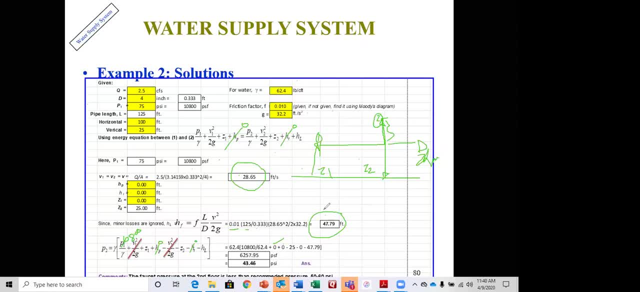 so little less pressure here. okay, then they have a comment here. the the facet uh pressure at the second floor is less than the recommended pressure, 50 to 60 psi. so this is my answer. so that is the case. i'll keep it in a screen for a minute or so. i don't have a lot of time, looks like. 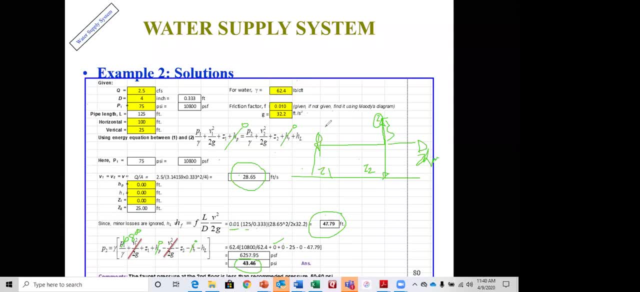 it is a pretty good answer, just a good one. uh, so that's when we get a model of the shorter length so you can see on the screen it's not the shortest length, it's still a 형tso. so this is the length of the third layer per unit, and this is the length that's going to be the length of the other two layers right here. so this is this is the length that the other two layers are going to have. is. this is a becomes a 삼 информ max, like we were talking about. so that means that when you take a plus number, you're going to put a minus at the first line of the spirit, at the end of the second line, of the second line, of the second layer, and then when you put a minus in the second line, you're going to get the negative gradient and the negativeて, or we're going to be a minus in the negative gradient as well. so this is a not a positive thing. we're just going to have to change that point until we're able to make this point in the next two lines. 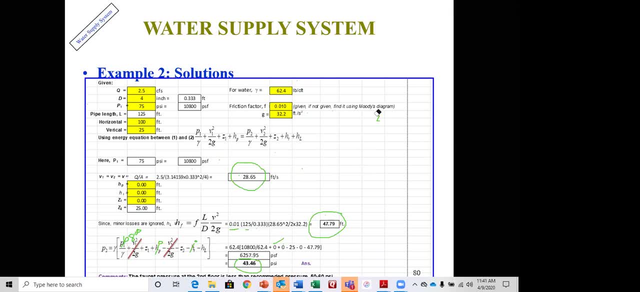 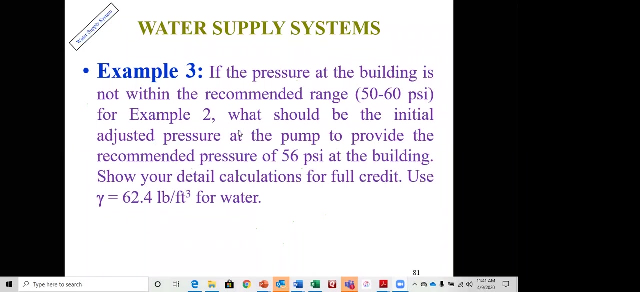 okay, very good. so then let's move forward. this is my next problem: if the pressure at the building is not within the recommended range, that is true now in the example 2. what should be the initial is just pressure at the pump to provide the recommended pressure of. 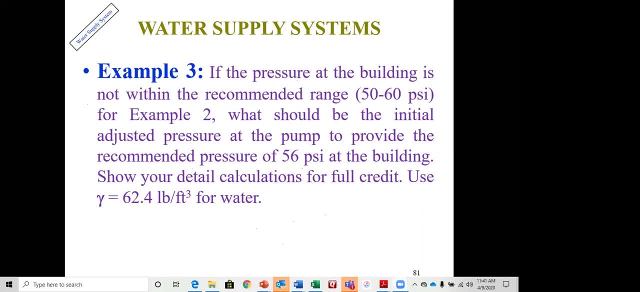 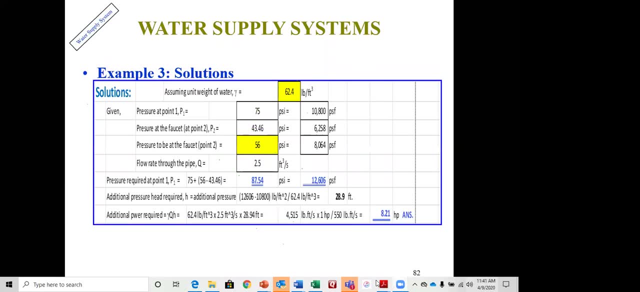 56 psi at the building, so it was 43. now we are, we would like to provide 56 in the building. show you detail calculations? okay in there. so here is the one. I again I use the Excel to do it. gamma is there, p1 is. 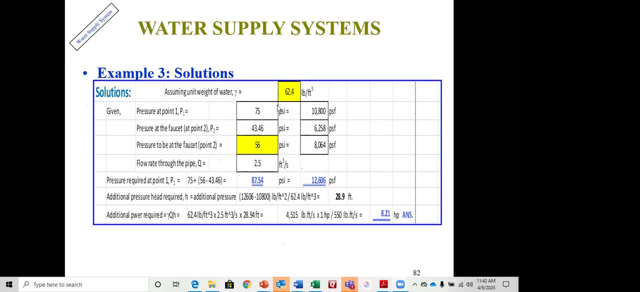 75 in here, but in this case is given to us. that means that means PSI, PSF. already we know at p2, based on the arrangement, this 75, we get 43 psi, 50, 60 to 58 PSF into the facet. what we are looking for now. we would like to provide the pressure at 56. 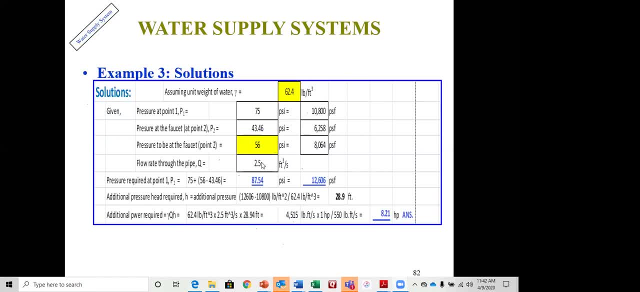 not 43. okay, so then Q is this? so what kind of additional pressure we might need, right, or pump house or anything. so pressure required at the point one. 75 was the year, but it was shortage. how much roadage was there if the six minus forty three? so ultimately that much. 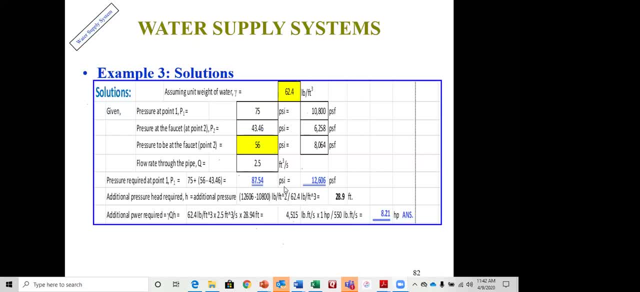 right, we totally need 87 PSI. so that means 12,000, six or six PSF, so additional pressure here that we need. that means that just the differences, right, difference班- this minus this, ultimately we can say this minus this and the same kind of. same thing. moving the tip of the head is done right. we can at least have those real numbers and two engineers working with this plan. so this of course you require that information if we have to move the bed into action. we need utilities. we just added more of my cap because we do not have that much space to convert. 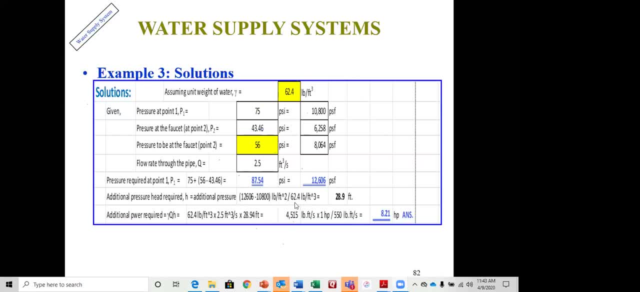 is the same, right. so uh then uh, we do the additional pressure. uh equal to uh, this 28.9 means 29 feet, almost. then we can use the power equation: gamma, qh is the power, uh, 62.4 then 2.5, then h is this? so ultimately we got 45, 15 pound per feet per second, then one horsepower equal to. 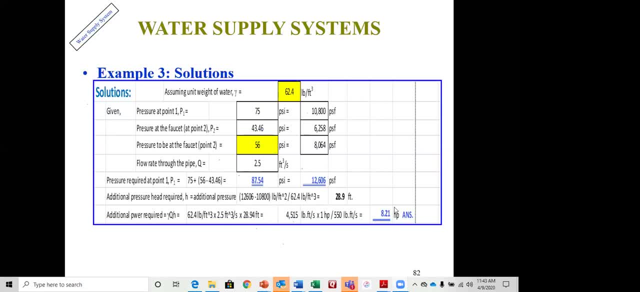 550 pound feet per second. so if you do the math, we get uh 8.21 horsepower. so meaning 821, 8.21 horsepower, we need additional, okay, and total horsepower would be one. uh like say, if we do the calculation based on the total height, uh, total pressure, then definitely would be there. 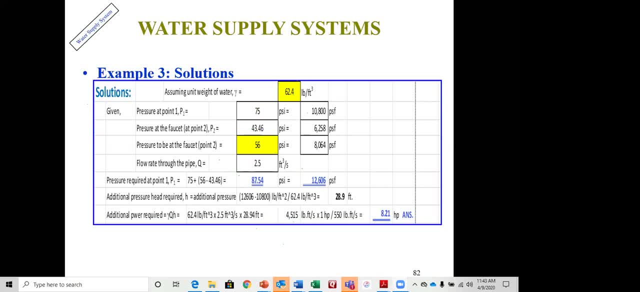 that means gamma into p, gamma okay, gamma p equal to the uh, gamma h, so pq. i think sorry it would be pq. so if we know the p pressure is uh like 87.54 psi, then multiplied with q in, then divided by 550, you should get total horsepower. so 87.54 times 2.5, right. 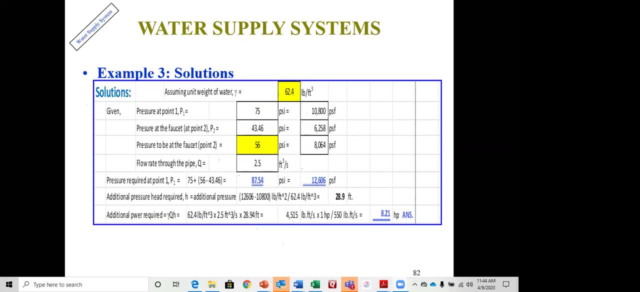 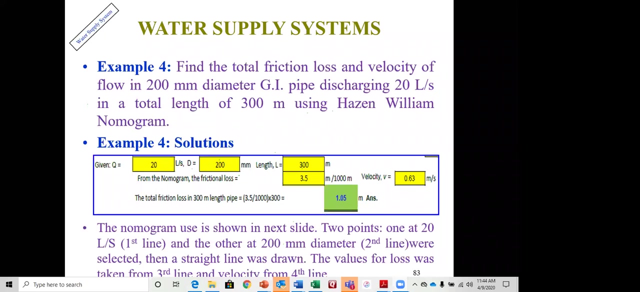 into 144 divided by 62.4 plus 505 times. okay, whatever it comes out to be, all right, okay. so now we'll do one more problem here to uh. see the use of uh as in william nomogram. okay, we used to use it before. nowadays we don't use it because they are different ones. so find 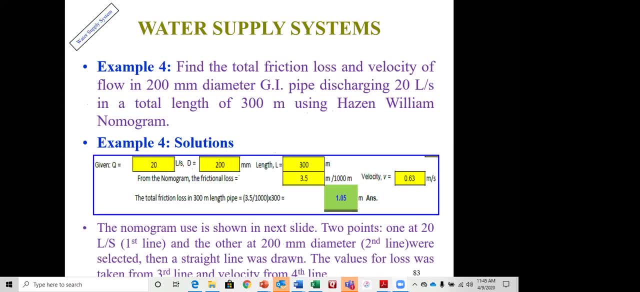 the total friction loss and velocity of flow in 200 millimeter diameter gi pipe, discharging 20 liter per second. 20 liter per second in a total length of 300 meter, using, as in william, homogram. so in this case, given q equal to this, d equal to this, l equal to this, and the friction loss. 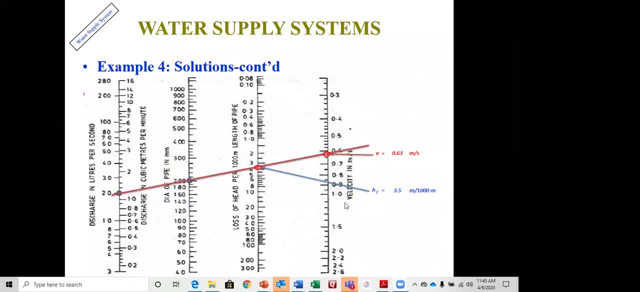 let's use this so i have this data right if i go back here. so that means i had a q equal to two liter per second. then i had a diameter of the pipe 200 millimeter. so i got this two point right. i got this two point: this point and this point. then 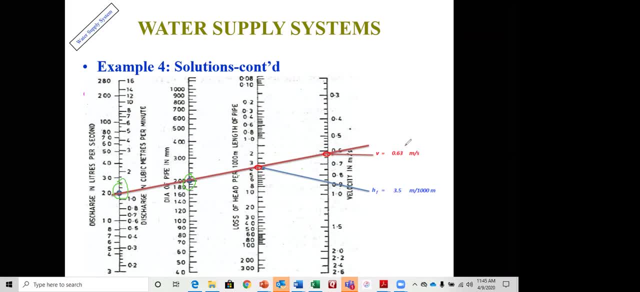 what i did. i had a scale. using the scale, i draw a straight line. then i see it's heated here. right, that means this is almost what: 3.5 meter per 100 meter, 1000 meter, sorry, because it says loss of head length of the pipe. then I used this one here. looks like this is 0.63, so this: 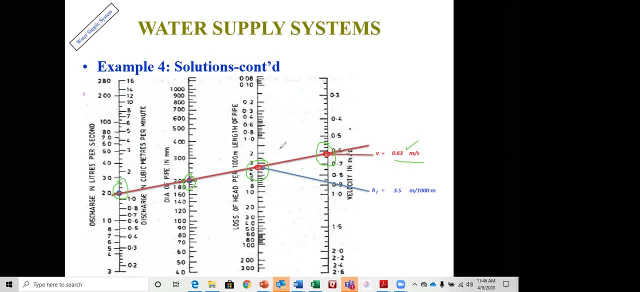 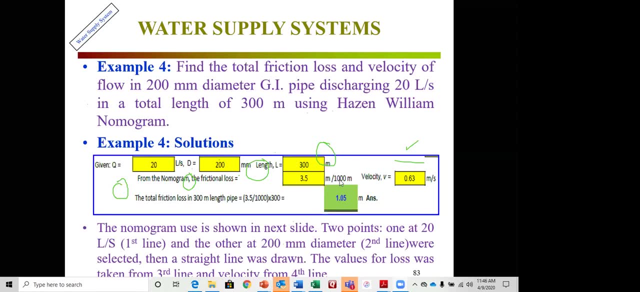 point 63 is a velocity. so then I went back here. okay, I went back here and put the value 3.5 meter per hundred meter, velocity equal to this, and I did the calculation, since it is for thousand meters, since my length of the pipe is: 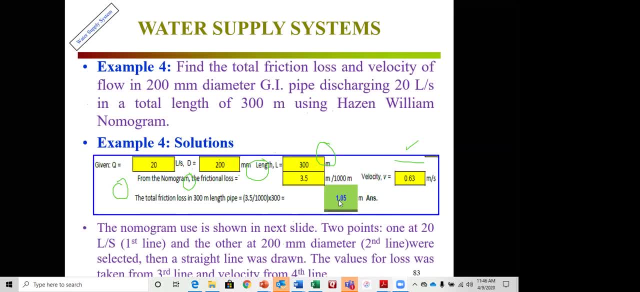 300 meter. I multiplied with 300, I got one point zero five meter. so this is an SI unit. so I get this. now you guys can try another way. so do the same problem like this, problem with the friction loss of 0.01, a friction factor of 0.01, and see: 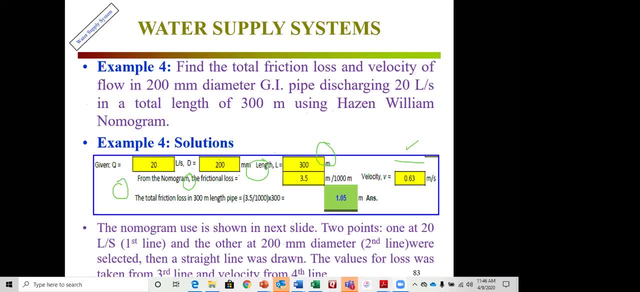 what it comes out to be. we could do probably one solve problem solving to compare like. so which method is good? either Darcy-Weisbach equation or the the Hazen-William Hazen-William is more conservative. it gives you more values, more head loss. 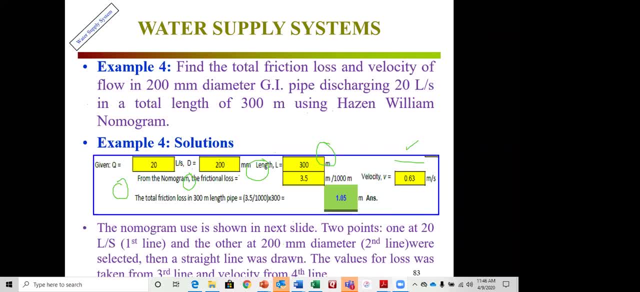 compared to the Darcy-Weisbach equation. I did several calculations on that and that's the one I found. the nomogram is is shown in the next slide. two points, two points: one at 20 liter per second, first line, and two and that means I. 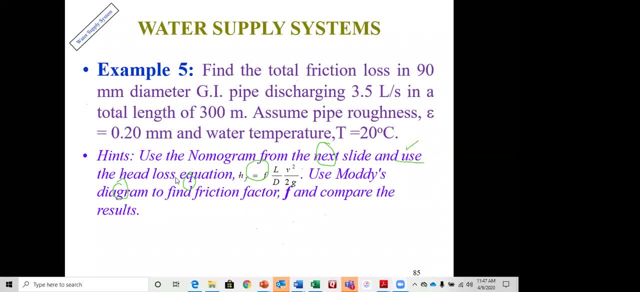 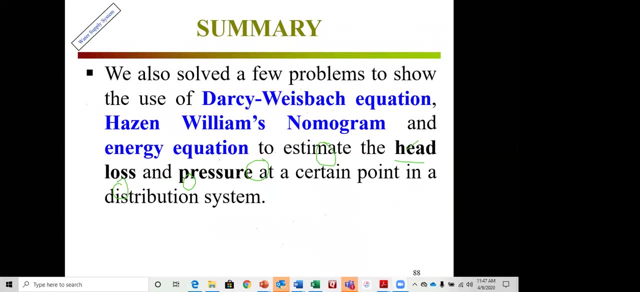 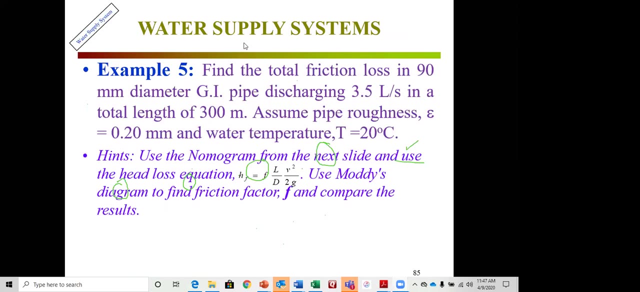 explained whatever I explained over here. okay, you, okay. so it looks like I have another problem here to solve. this could be the last one, looks like. so I think. yeah, I have a comparison here, looks like. okay, so find the total friction loss in 90 millimeter diameter GA pipe discharging. 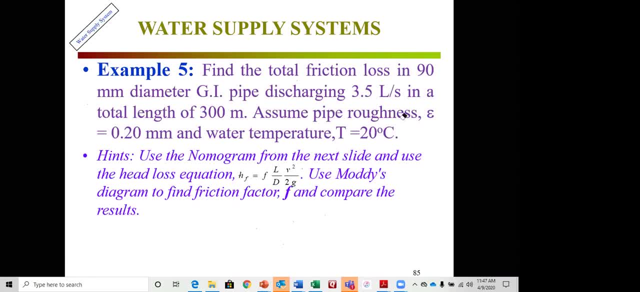 3.5 liters per second in a total length of T and a mutation pipe roughness. if Ceylon is equal to this, and if Ceylon is equal to 3.5 liters per second in a total length of T and a mutation pipe roughness, epsilon is equal to this, and if Ceylon is equal to this and if 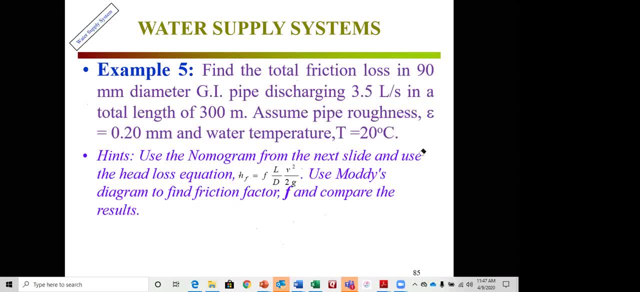 temperature. is this? use the nomogram from the next slide and use the head loss temperature. is this? use the nomogram from the next slide and use the head loss. equation this: you use Moody's diagram to find the factor F and so on. so I think, equation this: you use Moody's diagram to find the factor F and so on. so I think. 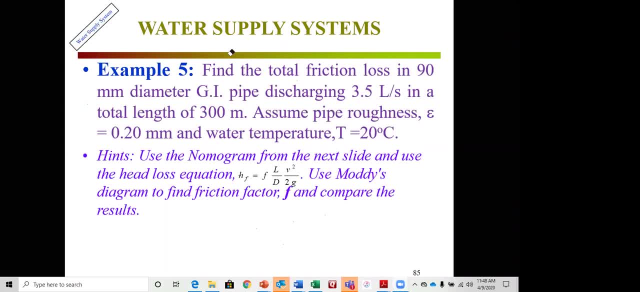 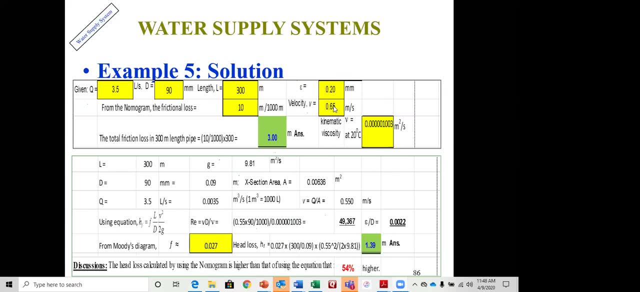 we did it here. see whether I can go back to that. okay. so here is the Q is given. we did it here. see whether I can go back to that. okay. so here is the Q is given. D equal to given this plan. epsilon is given velocity from that one. I use this. D equal to given this plan, epsilon is given velocity from that one. I use this. normal gram looks like. let me see, do I have the normal gram. I think normal gram looks like. let me see, do I have the normal gram. I think normal gram looks like. let me see, do I have the normal gram? I think. 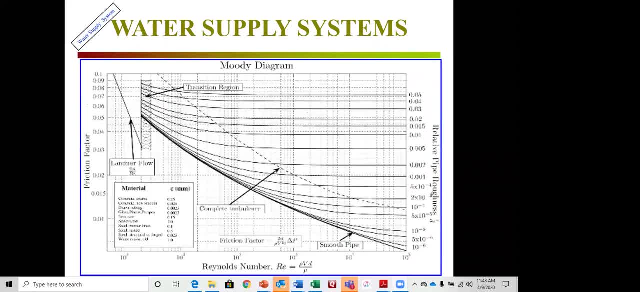 I think I didn't show you here. okay, I didn't. I think I didn't show you here. okay, I didn't. I think I didn't show you here. okay, I didn't show you here how I used it, but show you here how I used it. but. 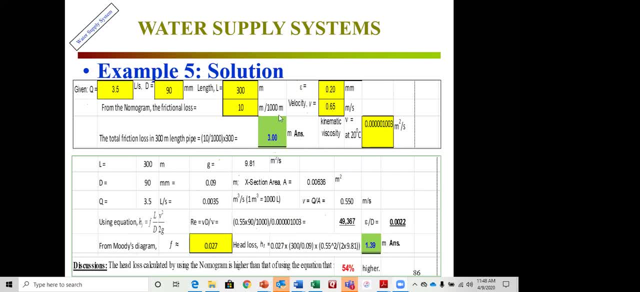 show you here how I used it. but anyway, I got three meter total head loss. anyway. I got three meter total head loss. anyway. I got three meter total head loss and like say: velocity, is this right? if and like say: velocity, is this right? if and like say: velocity, is this right if Ceylon is given now kinetic viscosity, I 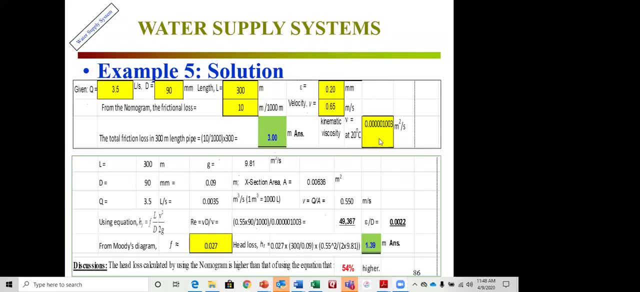 Ceylon is given now kinetic viscosity. I Ceylon is given now kinetic viscosity. I got from the table. because that's what got from the table, because that's what got from the table, because that's what we need, we have to calculate this one for. 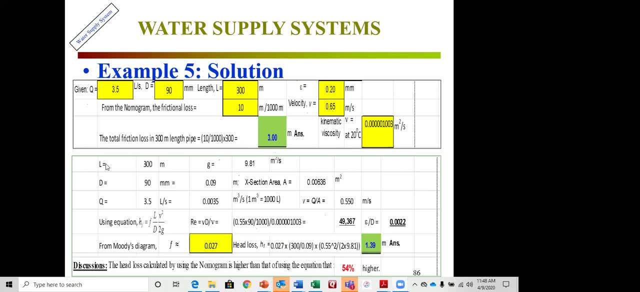 we need. we have to calculate this one for we need. we have to calculate this one for the purpose of HF right for Darcy. the purpose of HF right for Darcy. the purpose of HF right for Darcy. Weisbach equation L equal to 300 meter. 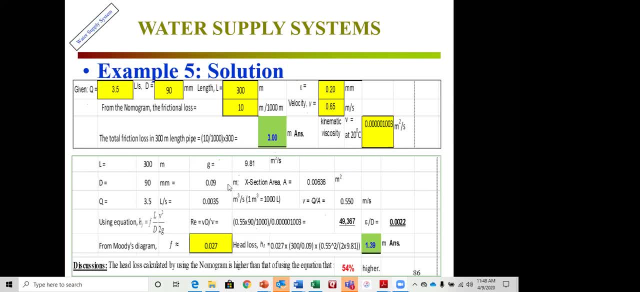 Weisbach equation L equal to 300 meter. Weisbach equation L equal to 300 meter D equal to 90 millimeter means 0.09 meter. D equal to 90 millimeter means 0.09 meter. D equal to 90 millimeter means 0.09 meter a. Q equal to 3.5 liter per second. 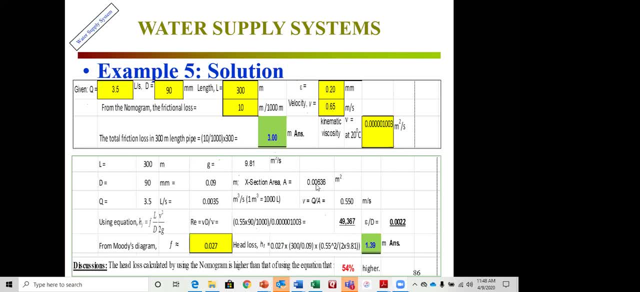 a Q equal to 3.5 liter per second. a Q equal to 3.5 liter per second means 0, 0, 3, 5 meter cube per second. okay, means 0, 0, 3, 5 meter cube per second. okay, means 0, 0, 3, 5 meter cube per second. okay, then, cross-sectional area. we found the 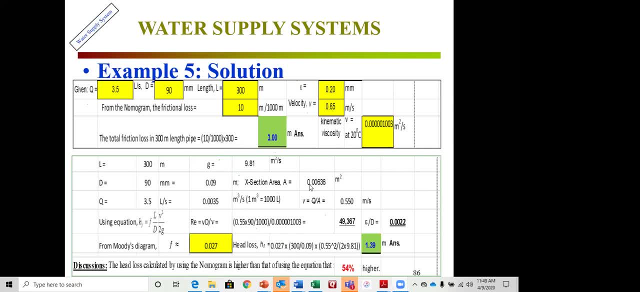 then cross-sectional area. we found the then cross-sectional area. we found the cross-sectional area G equal to 9.81. cross-sectional area. G equal to 9.81. cross-sectional area. G equal to 9.81. cross-sectional area is point 0, 0, 6, 3, 5. 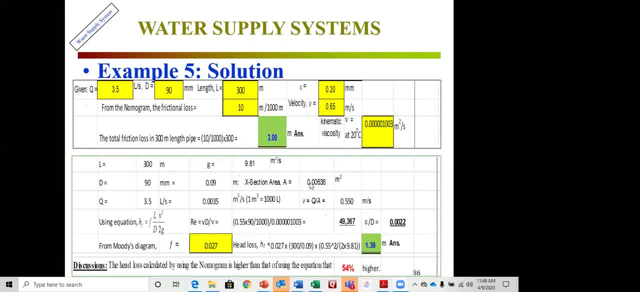 cross-sectional area is point 0, 0, 6, 3, 5. cross-sectional area is point 0, 0, 6, 3, 5. because we know the diameter right this, because we know the diameter right this, because we know the diameter right, this is my diameter, so I calculated this and 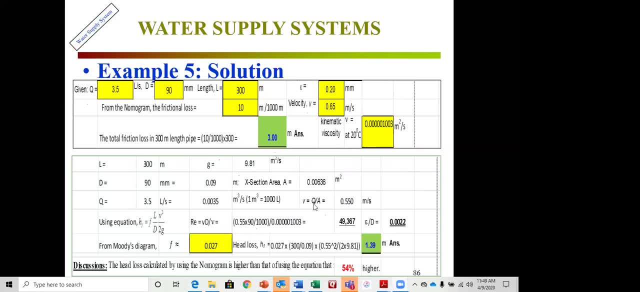 is my diameter, so I calculated this. and is my diameter, so I calculated this. and Q equal to this and B equal to Q over Q equal to this, and B equal to Q over Q equal to this and B equal to Q over A. so Q is given, Q is point 0. 9 area is: 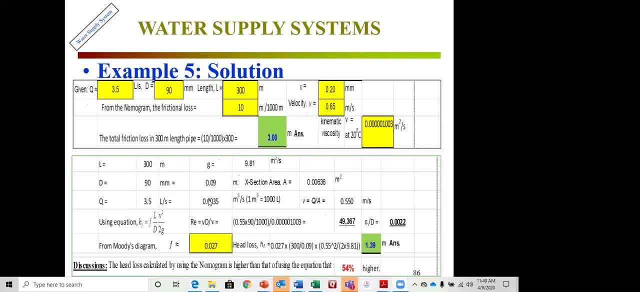 A, so Q is given. Q is point 0, 9 area is A, so Q is given. Q is point 0, 9 area is sorry. Q is like point 0, 0, 3, 5 area is sorry. Q is like point 0, 0, 3, 5 area is. 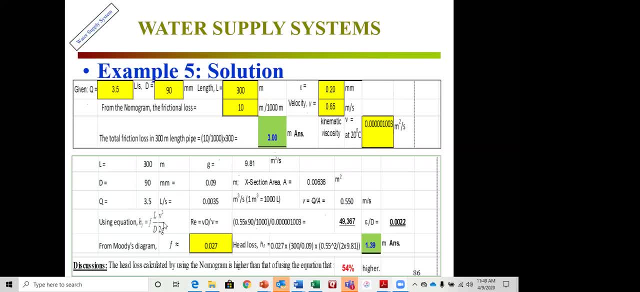 sorry, Q is like point 0, 0, 3, 5 area is this: if I do that, I get a velocity of 0.5. this: if I do that, I get a velocity of 0.5. this: if I do that, I get a velocity of 0.5, 5 meter per second. now using HF, equal. 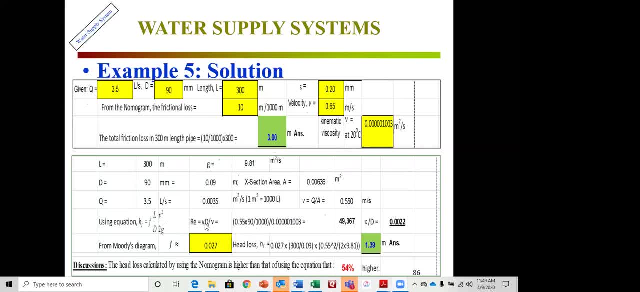 5 meter per second now using HF. equal 5 meter per second now using HF. equal to this. we have to calculate something to this. we have to calculate something to this. we have to calculate something else. this coronal's number, a video over. else, this coronal's number, a video over. 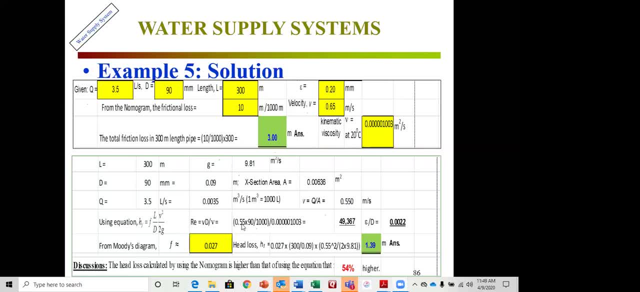 else this coronal's number. a video over new, so new. that's the reason I get the new so new. that's the reason I get the new so new. that's the reason I get the new here. so V D over new. so I got 49. 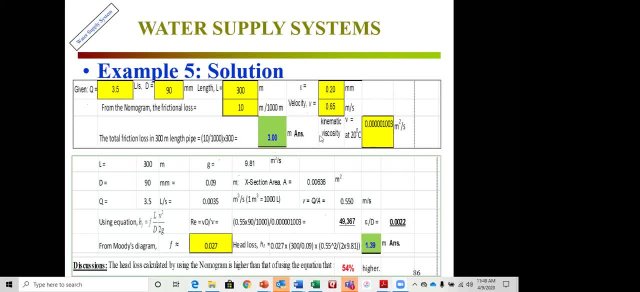 new here, so V D over new. so I got 49 new here, so V D over new. so I got 49 366 epsilon by D equal to this epsilon: 366. epsilon by D equal to this epsilon: 366. epsilon by D equal to this epsilon is given here. D is also given here, so I 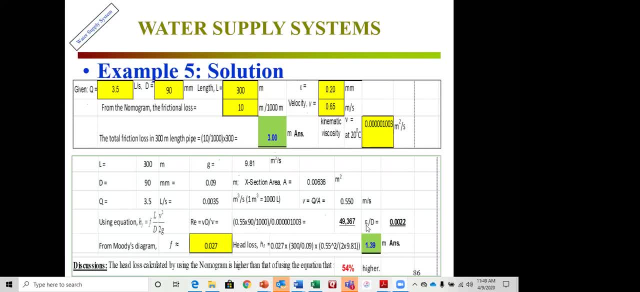 is given here. D is also given here, so I is given here. D is also given here, so I got this. if it is in millimeter, then D got this. if it is in millimeter, then D got this. if it is in millimeter, then D have to be millimeter, so I get point 0: 0. 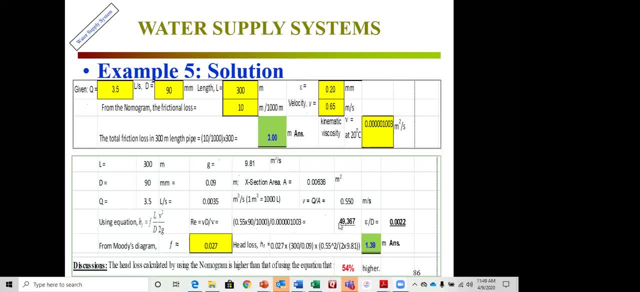 have to be millimeter, so I get point 0. 0 have to be millimeter, so I get point 0. 0. 2. 2 now we can go back to: I have 49,000. 2- now we can go back to: I have 49,000. 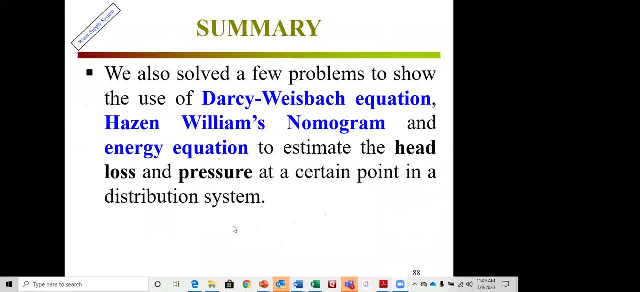 2 now we can go back to. I have 49,000, and here it is a point 0, 0, 2, 2. so if I, and here it is a point 0, 0, 2, 2. so if I- and here it is a point 0, 0, 2, 2. so if I go to a husband- William, sorry this- 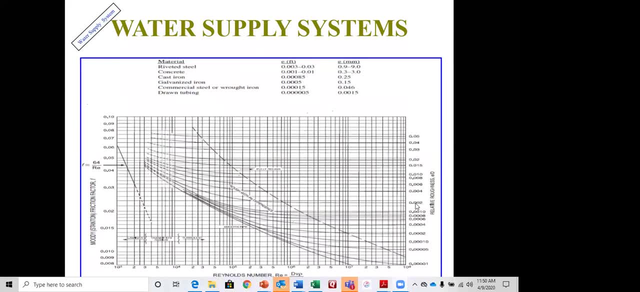 go to a husband, William. sorry this. go to a husband, William. sorry this diagram. let's see: have better 1.0 2 2 diagram. let's see: have better 1.0 2 2 diagram. let's see: have better 1.0 2 2 right or 0 0 0 2 2, I think it's 0 0 2. 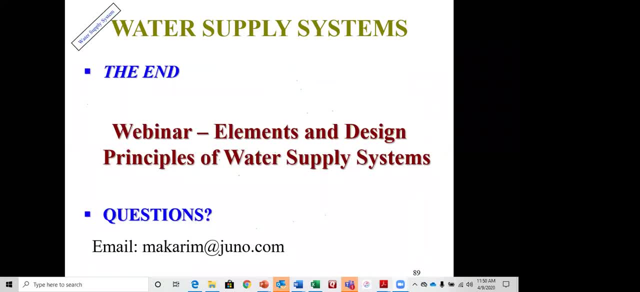 right, or 0 0 0 2 2? I think it's 0 0 2 2 right, or 0 0 0 2 2? I think it's 0 0 2 2, you can remember 0 0 2, 2 and 49,000. 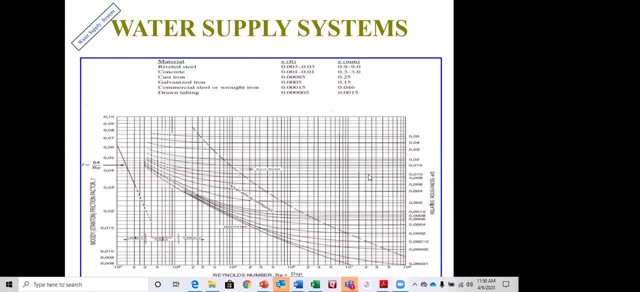 you can remember 0 0, 2, 2 and 49,000. you can remember 0 0, 2, 2 and 49,000. right 0 0 2, 2, so it will be somewhere. right 0 0, 2, 2, so it will be somewhere. 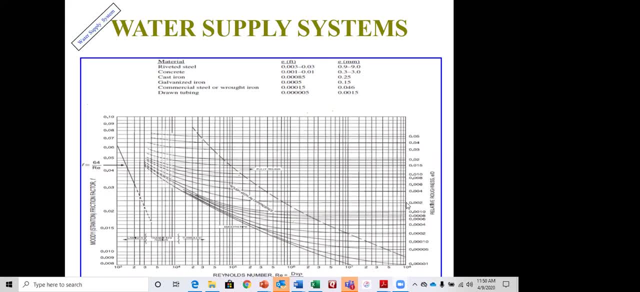 right: 0, 0, 2, 2, so it will be somewhere around here, somewhere around here and around here, somewhere around here and around here, somewhere around here. and the. the other one is 49,000, so this is the. the other one is 49,000, so this is. 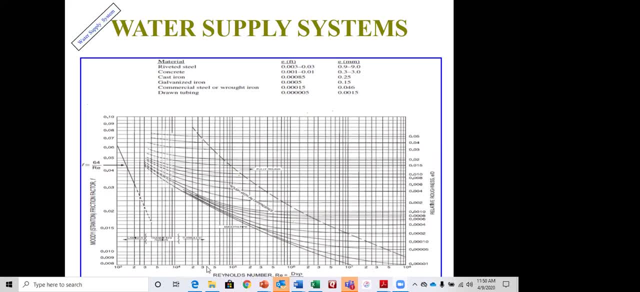 the. the other one is 49,000. so this is 10,000, right? this is 10,000 20,000. 10,000, right. this is 10,000, 20,000. 10,000, right. this is 10,000, 20,000, 30,000, 40, 50, so 49,000 would be. 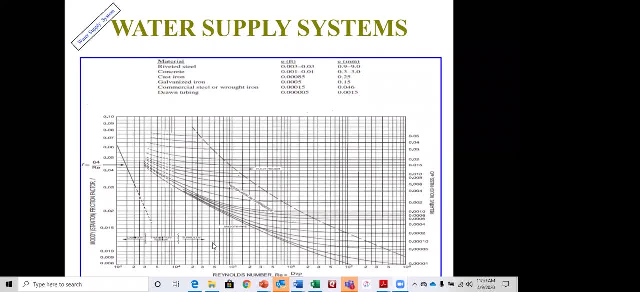 30,000- 40- 50, so 49,000 would be. 30,000: 40- 50, so 49,000 would be somewhere around here. if I go this way, somewhere around here, if I go this way, somewhere around here, if I go this way, so if I go this way and I come up with 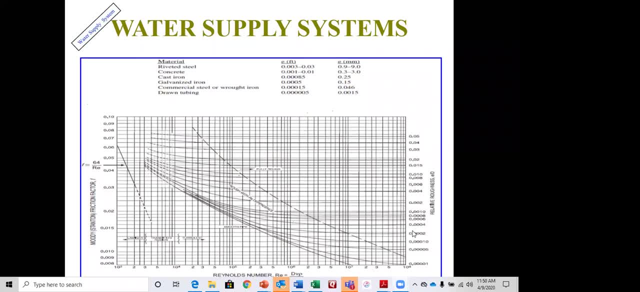 so if I go this way and I come up with, so if I go this way and I come up with something like this, okay, so that mean something like this. okay, so that mean something like this. okay, so that mean this line may go this way. okay, this way. 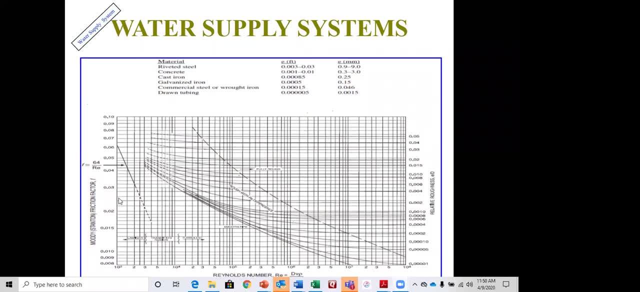 this line may go this way, okay, this way, so that means in here somewhere. then if so, that means in here somewhere. then if so that means in here somewhere, then if I go back here, I get point zero to five. I go back here, I get point zero to five. 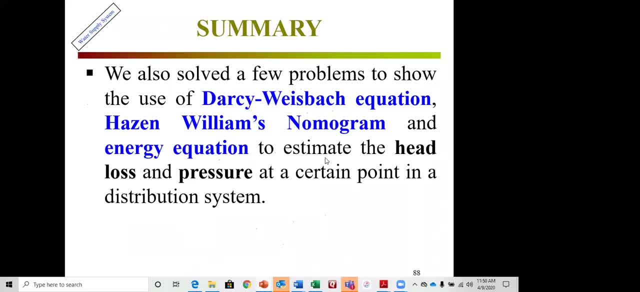 I go back here, I get point zero to five: maybe so F value. let's see what I have. maybe so F value. let's see what I have maybe so F value. let's see what I have in here. how I calculate it. so I got one in here. how I calculate it. so I got one. 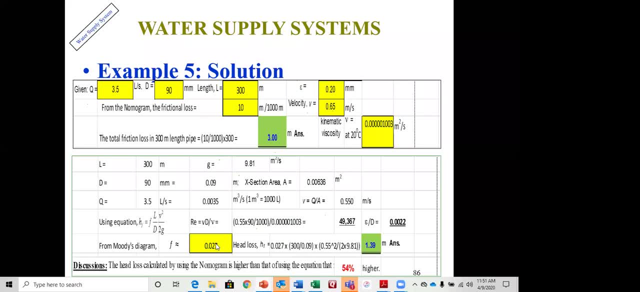 in here how I calculate it. so I got one zero to seven. okay, I probably I said zero to seven. okay, I probably I said zero to seven. okay, I probably I said because this is more accurate. so now because this is more accurate, so now because this is more accurate. so now head loss is going to put F equal to 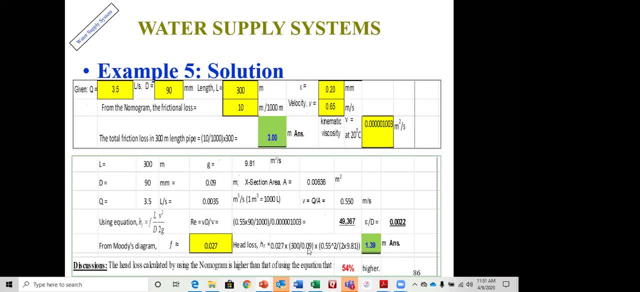 head loss. is going to put F equal to head loss. is going to put F equal to point zero to seven, then 300 divided by point zero to seven, then 300 divided by point zero to seven, then 300 divided by this, L, L is 300 meter, D is basically D. 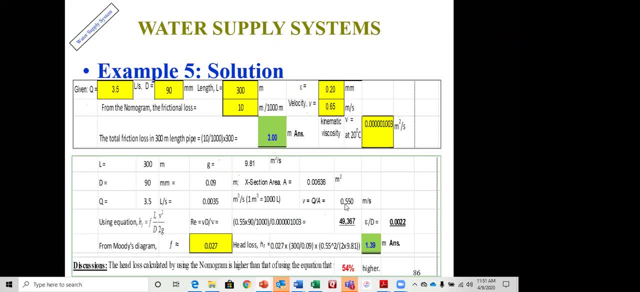 this L? L is 300 meter. D is basically D. this L? L is 300 meter. D is basically: D is 0.09 and V is equal to this. V. squared is 0.09 and V is equal to this. V. squared is 0.09 and V is equal to this V squared by 2 G. G equal to nine point eight one. 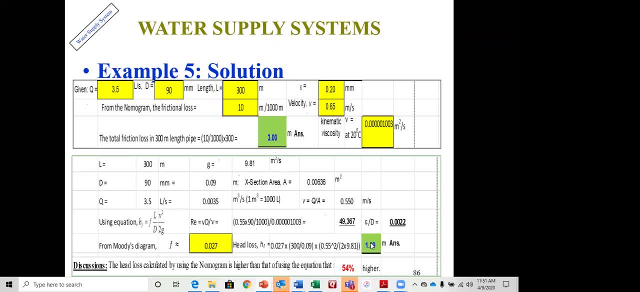 by 2 G G equal to nine point eight. one by 2 G G equal to nine point eight one. here I get one point three nine. so you, here I get one point three nine. so you, here I get one point three nine. so you see, this one looks like this is by: 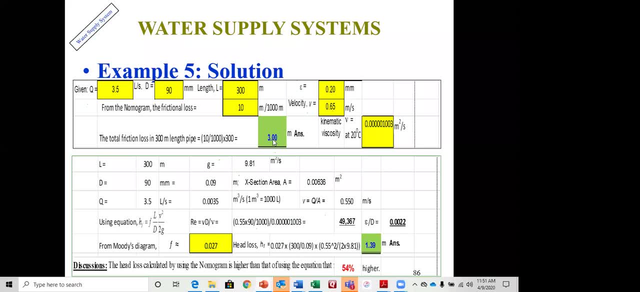 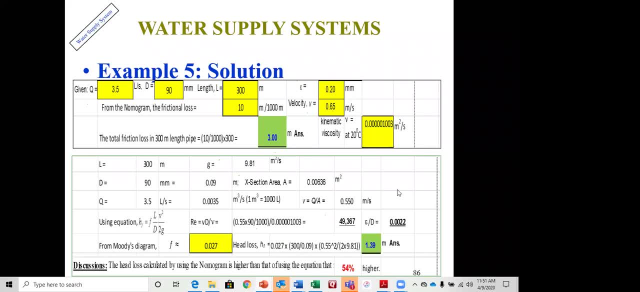 Darcy-Weisbach equation. and this is by: as in William diagram 3 and 1.49, the. as in William diagram 3 and 1.49, the. as in William diagram 3 and 1.49. the difference is almost 54 percent here it. 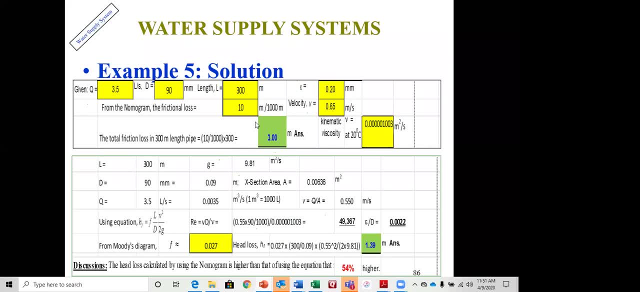 difference is almost 54 percent. here it difference is almost 54 percent. here it is 44 percent higher. okay, here it is is 44 percent higher. okay, here it is is 44 percent higher. okay, here it is. more conservative calculation- more wrong. more conservative calculation, more wrong. 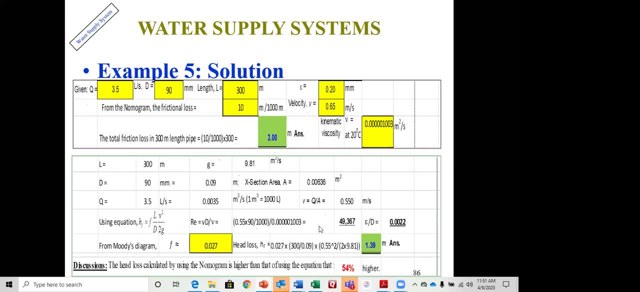 more conservative calculation, more wrong right in the sense of being wrong, so right in the sense of being wrong, so right in the sense of being wrong. so that's another way to understand the two. that's another way to understand the two. that's another way to understand the two. problem I mean, which one is more? 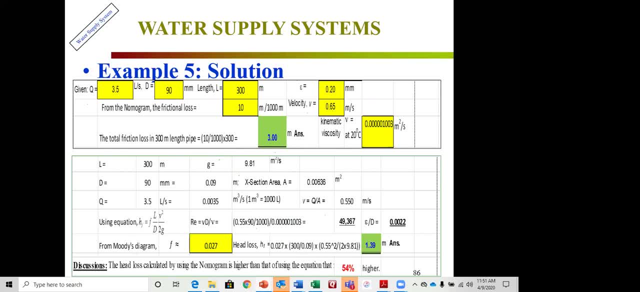 problem. I mean, which one is more important in this case, and and so on. important in this case, and and so on. important in this case, and and so on. okay, the summary of the code, this course. okay, the summary of the code, this course. okay, the summary of the code, this course. we define and elaborated on water cycle. 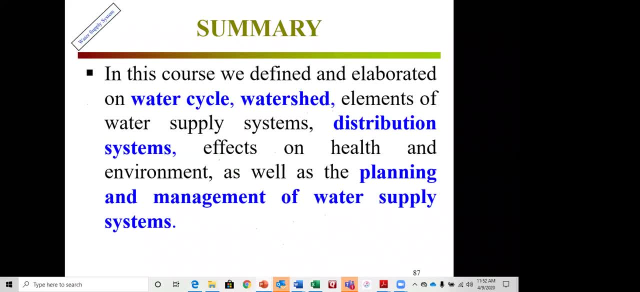 we define and elaborated on water cycle. we define and elaborated on water cycle. watershed elements of water supply. watershed elements of water supply. watershed elements of water supply system distribution system. effect on system distribution system. effect on system distribution system. effect on health and environment, as well as the. 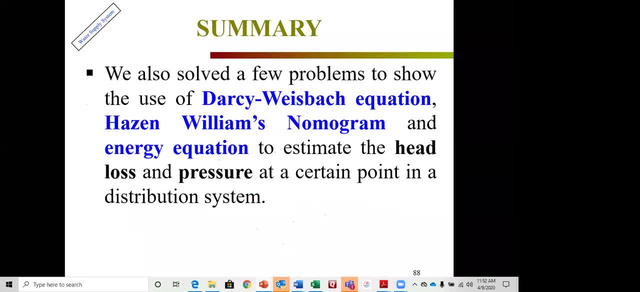 health and environment, as well as the health and environment, as well as the planning and management of water supply: planning and management of water supply, planning and management of water supply system. we also solve a few problems to system. we also solve a few problems to system. we also solve a few problems to show the use of Darcy-Weisbach equation. 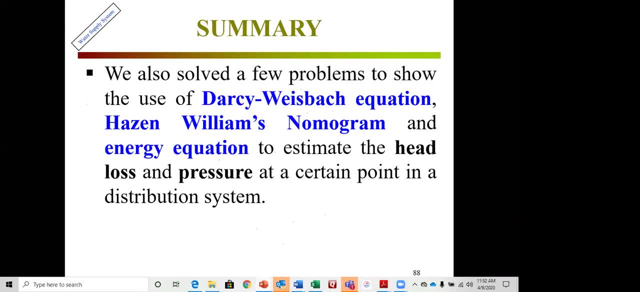 show the use of Darcy-Weisbach equation. show the use of Darcy-Weisbach equation. Hazel Williams tomogram and energy. Hazel Williams tomogram and energy. Hazel Williams tomogram and energy equation to estimate the head loss. and equation to estimate the head loss and. 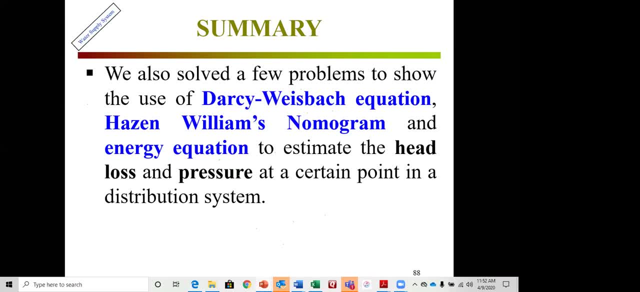 equation to estimate the head loss and pressure at the certain point in pressure, at the certain point in pressure, at the certain point in distribution system. so that's it for distribution system. so that's it for distribution system. so that's it for that, and I think this is the diagram you 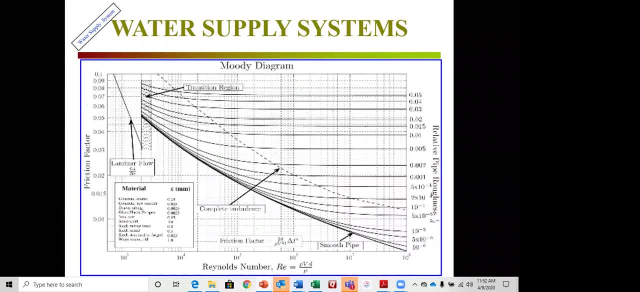 that and I think this is the diagram. you that and I think this is the diagram. you can use it if you want to. this is can use it if you want to. this is can use it if you want to. this is Moody's diagram. this Reynolds number. 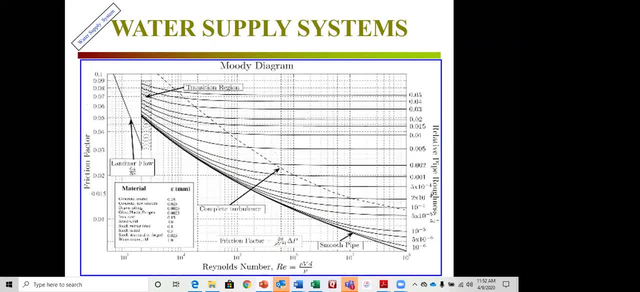 Moody's diagram, this Reynolds number, Moody's diagram, this Reynolds number. this is the friction factor and this is this is the friction factor and this is this is the friction factor and this is the relative pipe roughness external. the relative pipe roughness external, the relative pipe roughness external over D and anything's like that, I think. 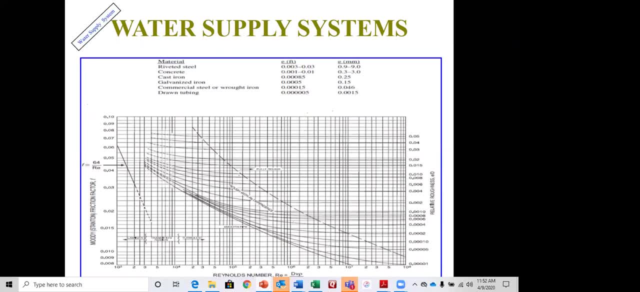 over D and anything's like that. I think over D and anything's like that, I think the last one is the better one. yeah, okay, the last one is the better one. yeah, okay, the last one is the better one. yeah, okay. now I'm opening it for the question and. 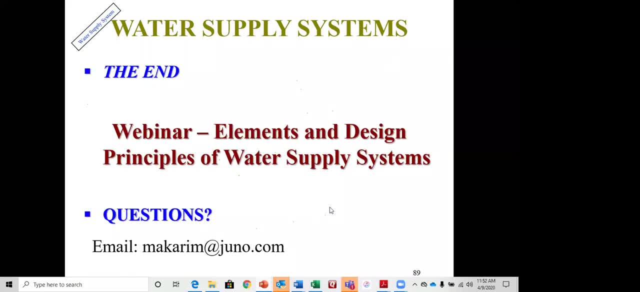 now I'm opening it for the question and now I'm opening it for the question and answer. so okay, it looks like there may answer. so okay, it looks like there may answer. so okay, it looks like there may be some question or no. okay, so yeah, I. 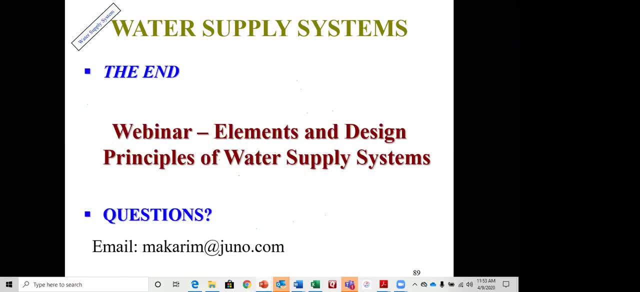 be some question or no, okay? so yeah, I be some question or no, okay? so yeah, I think it's from PDH source. please take. think it's from PDH source, please take. think it's from PDH source. please take the keys. you've said you do the. 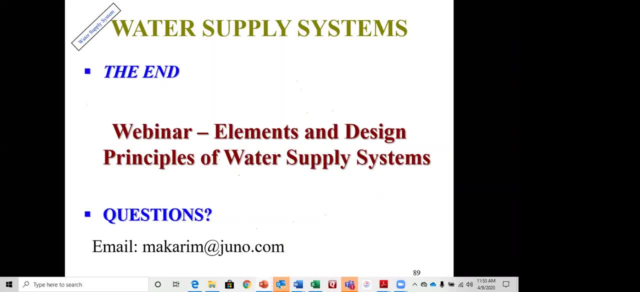 the keys you've said you do the. the keys you've said you do the completion will be okay. we have seven- completion will be okay. we have seven- completion will be okay. we have seven more minutes. we can hang around and ask more minutes. we can hang around and ask. 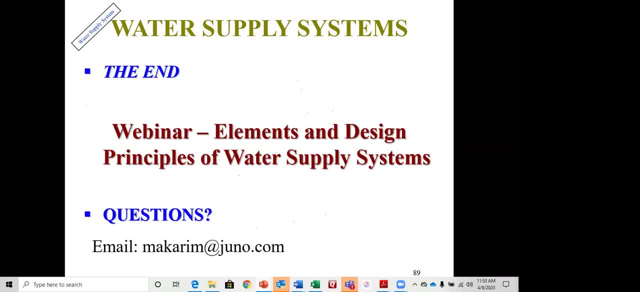 more minutes. we can hang around and ask any questions, or can you guys speak up any questions? or can you guys speak up any questions? or can you guys speak up, maybe, maybe, okay, you have to raise your hand to speak. okay, you have to raise your hand to speak. 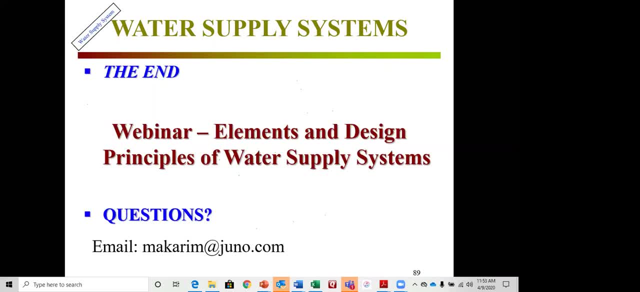 okay, you have to raise your hand to speak up. I can see their hands, or anything. okay, let me see it. even I don't see the. okay, let me see it. even I don't see the. okay, let me see it. even I don't see the list of the participants. they are and I. 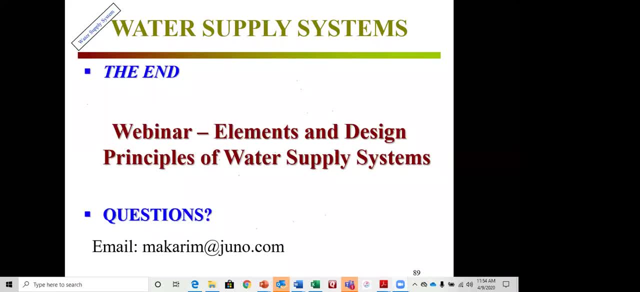 list of the participants they are and I list of the participants they are. and I don't know that anybody raised don't know that anybody raised don't know that anybody raised hands or hands, or hands, or okay guys, thank you, you guys can drop. okay guys, thank you, you guys can drop. 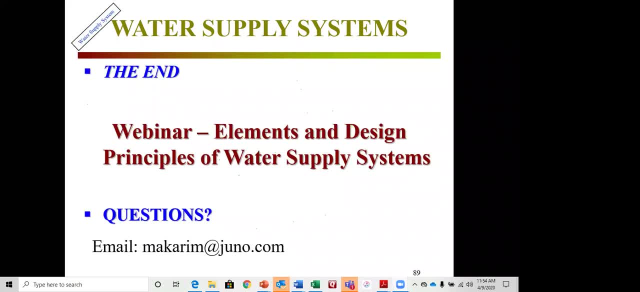 okay guys, thank you, you guys can drop. I'll hang in in few more minutes. if I'll hang in in few more minutes. if I'll hang in in few more minutes if anybody has any questions. anybody has any questions. I'll hang in in few more minutes if anybody has any questions. 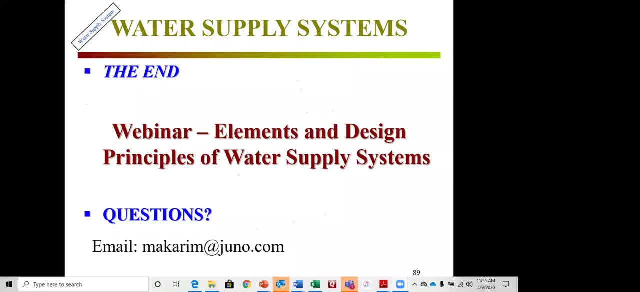 I'll hang in in few more minutes. if anybody has any questions, Okay, Go ahead and speak. if you want to speak, I can hear you. maybe Can you speak, Richard. No, I can't hear you. How do we receive our PDH points?